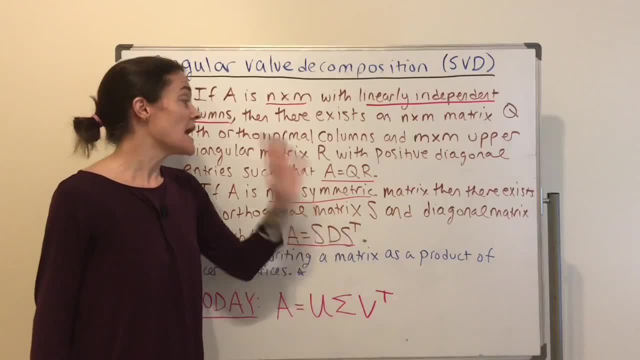 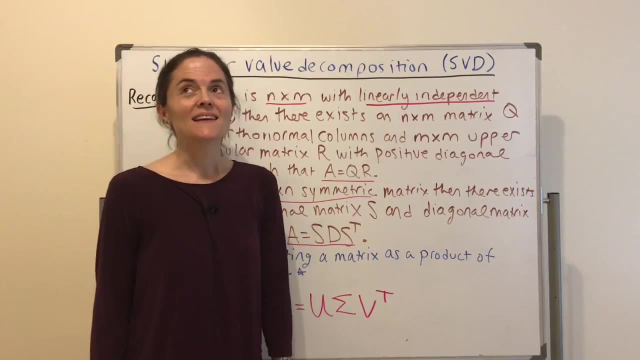 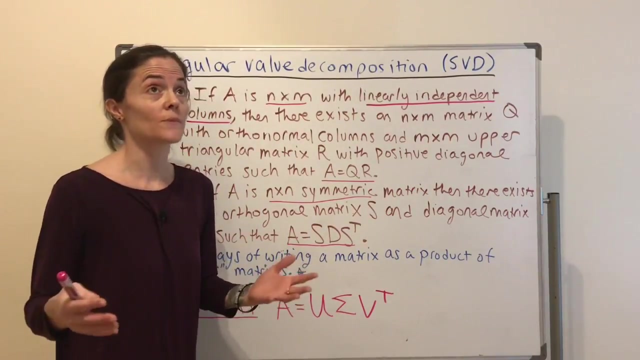 So that means SI. So we have this orthogonal matrix S, So that means SI is n by n and has orthonormal columns and a diagonal matrix d, such that a is sd s transpose, and you can, you can make a similar statement to two, as we know. if you have a general, just say: 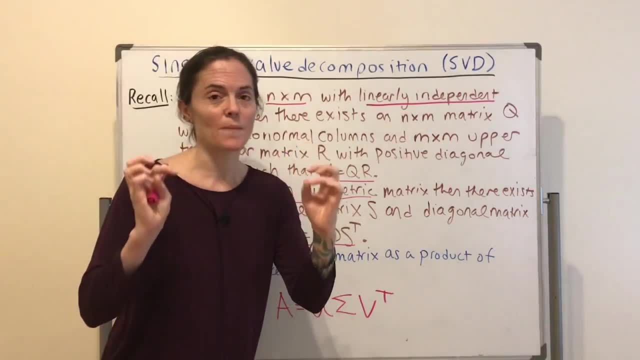 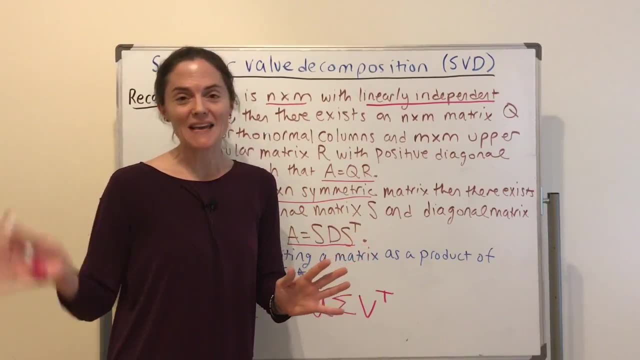 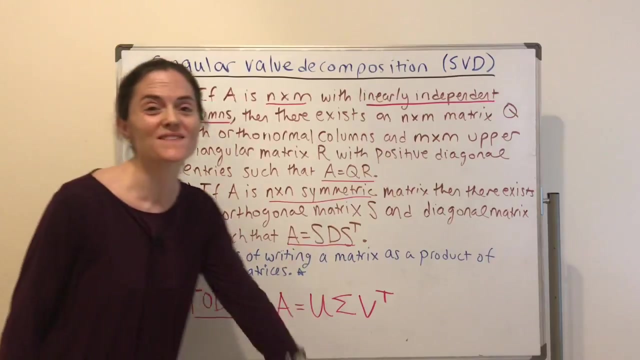 you don't necessarily need symmetric, but you need diagonalizable matrix, and then this would read sd s inverse right. this was what we did when we started doing eigenvalues and eigenvectors, but these are our two main decompositions we have talked about, and both of them are ways of 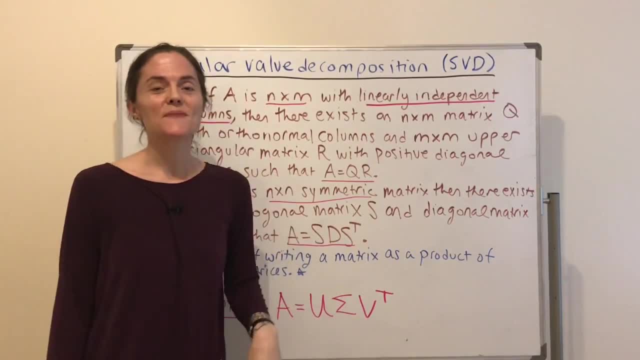 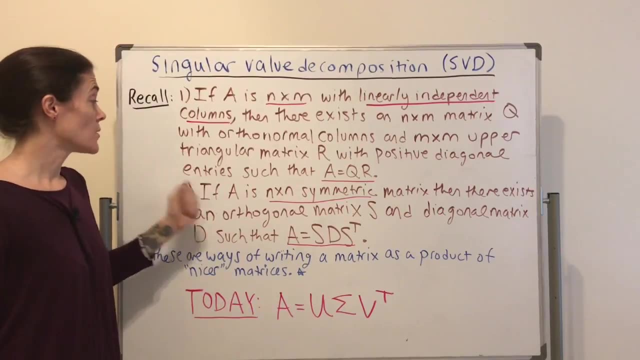 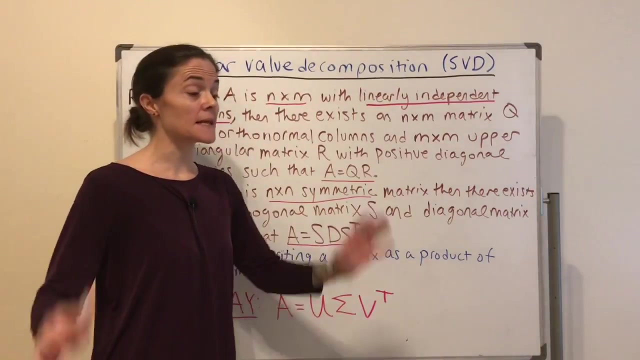 writing a matrix, a as a product of matrices that are that are easier to work with. but we have some hypotheses right here we need symmetric, here we need literally independent columns, and today singular value decomposition is something that constantly occurs in our daily life and we need to remember that singular value decomposition. 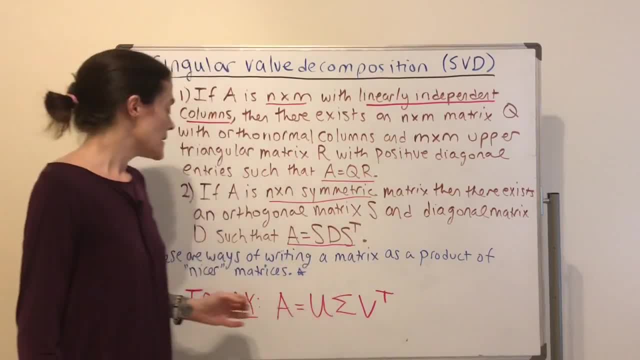 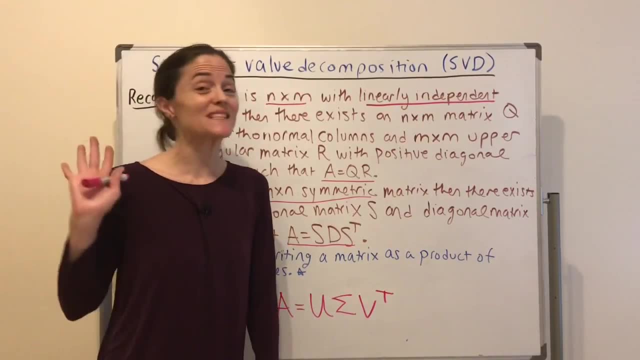 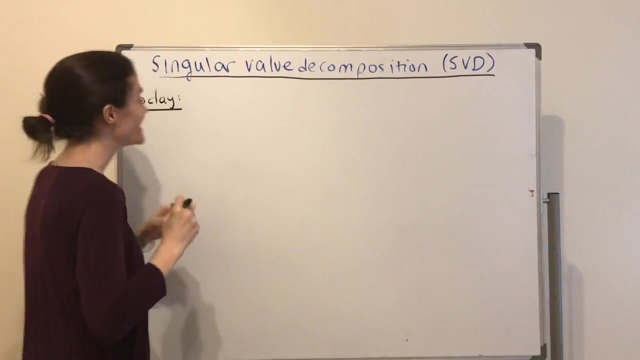 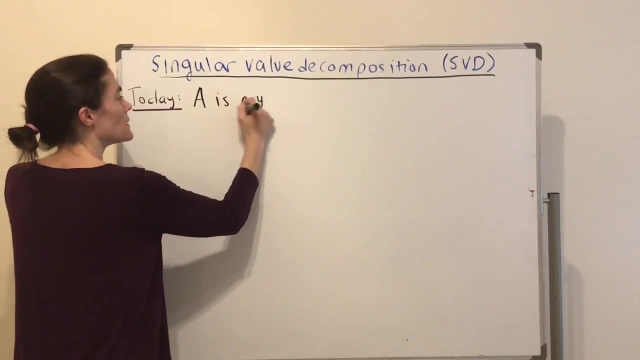 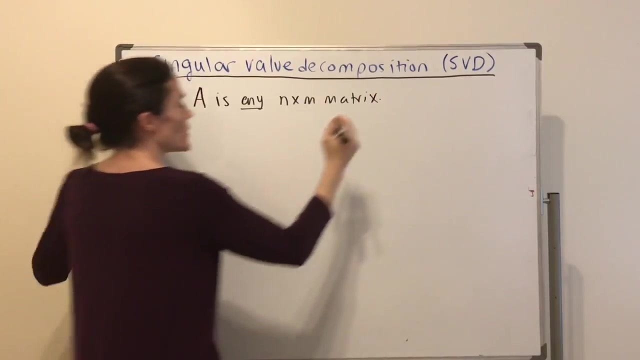 is something that constantly occurs in our daily life and we need to remember that singular value up so much in applications. and we will write a matrix as a product of three matrices, and we can do this for any. and by M matrix: a today, okay. singular value decomposition here: a is any and by M matrix: okay. and then we 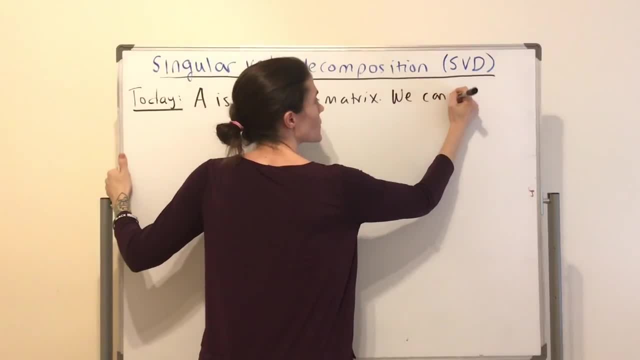 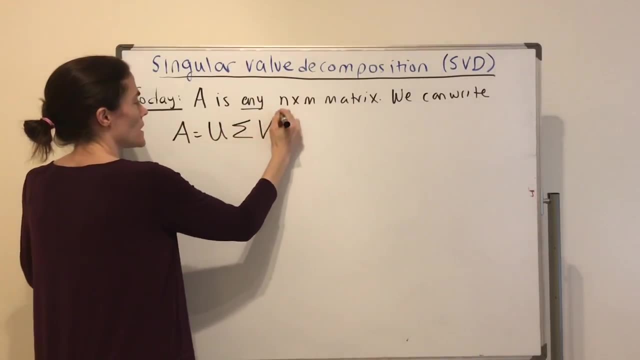 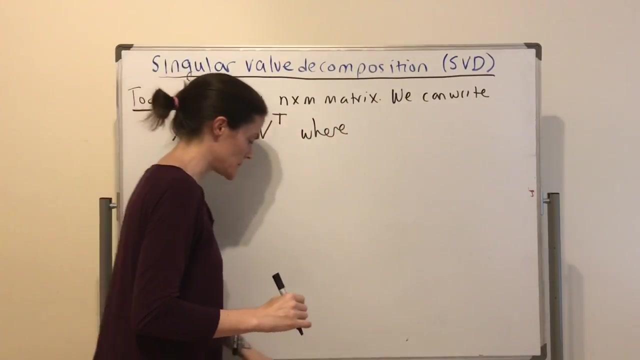 can write a as follows: a is u Sigma V transpose where well, let's think about the size for a matrix. and we can write a as follows: a is u Sigma V transpose where well, let's think about the size for a moment. okay, this is n by M, I'll just a is u Sigma V transpose where well, let's think about the size for. 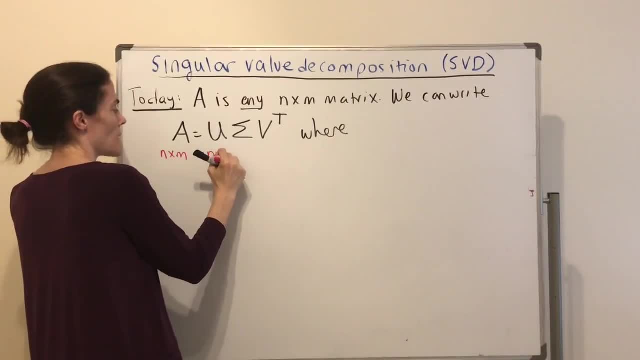 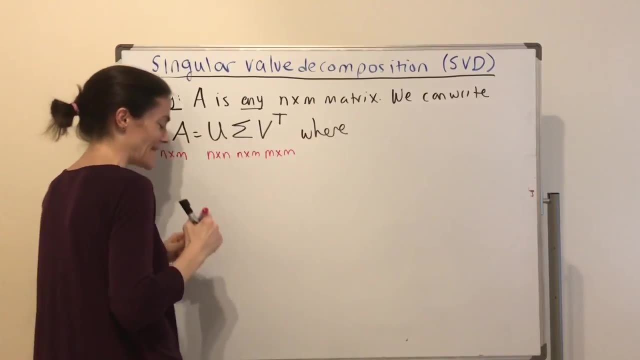 say so. this one needs to be a. n is gonna say so. this one needs to be a. n is gonna be in by n. this one will be M by M and be in by n. this one will be M by M and this one will be n by M. okay, now I can. now, this one will be n by M, and. 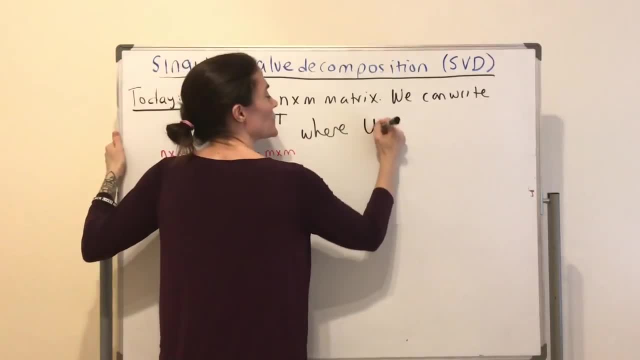 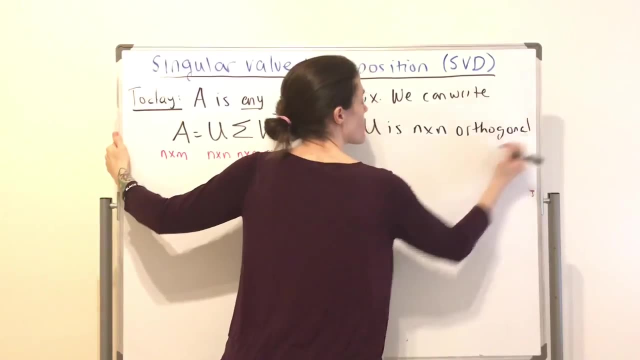 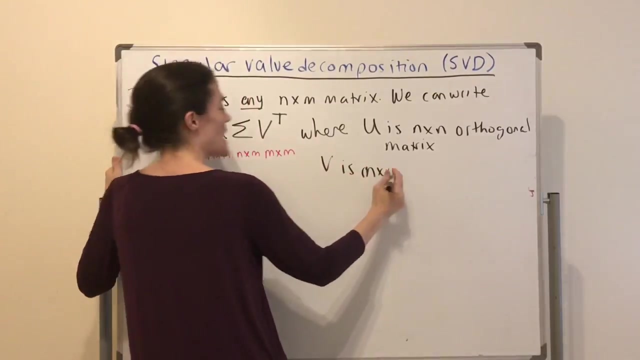 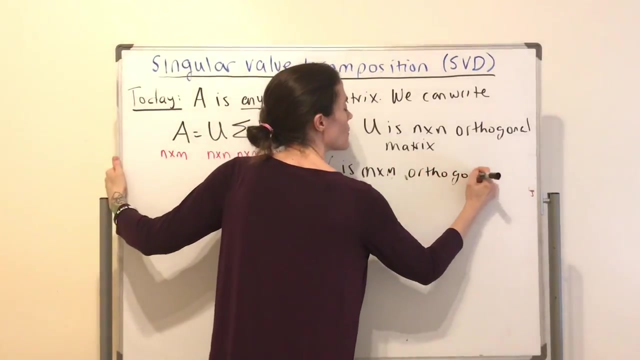 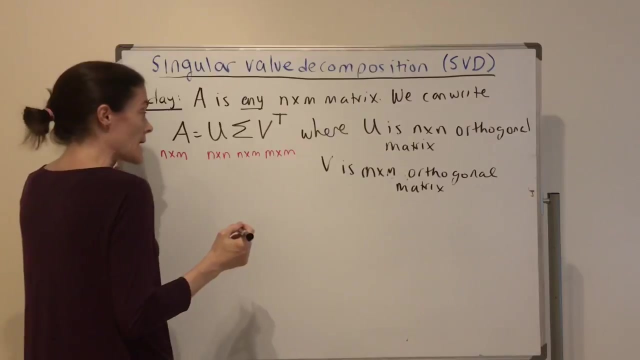 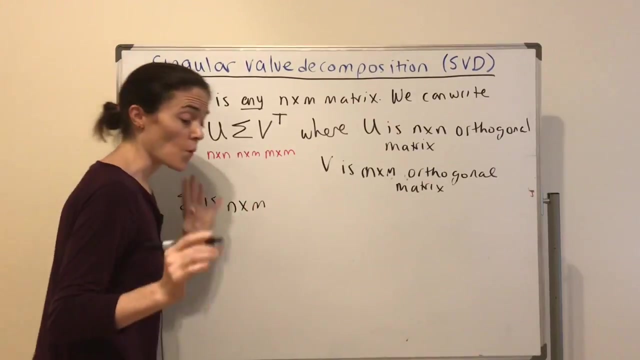 I can explain. so you is n by n- orthogonal. I can explain. so you is n by n- orthogonal matrix, okay, and then V is M by M- orthogonal, okay, and then V is M by M- orthogonal matrix, and Sigma is in by M, where the matrix, and Sigma is in by M where the 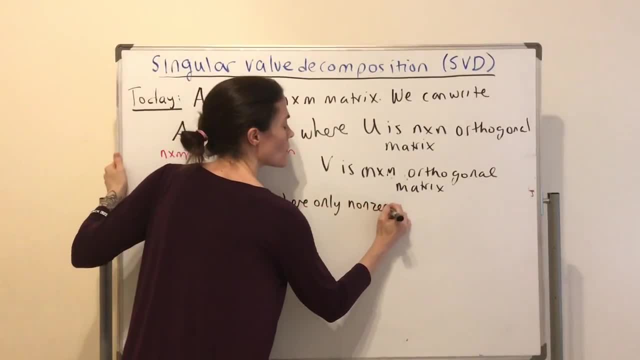 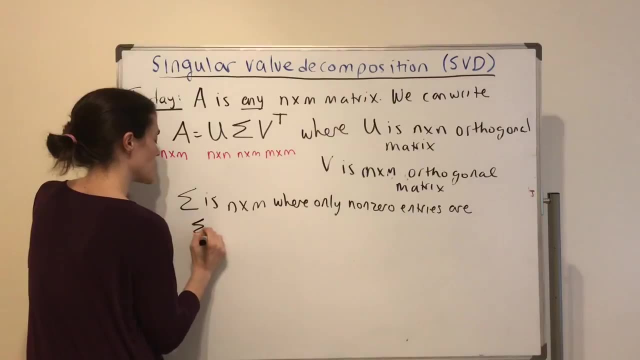 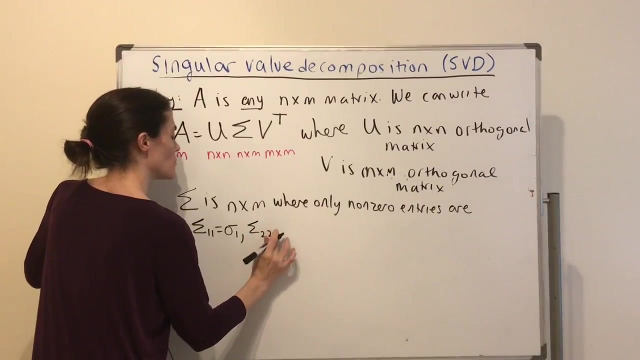 only nonzero entries are, I'll say Sigma only nonzero entries are. I'll say Sigma only nonzero entries are. I'll say Sigma 1, 1, which I'll say is sigma 1, sigma 2, 2, which I'll say is sigma 2, out 2, sigma R, R. 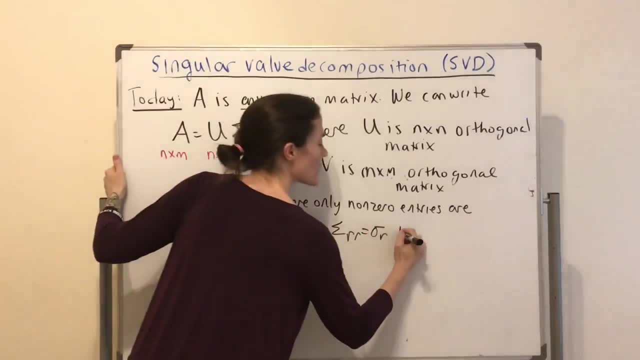 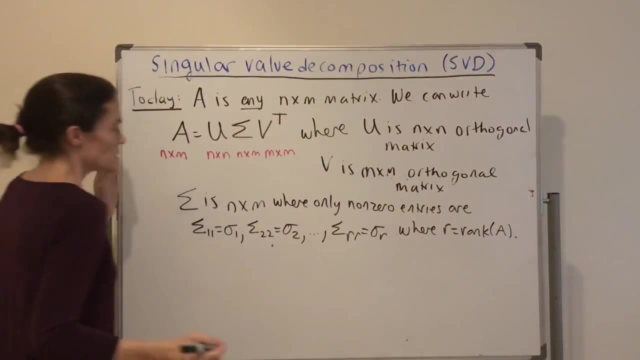 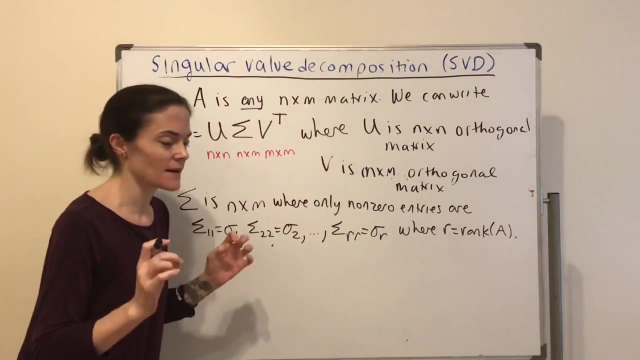 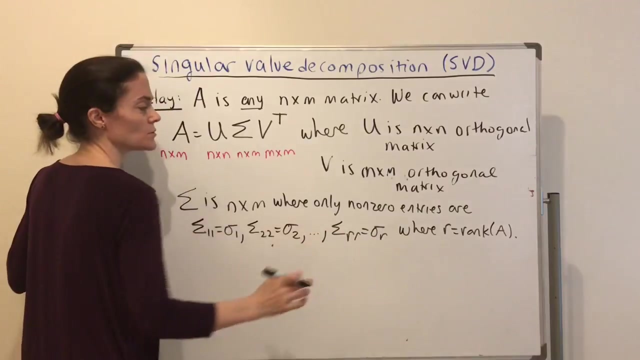 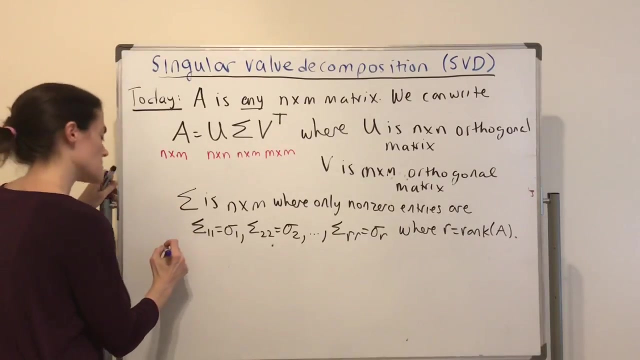 where R is the rank of A. So sigma is not exactly a diagonal matrix, because sigma is generally not square, but the only non-zero entries are along the diagonal and you have them out to the rank of A. okay, And then let's see what else can I say? I'll just mention this comment is: if A is 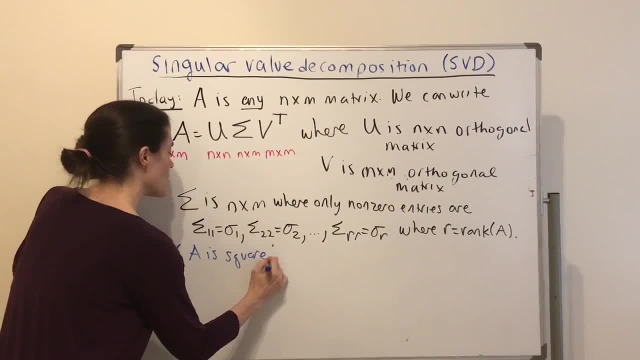 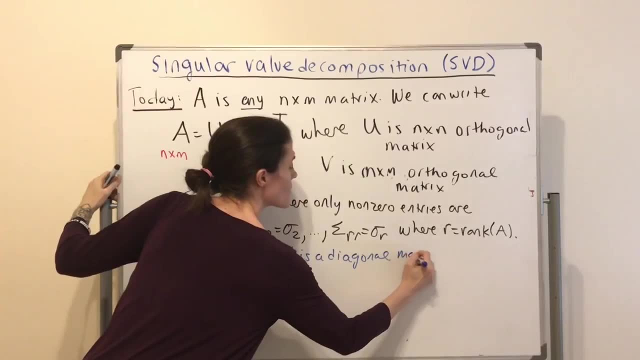 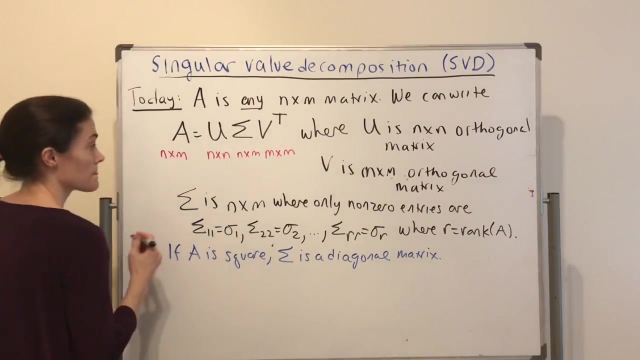 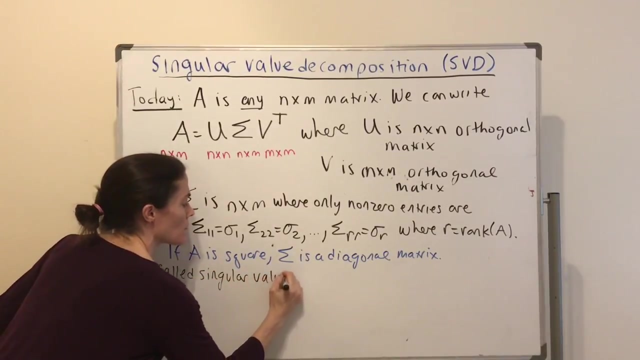 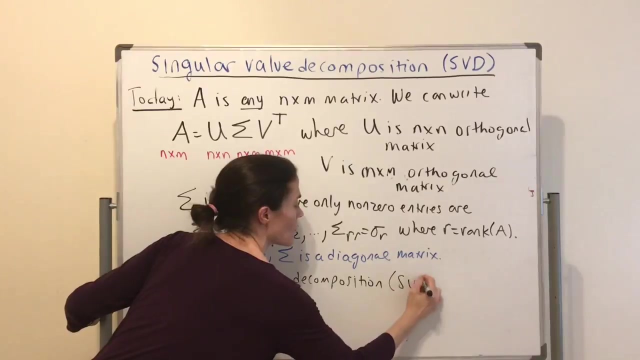 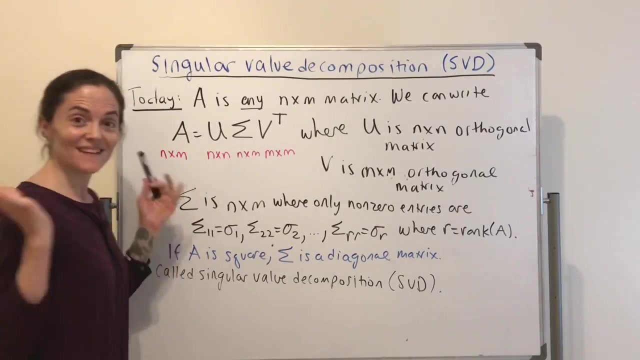 square sigma is a diagonal matrix, and this is called the singular value decomposition. Now there's a lot to discuss here. How do we find sigma? How do we find V? How do we find U Right, that's the whole purpose of today. 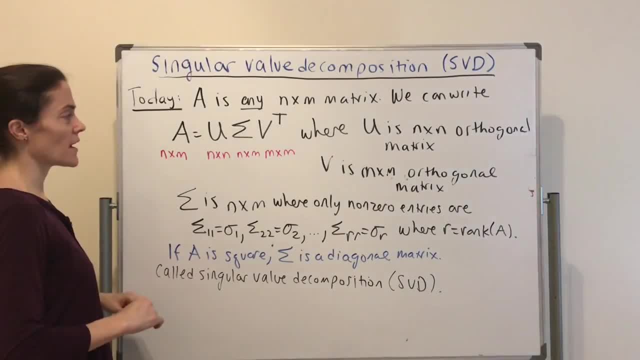 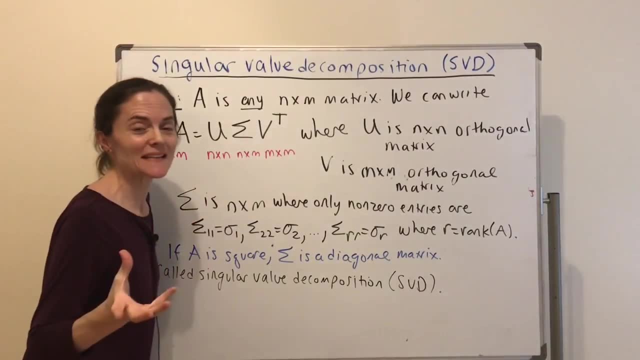 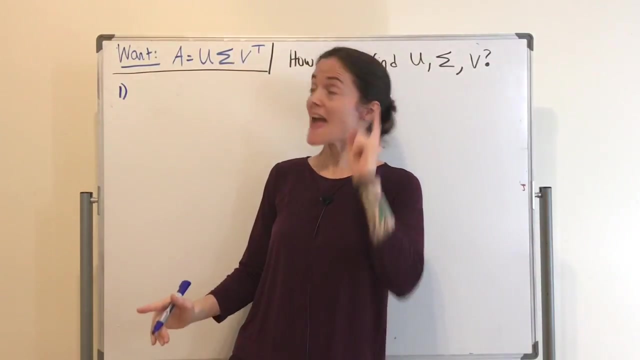 But this is the decomposition we are going for. This is an orthogonal matrix. This is an orthogonal matrix and this is well. you can think of it as being a diagonal, except it's not necessarily a square matrix. Well, this is what we're going for. A is U sigma V transpose. 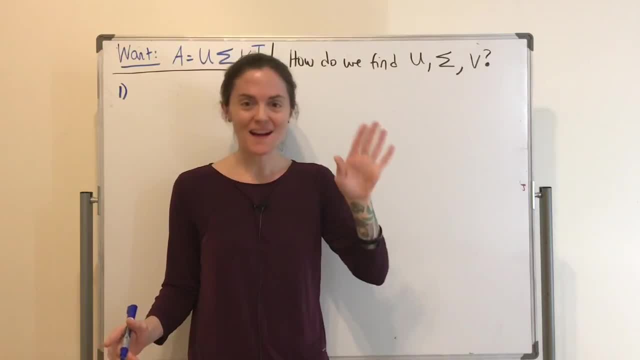 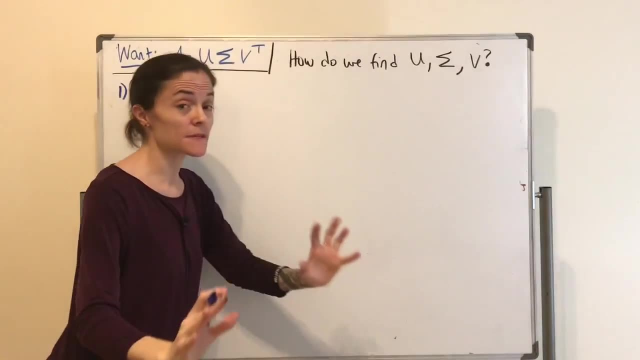 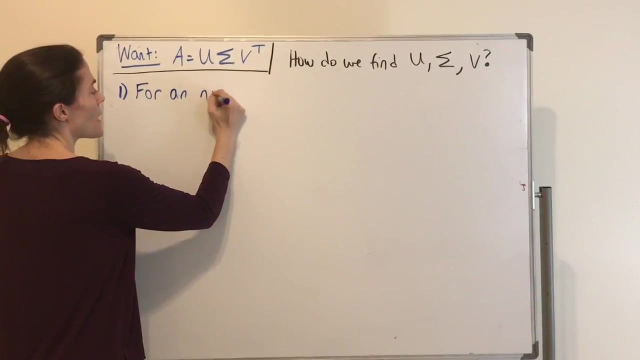 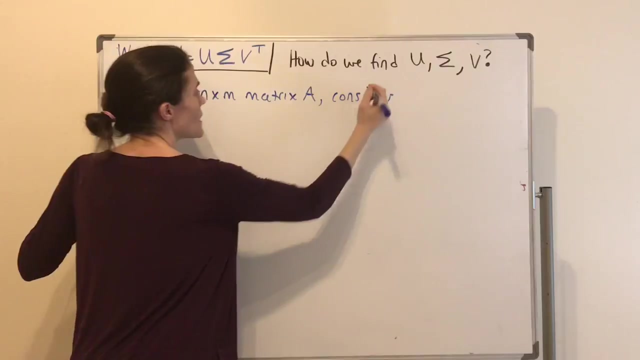 and, just as I said, how are we going to find U, sigma and V? Okay, well, we're going to have to get ourselves there. We're going to have to build some ideas to be able to answer this question. So first, for an N by M, matrix A. let's consider the matrix A. transpose A. 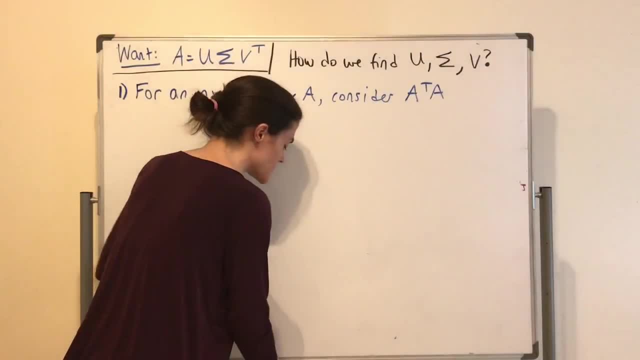 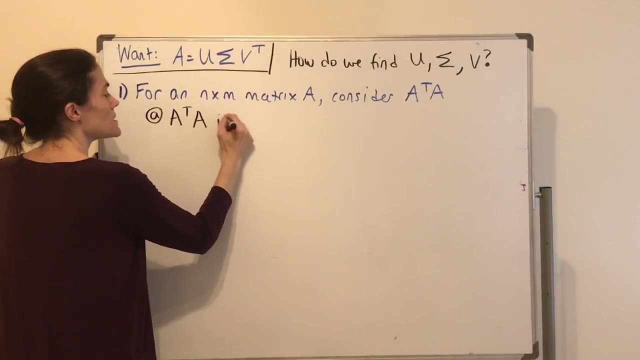 Okay, now I'm going to say a few things about that. The first I will say is the following: A transpose, A is symmetric. And well, what size is it? It's M by M. right, Because A transpose will be M by N. 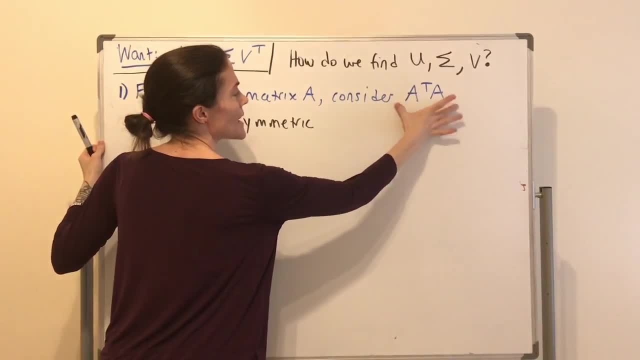 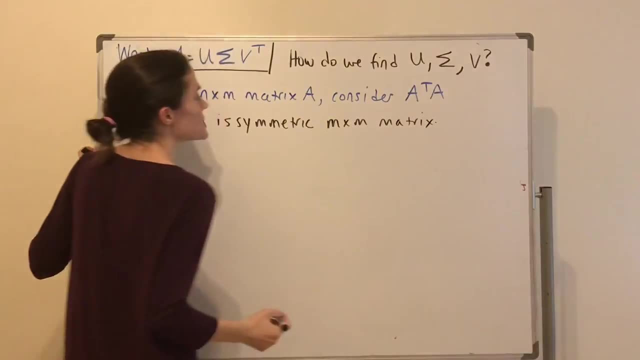 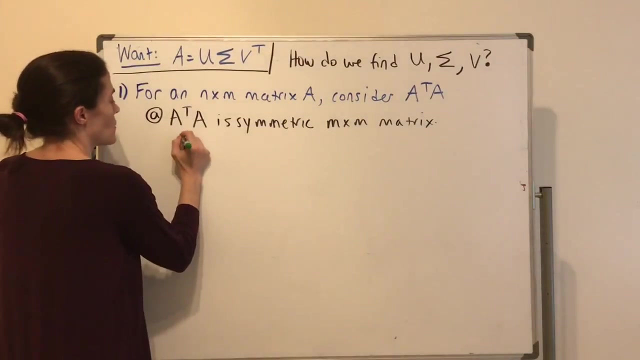 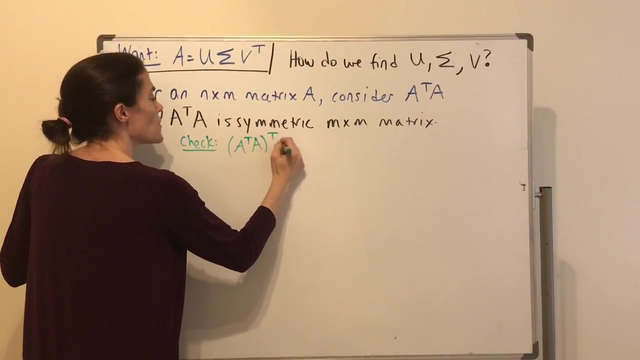 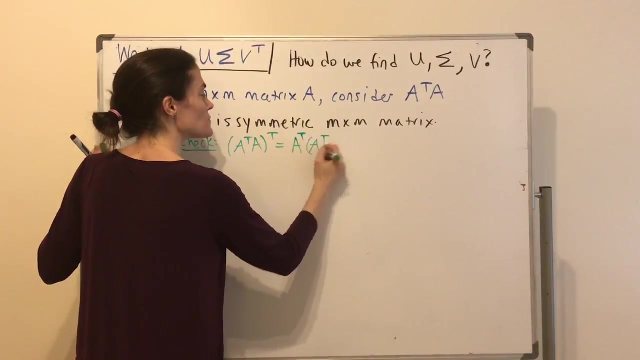 This is N by M, Middle ones match. We get M by M. Okay, the size is definitely that, but why is it symmetric? We can check. I'll do it in green- If we take A transpose, A transpose, this is A transpose, and then A transpose, transpose. 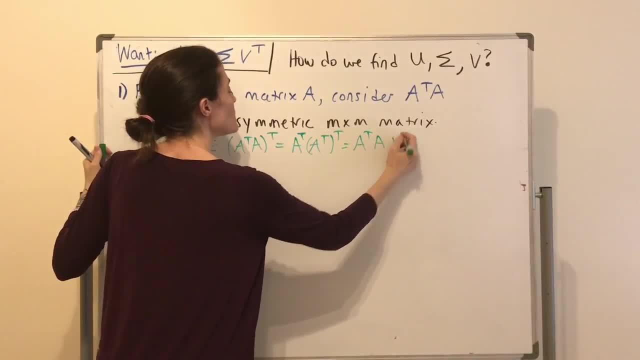 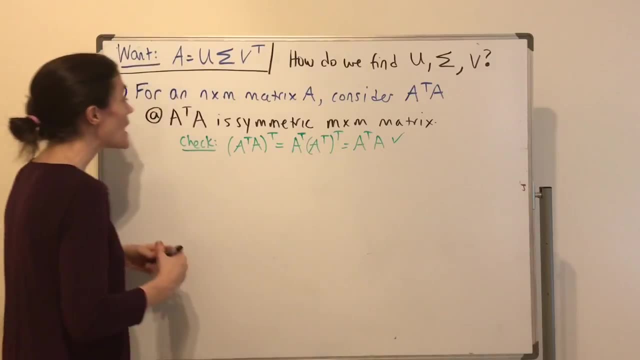 which is A transpose A. So, in fact, just using properties of transposes, this matrix is symmetric. Okay, what does this mean? Well, by the spectral theorem- maybe I'll write this underneath here- So thus, by the spectral theorem. 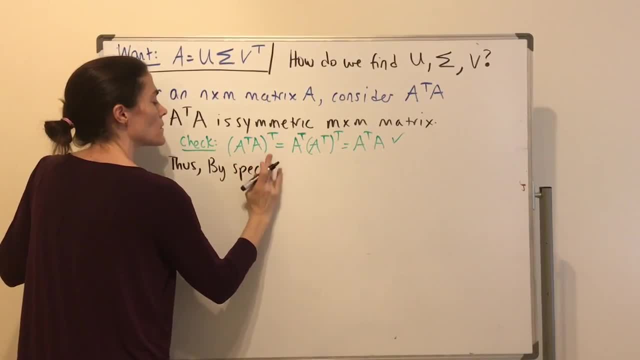 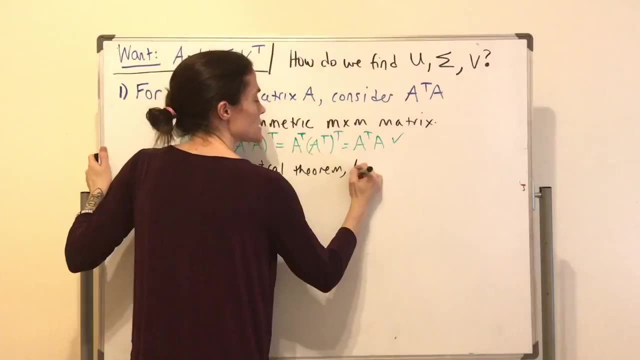 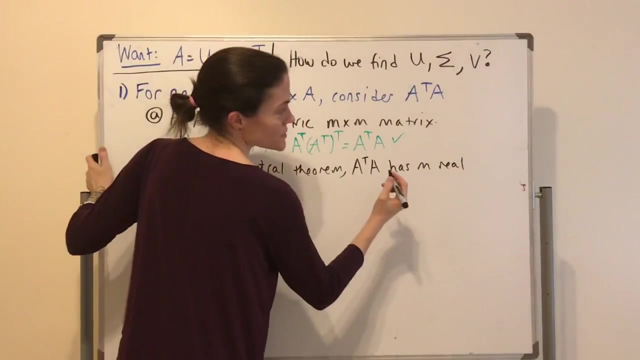 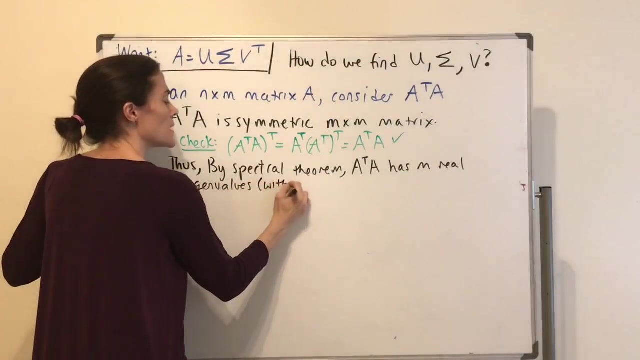 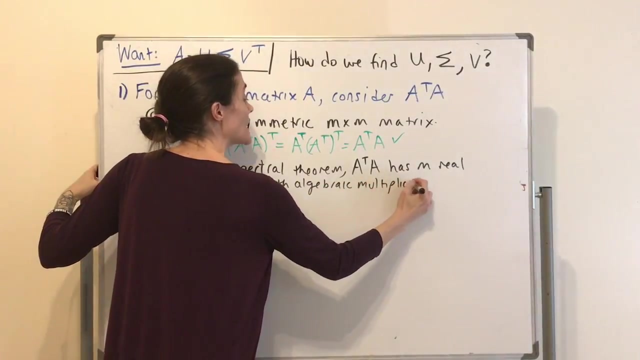 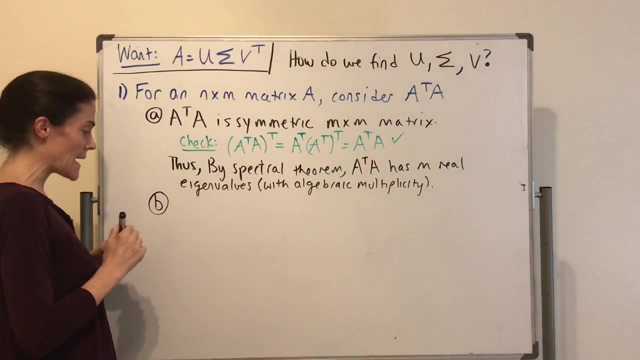 we know that A transpose A has M real eigenvalues, And this is counted with algebraic multiplicity. Okay, we could have repeated ones, this is fine, But we know they're all real. Now I can say more, in fact, And this is my number B, letter B. I can say more, In fact. 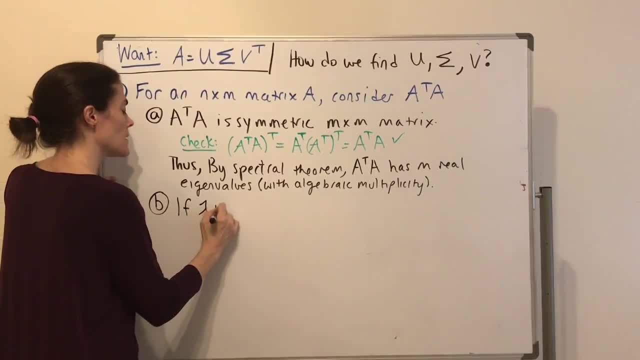 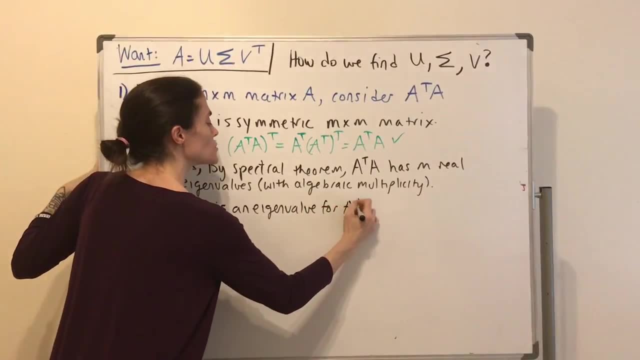 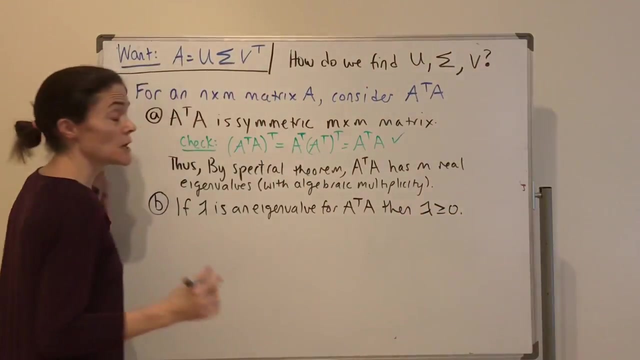 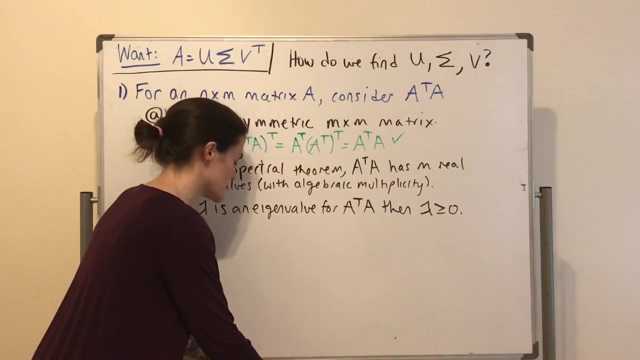 I'll say this: if Lambda is an eigenvalue for A transpose A, then then lambda is greater than or equal to zero. It's more than just being real. It's that it is non-negative, Now okay. well, let's prove this. 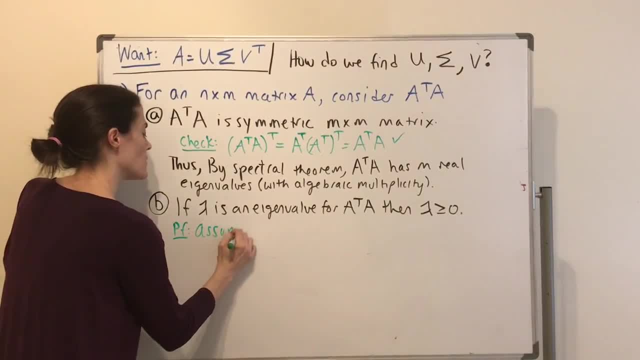 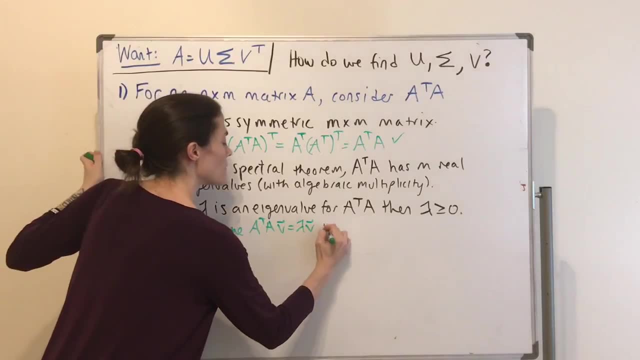 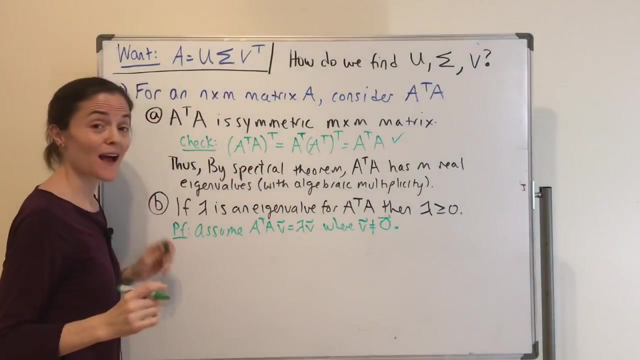 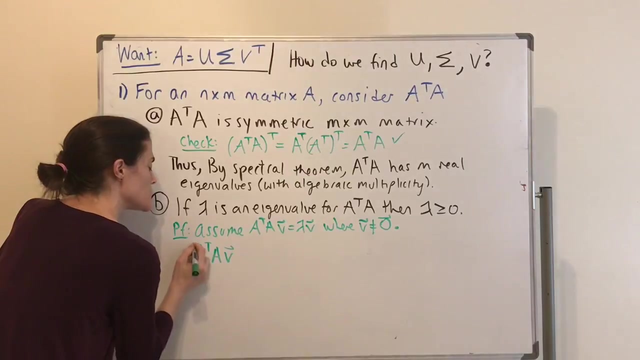 Proof. Okay. so let's assume A transpose A V is lambda, V where V is not equal to zero, So V is an eigenvector for eigenvalue lambda. Okay. well, if I take A transpose A V and I dot this with V, 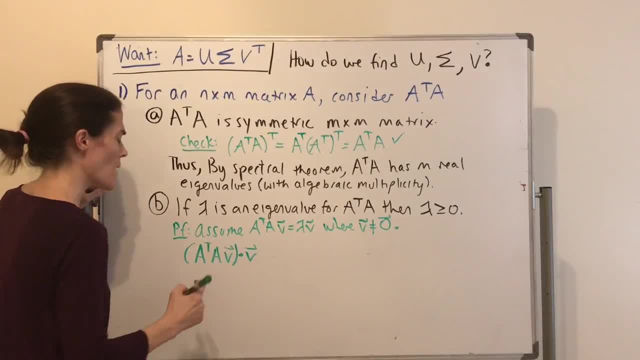 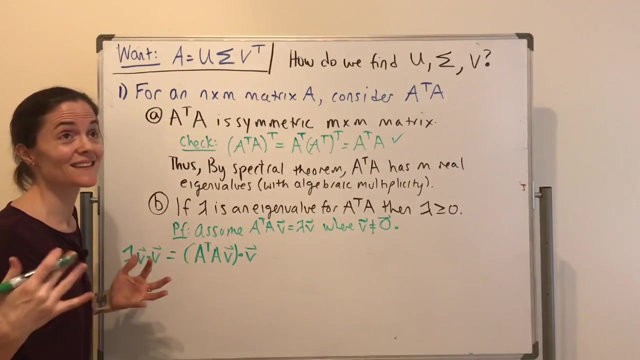 what do I get? Well, on the one hand, V is an eigenvector for lambda With eigenvalue lambda. So I get lambda V dot V. Technically it would be lambda V dot V, but it's a constant, so I can pull it outside. 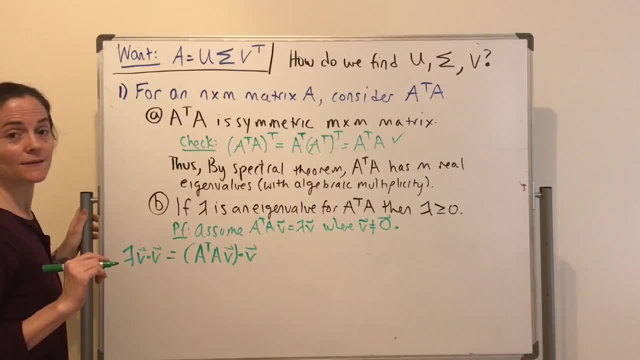 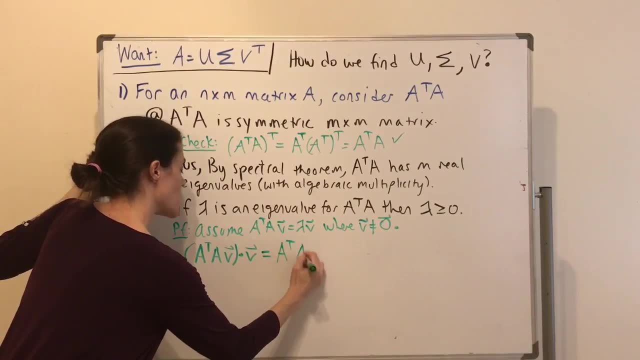 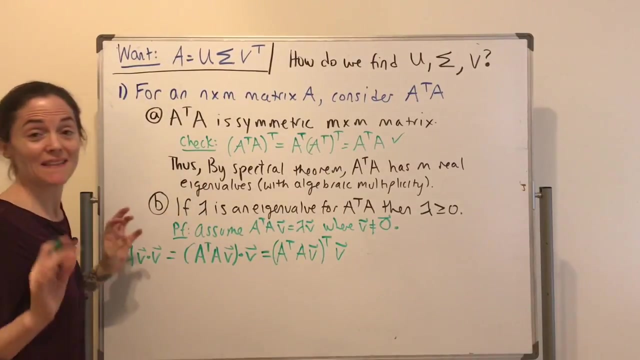 So this is lambda times: V, dot, V. Okay, no problem, Now I can also write this as follows: A transpose A, V transpose V. Okay, this is something we have used. This is just writing the dot product as a matrix product. 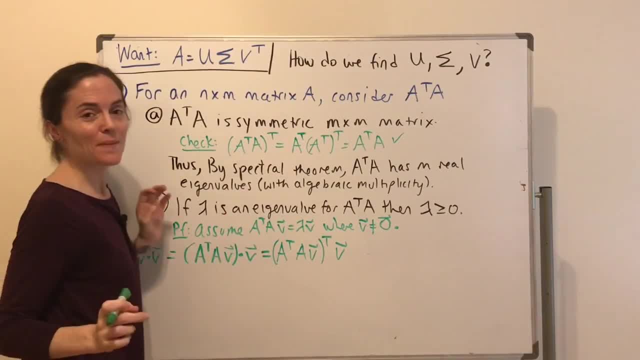 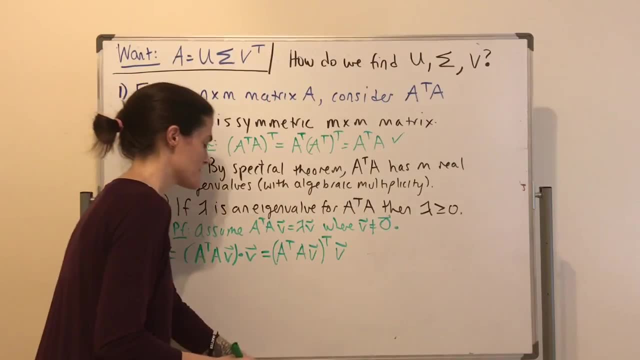 And now I'm gonna use sort of similar properties I did up here when I take a transpose of a product. Well, here's what I'm gonna do. I have some options, but I'll tell you what I will do. Ah, I'll underline in brown. 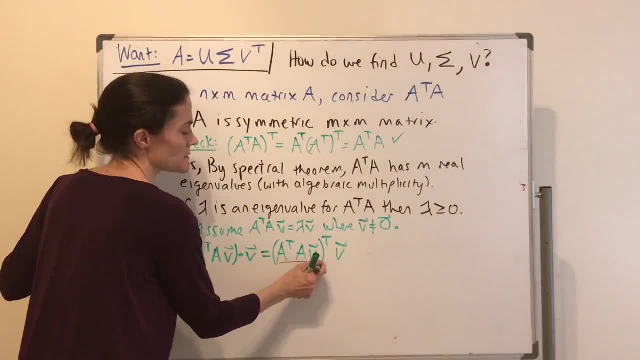 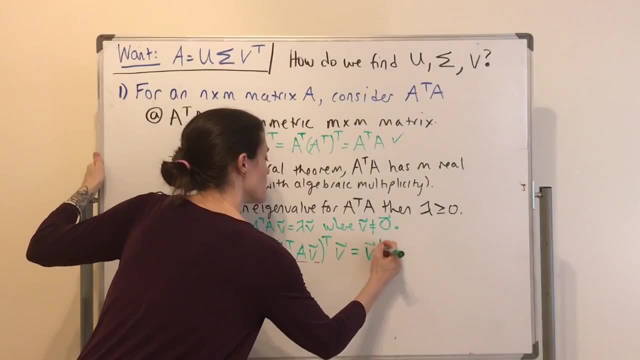 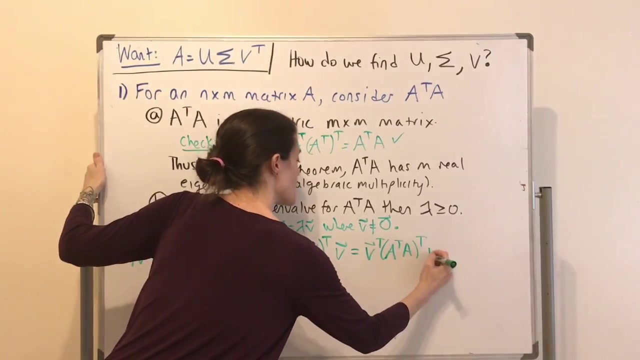 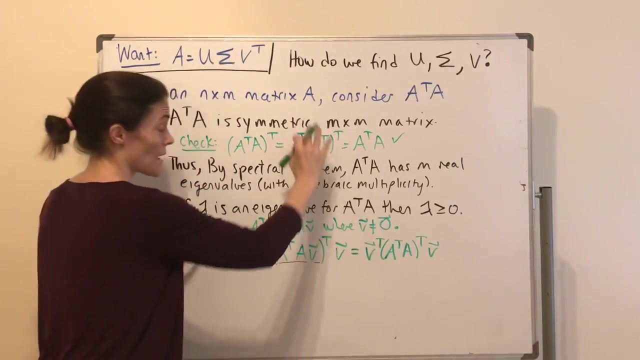 I'm gonna think about this as this times this: okay, So this would be equal to V transpose and then A transpose, A transpose and then V. okay, A transpose, A is symmetric, So this transpose is itself. That was in the first part. 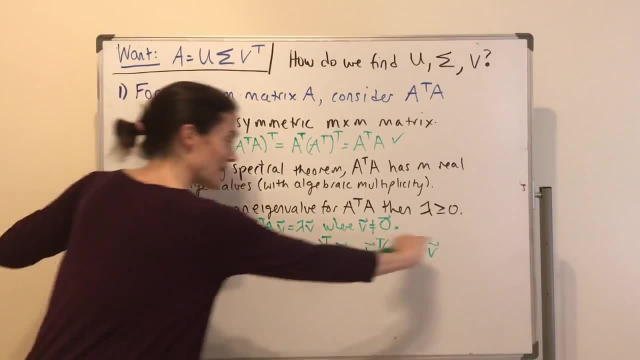 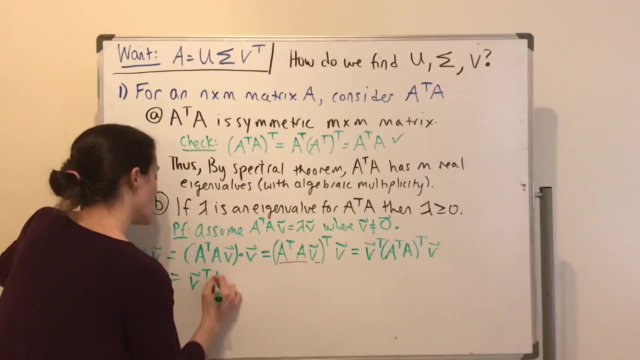 And so this becomes: maybe I'll move here. I have a big long equals. then I come here. Okay, this becomes V- transpose A, transpose A V. And now one more step. Look here I can use the same property again. 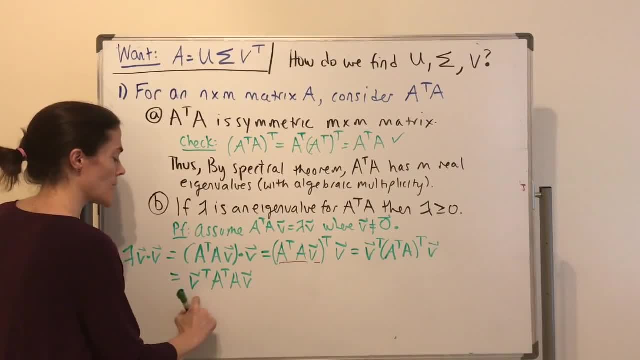 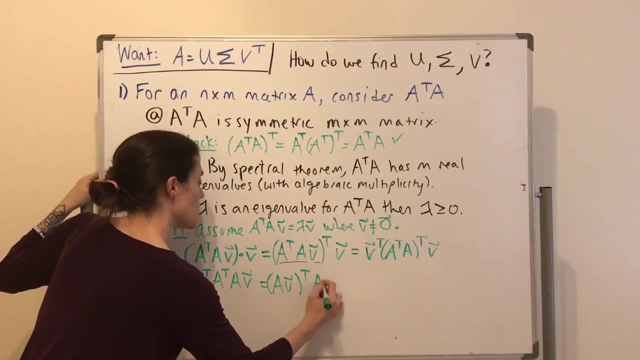 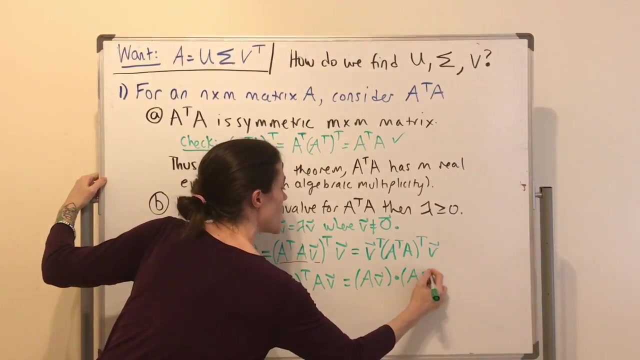 that this is A V. transpose A V. And then my final observation is: this is A V dotted with A V. Now, why did I do this? Well, any vector dot itself is greater than or equal to A V, So I can use this as a vector. 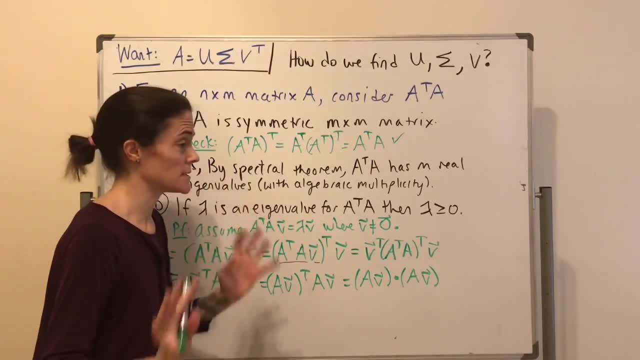 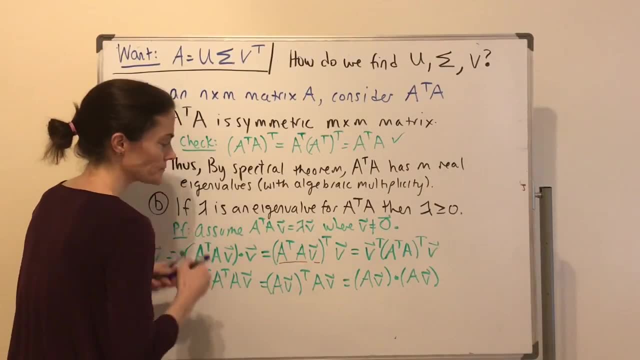 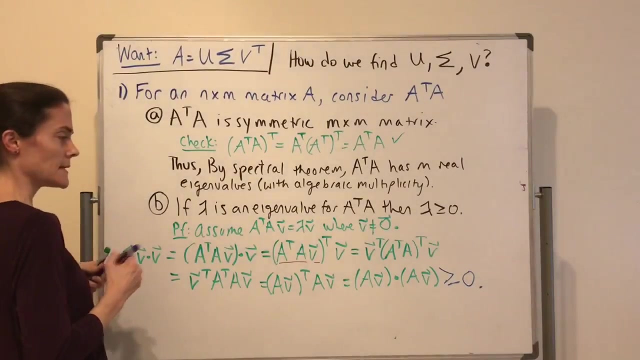 So I can use this as a vector. So this vector itself is greater than or equal to zero, And the only way it's equal to zero is if the vector itself is zero. So I can confidently say this: Okay, which means now, what is it on this side? 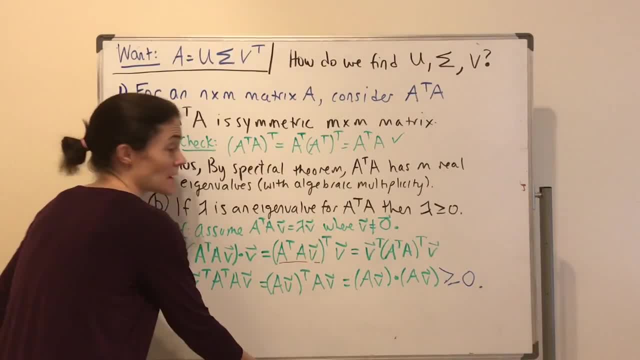 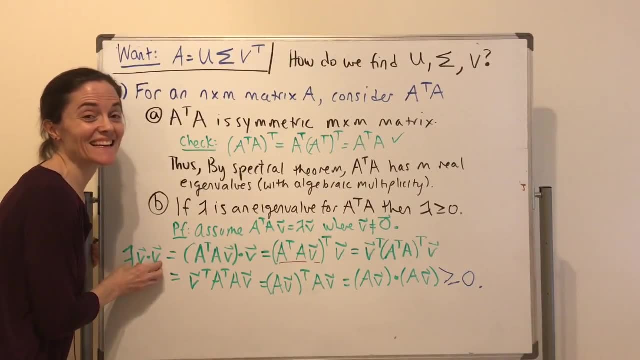 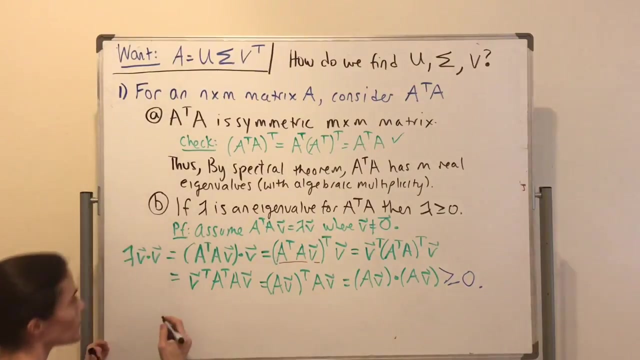 It's lambda times V dot V And V dot V is non-zero. This is non-zero, So I may divide. well, it's not only non-zero positive. Okay, So I may divide and we obtain, or we see, that lambda must in fact be greater than or equal to zero, And this is what I was trying to prove. 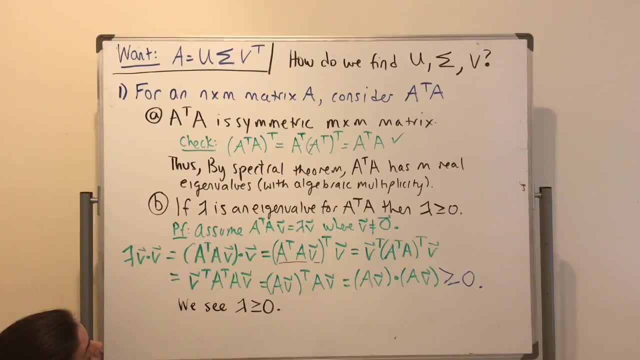 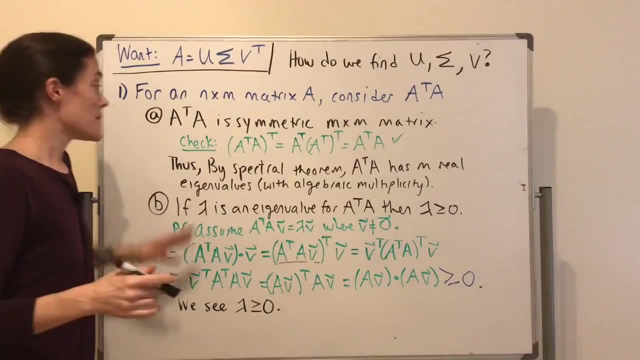 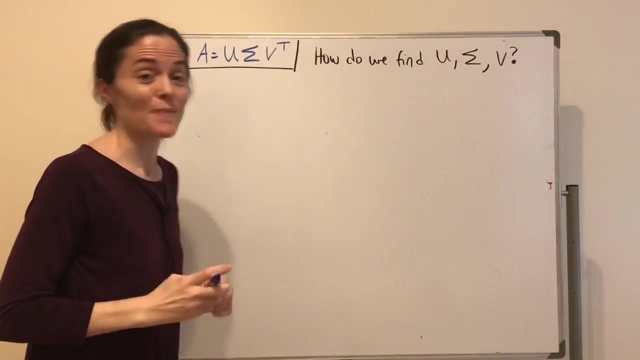 Okay. So if you have an eigenvalue, okay, very nice For this. A transpose A is greater than or equal to zero. So now maybe I'm going to erase and we will continue with our discussion Part two. we had part one which was thinking about the matrix A transpose A. It's symmetric. 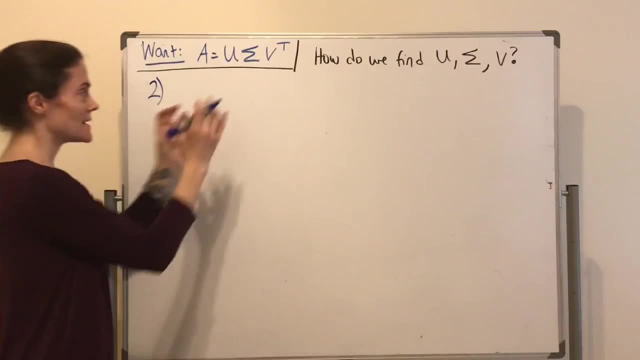 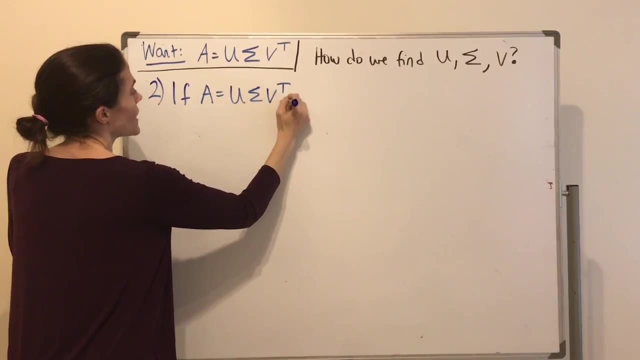 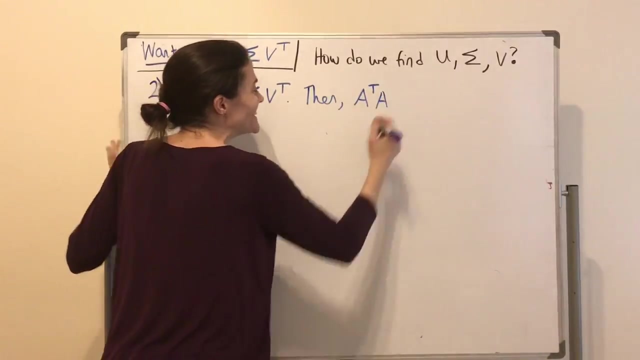 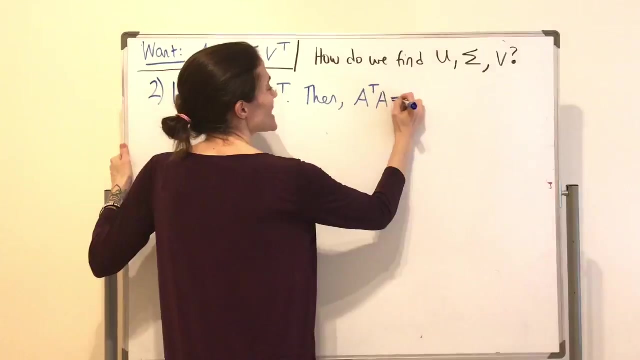 All the eigenvalues are non-negative. Now part two is: if A is in fact this, Okay. Well, what is A? transpose A: Okay. Hopefully you could have realized by my number one that this was going to come into play sometime in today's discussion, or otherwise I wouldn't have taken the time to do that Well. 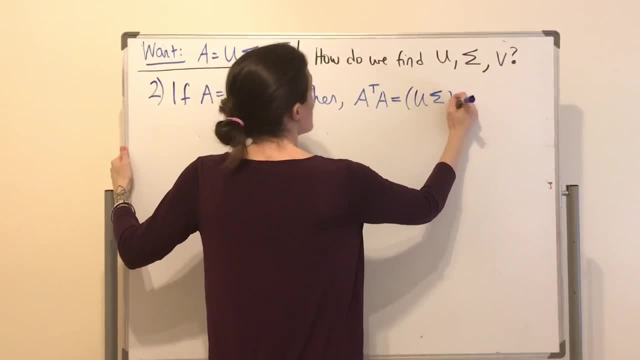 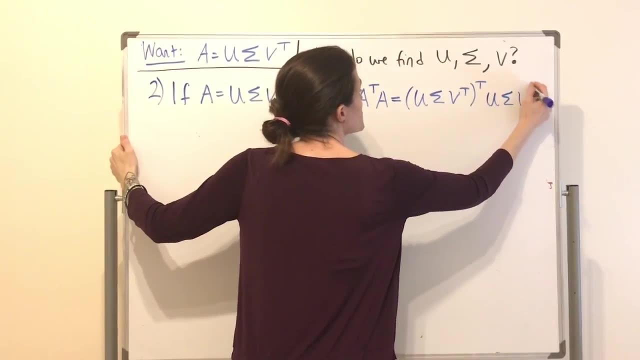 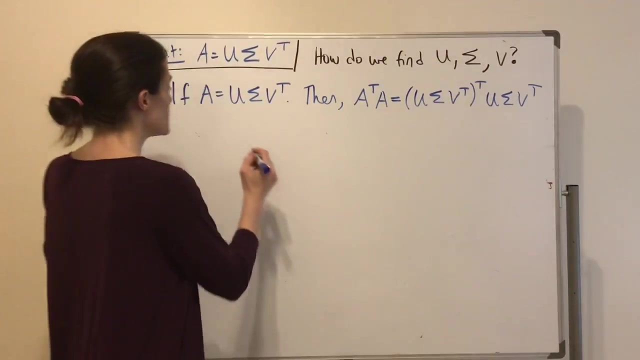 here we go. It's U sigma V, transpose, transpose, U sigma V, transpose. And again I have this property of taking the transpose of a product, So we get that A transpose A is it's going to be V, transpose, transpose, which is V. 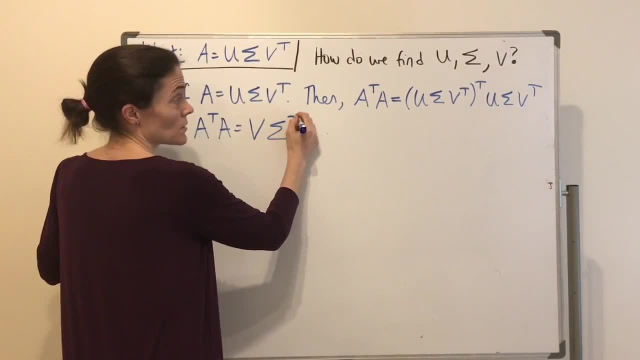 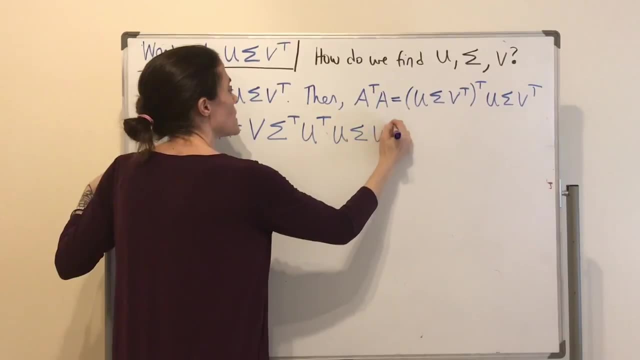 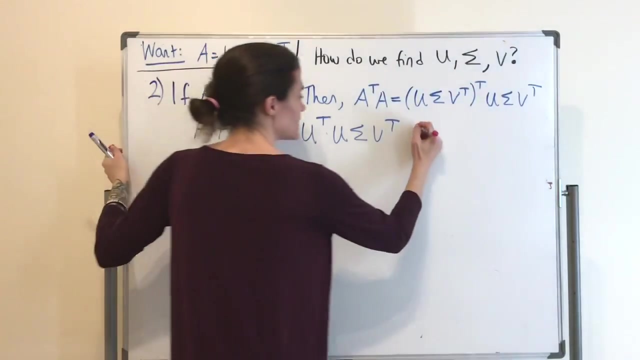 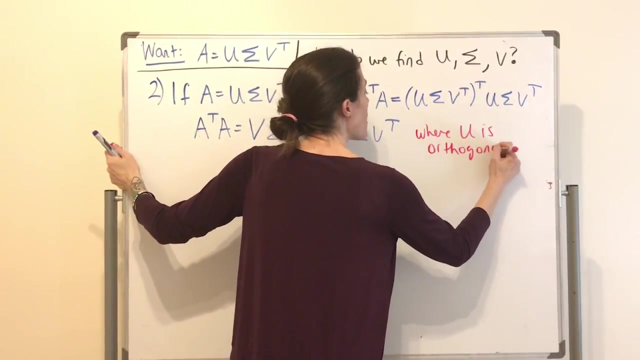 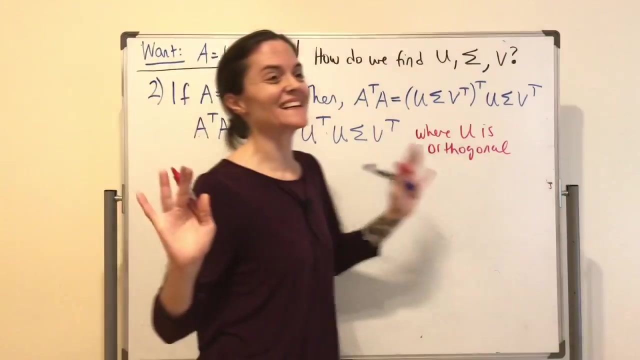 It's going to be sigma transpose, And then it's going to be U transpose, And then we have U sigma V transpose, where this is when it gets cool, where U is orthogonal And recall an N by N matrix, or let's see what's the size of U: A is U? is N by N? Good, Okay. 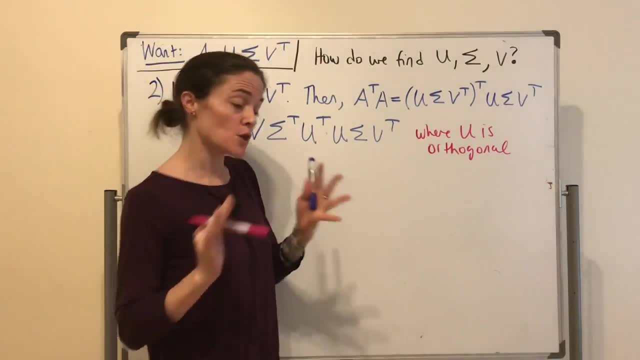 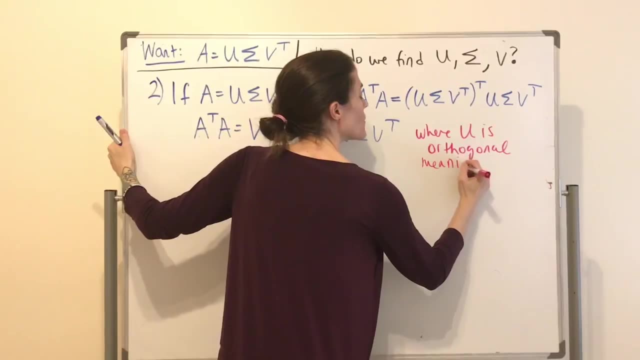 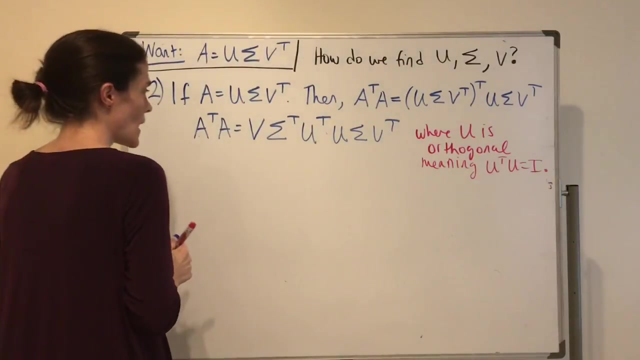 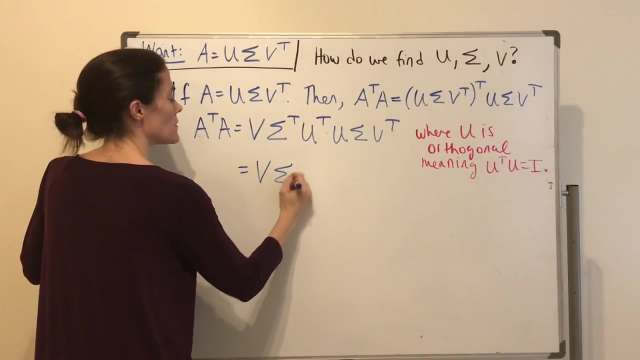 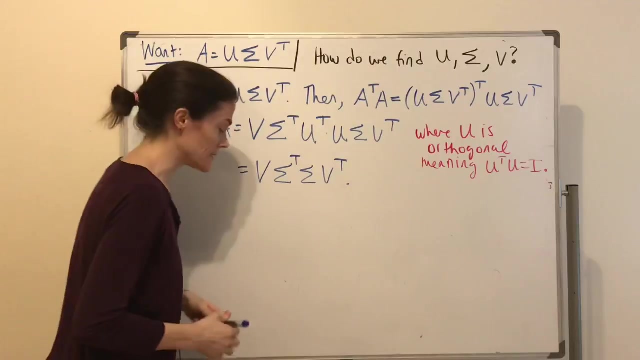 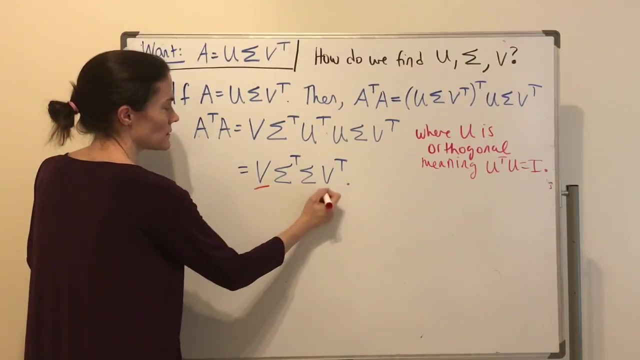 An N by N matrix is orthogonal if, and only if, U transpose, U is the identity. Okay, And so this equation, here it becomes. this is the identity We get: V and V transpose. Now look at what we have here: Orthogonal matrix, It's transpose This thing. well, what is this, If you think about it? 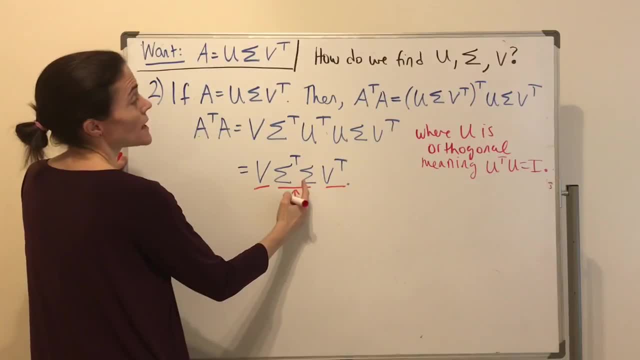 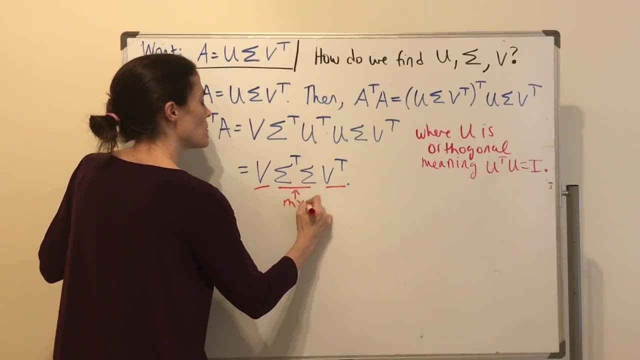 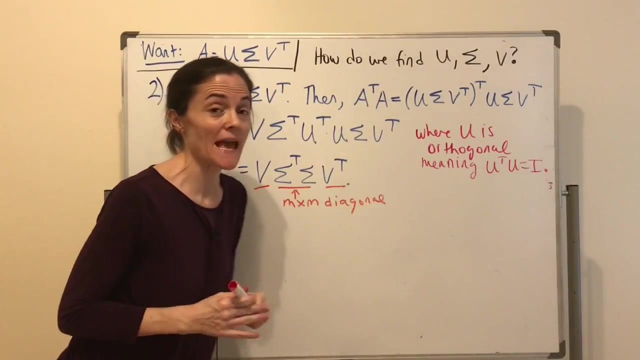 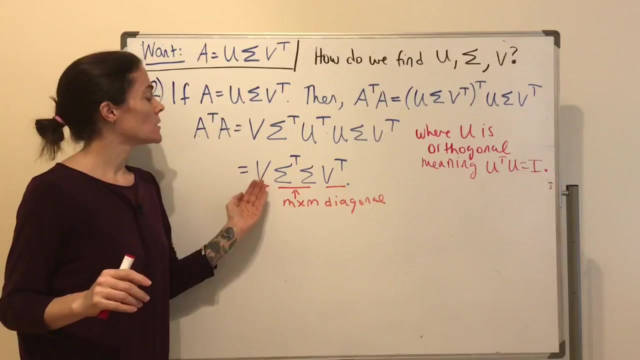 this sigma was N by M. This is going to be M by N, M by M. This is M by M, and it is diagonal. Okay, So look at what we have. We have decomposed this symmetric matrix A. transpose A into orthogonal matrix. 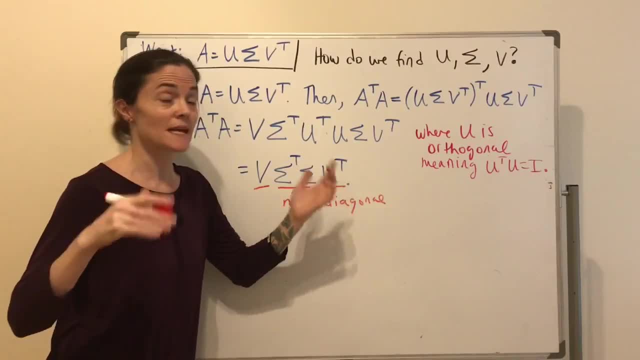 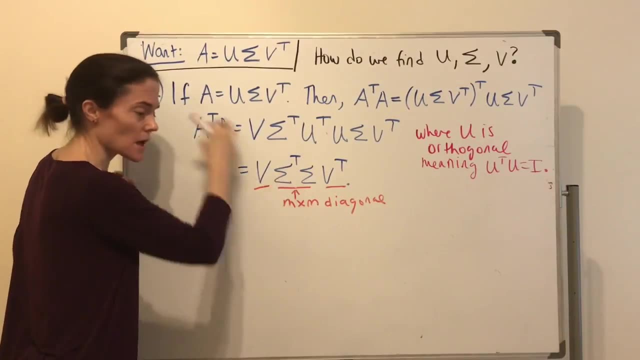 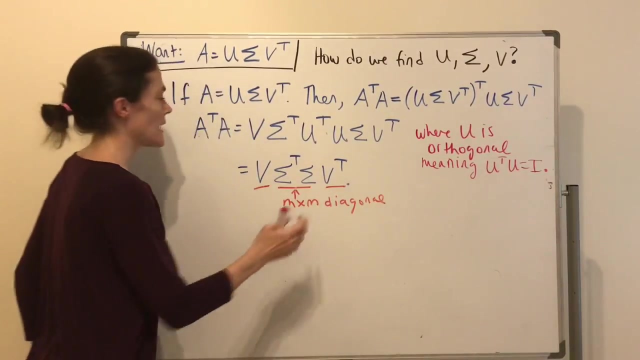 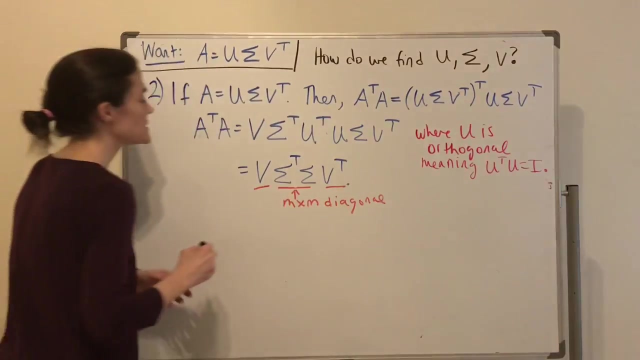 diagonal matrix, orthogonal matrix. transpose That says that this is the, the eigenvalues along the diagonal, This, well, this one would be the eigenvectors. and then there it's transpose. Okay, So now we know how to find V and sigma like this: Okay, 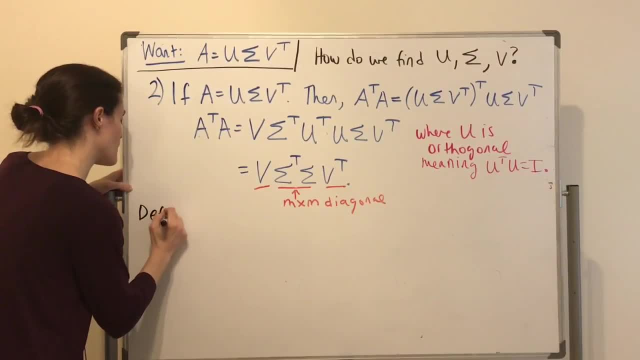 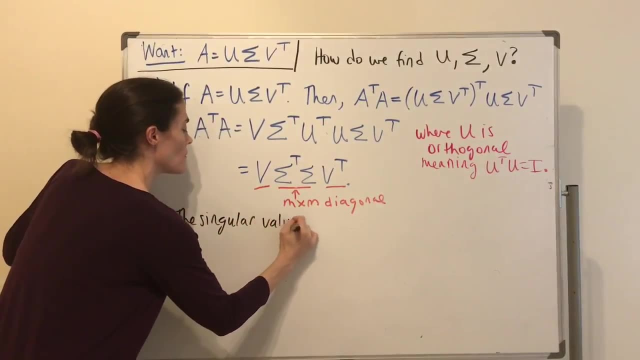 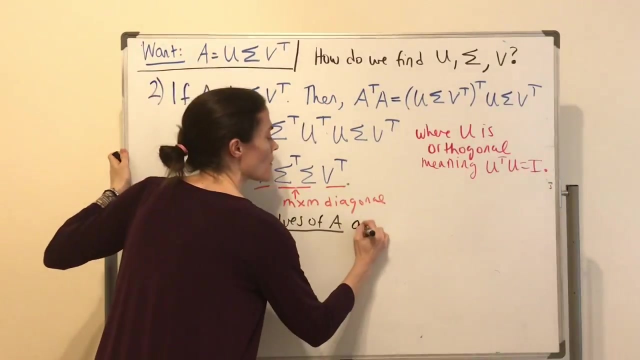 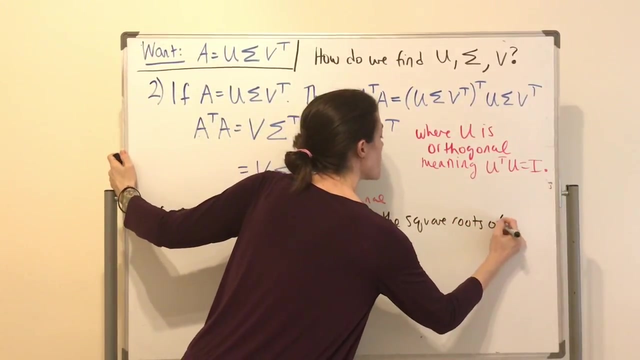 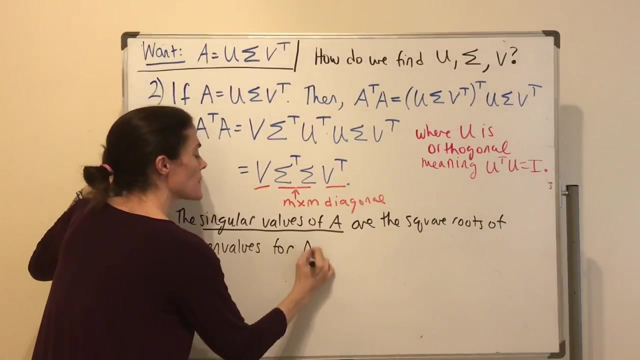 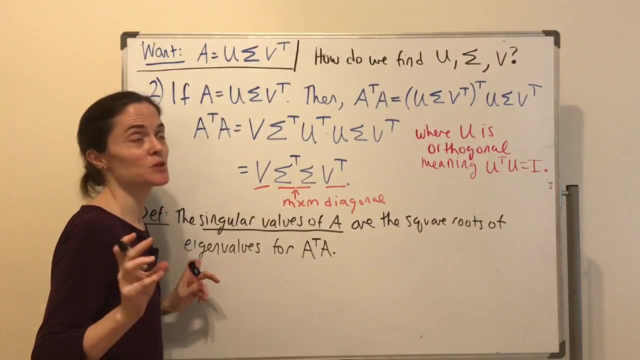 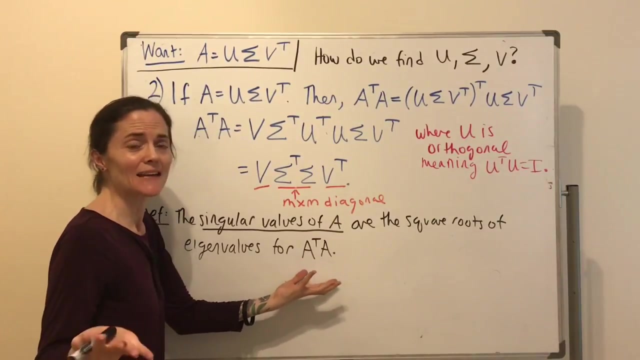 So definition: the singular values of a matrix are the square roots of the eigenvalues for this matrix. Okay, Now, that's why I spent the time to just, you know, justify why the eigenvalues for this matrix, A transpose A- were non-negative. because you need that to take the square root. 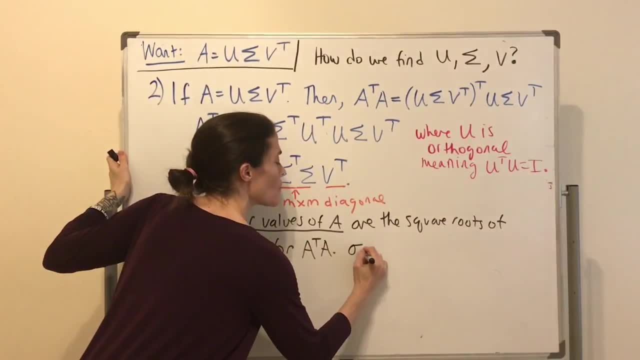 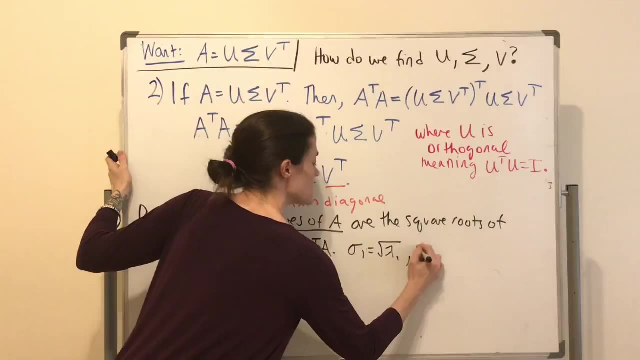 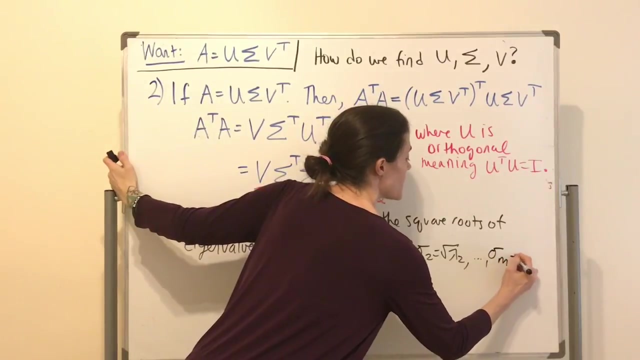 Right, And typically we will say, for example, sigma one: this would be the square root, lambda one. sigma two is the square root, lambda two out two. Well, it's going to be. it's M by M. 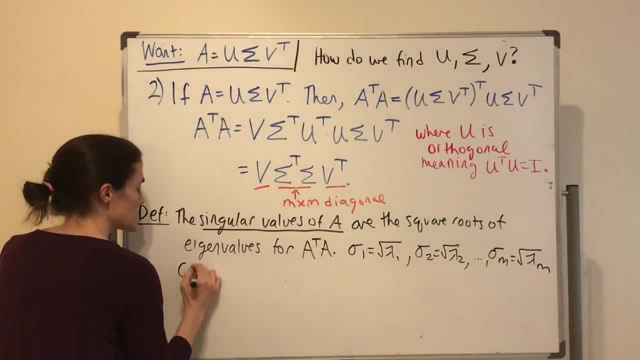 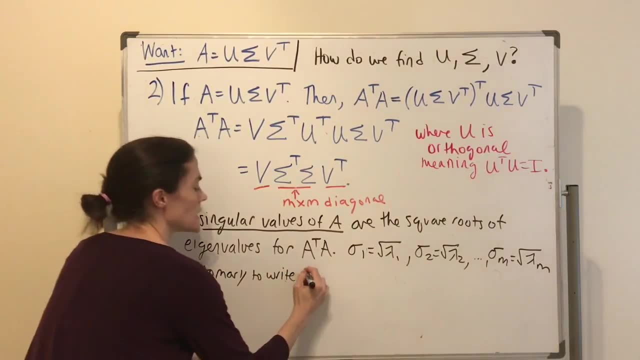 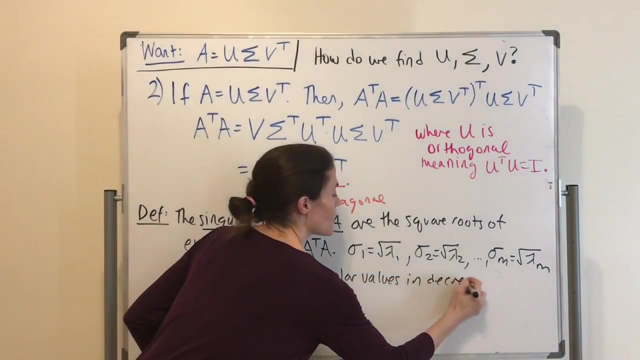 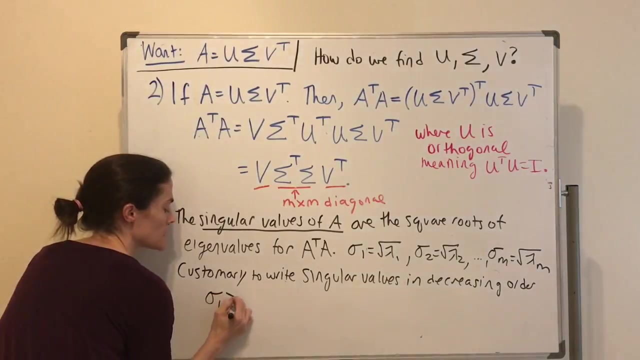 lambda M, And it's very customary to write the singular values in decreasing order, So we would write them such that sigma 1 is bigger than or equal to sigma 2, is bigger than or equal to sigma 3,, all the way out to sigma m. 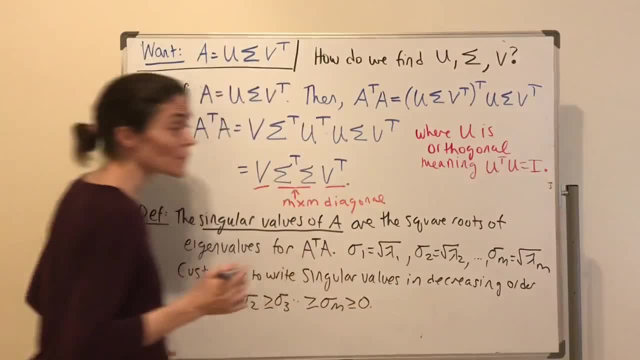 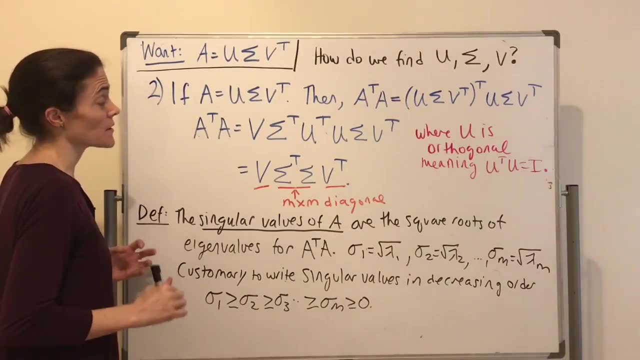 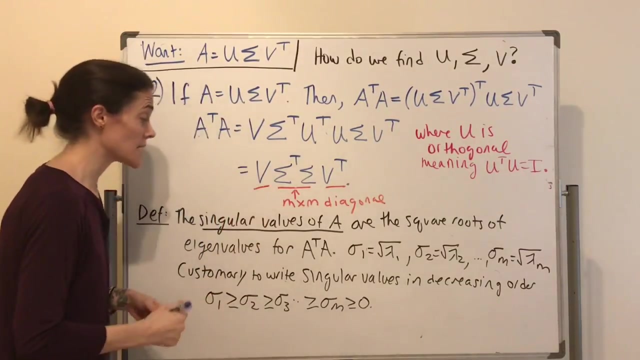 which is bigger than or equal to 0.. And we're taking the positive square root here of these non-negative numbers: lambda i. Okay, so these are the singular values And these will what be, what will be along this diagonal of sigma. 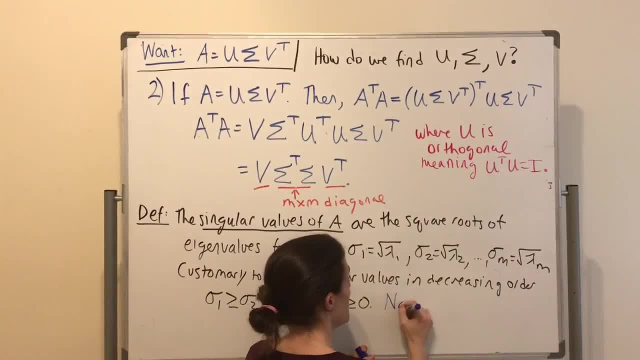 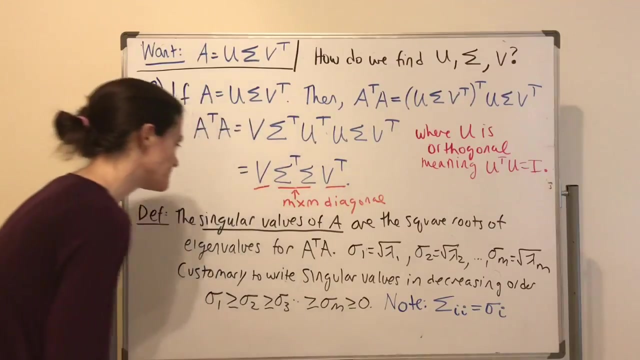 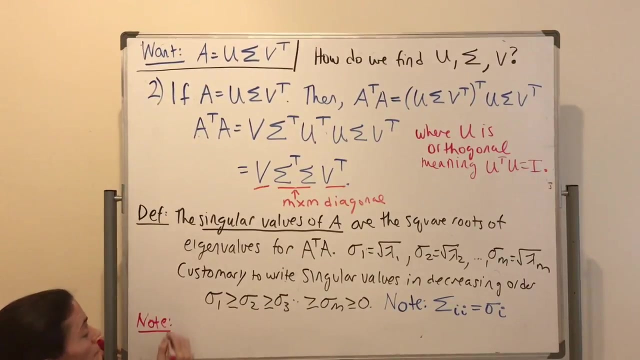 Maybe I'll make that comment here. So note: the sigma matrix satisfies that the ii position is this Sigma i. okay, But one comment, and I think I can make it here at the bottom, is that I'll just state it here before I erase and move on. 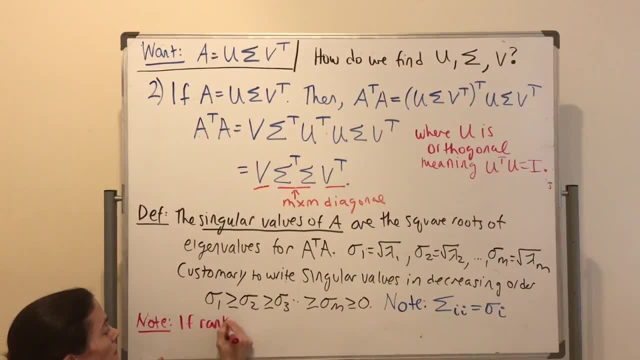 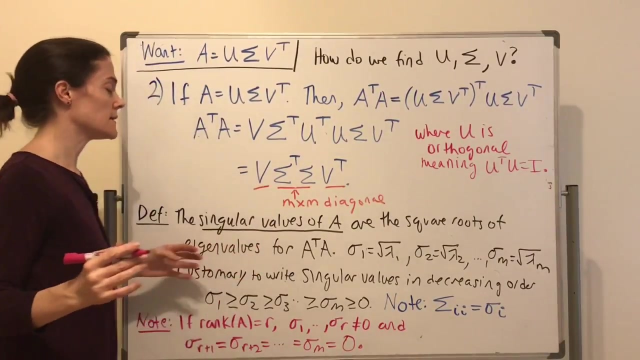 is that if the rank of a is r, then sigma 1 out to sigma r are not equal to 0. And sigma sigma r plus 1, sigma r plus 2, out to sigma m are all 0.. Okay, that's something that I mentioned when I mentioned the singular value decomposition. 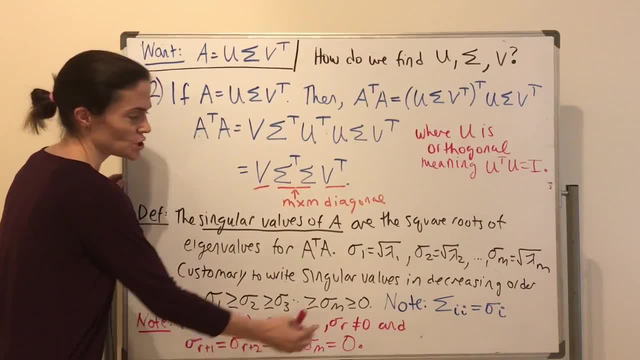 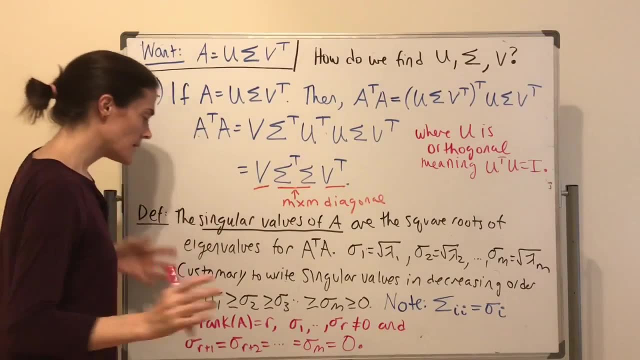 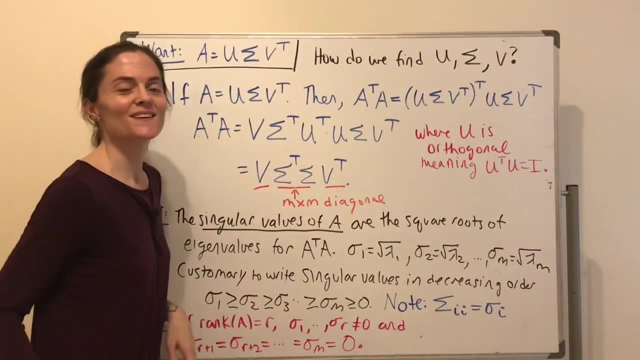 is that we had, just along the diagonal out to the rank of the matrix, we had non-zero things and that was it. Okay, These are the singular values, These are the singular values of a matrix that come up in this singular value decomposition. 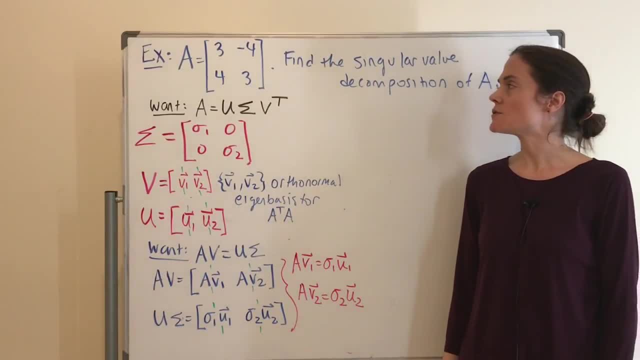 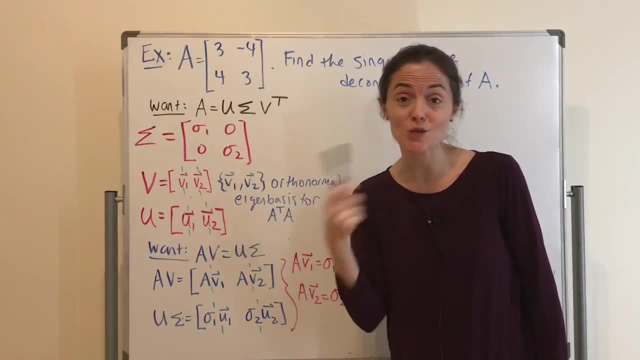 This is our first example, And what I'd like to do is talk about how are we going to find these matrices, And then we'll work. the example: This matrix A, is two by two. We see it's not symmetric, but it doesn't need to be. 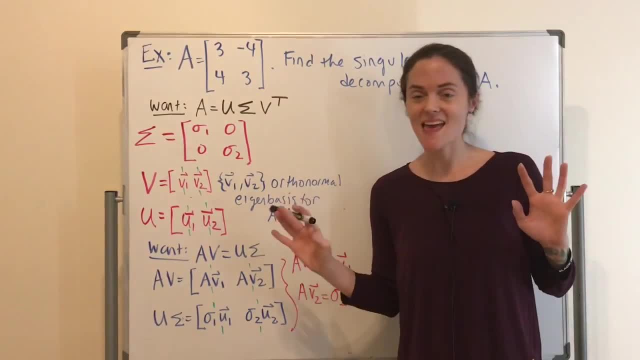 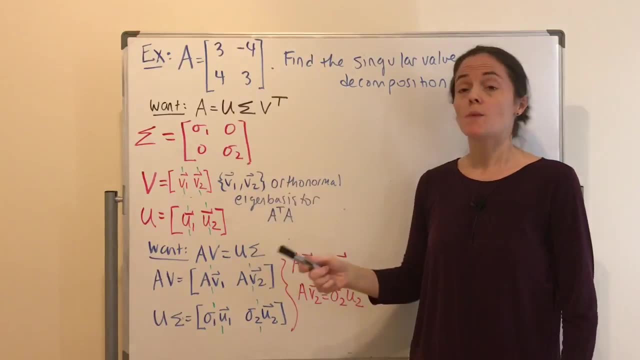 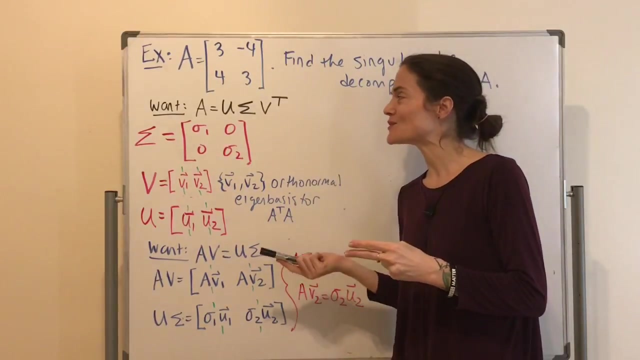 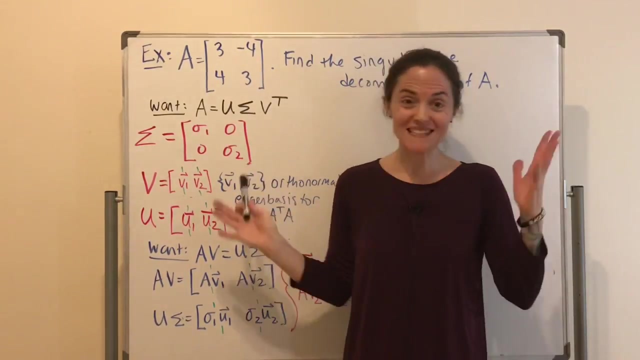 Singular value decomposition works with any n by m matrix And what we want is: A is U sigma V transpose where U and V are both orthogonal matrices. In this case, because A is 2 by 2, U and V will both be 2 by 2, and this sigma will be 2 by 2.. 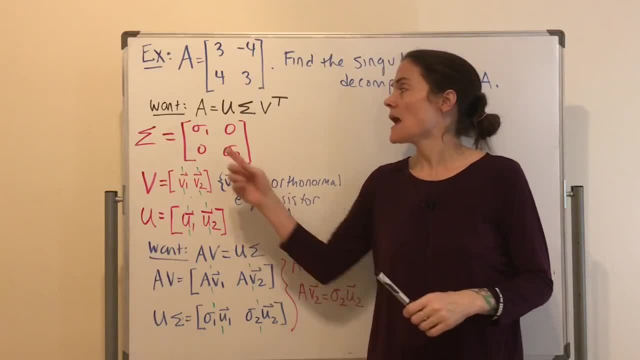 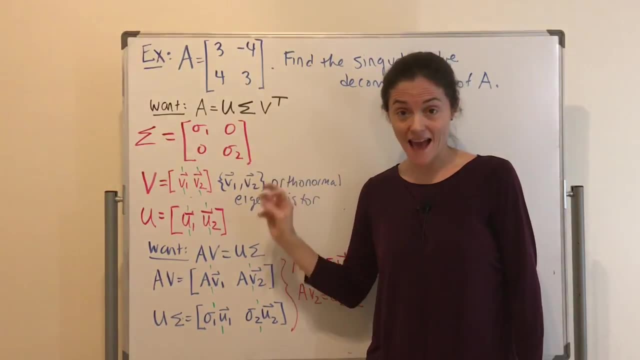 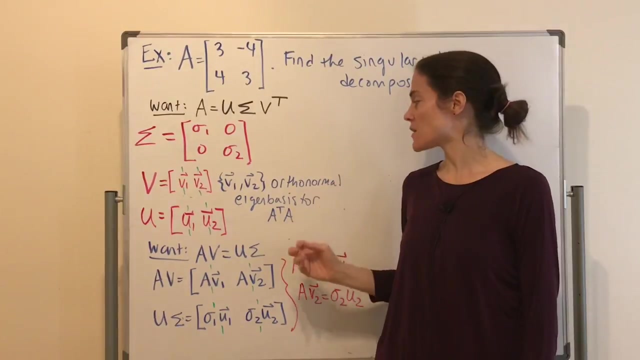 It will be diagonal because A is square And this we just talked about. It will have these singular values of the matrix A along the diagonal. Well, sigma 1 and sigma 2 are square roots of the eigenvalues for A. transpose A. 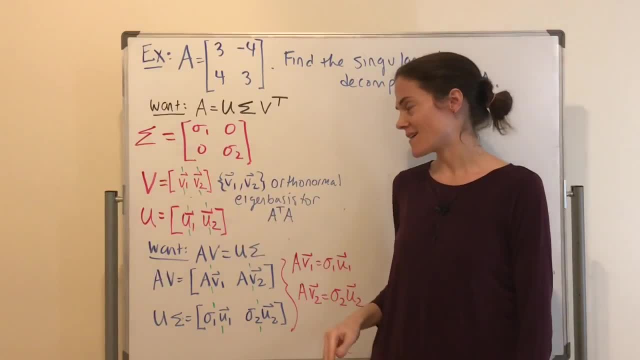 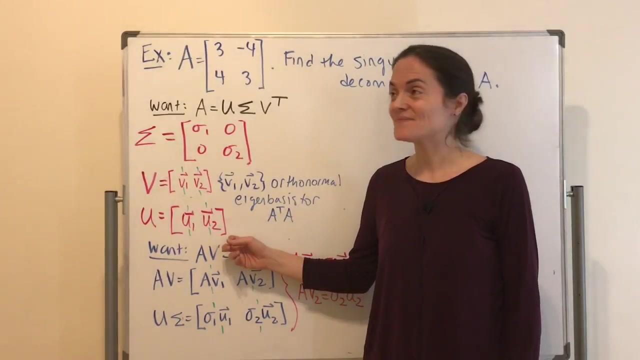 And then the matrix V, which is right here, the columns. well, because V is orthogonal, we will have the columns will be in, or the normal eigenbasis for the matrix A transpose A, Okay Then. Well, we need to discuss how do we find U? and that I didn't really do yet. 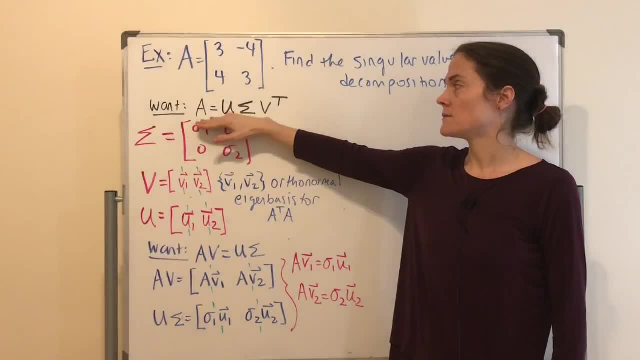 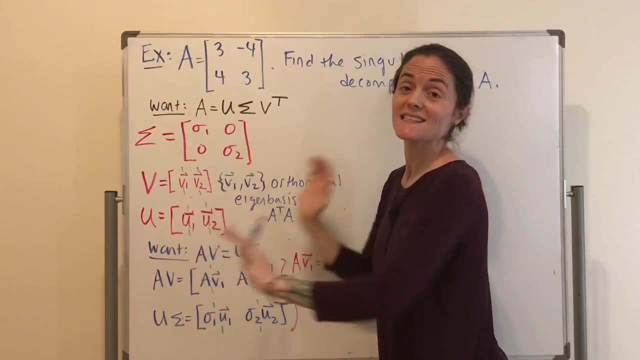 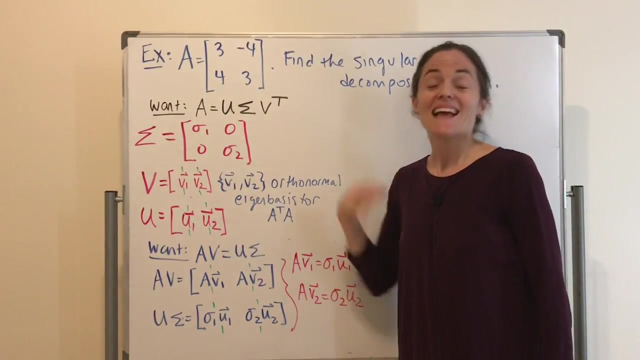 So what I'm going to do is: let's take this and multiply on this side by V, So V is an orthogonal matrix, V transpose. V is the identity. The right-hand side becomes U sigma and the left-hand side becomes A V. okay, 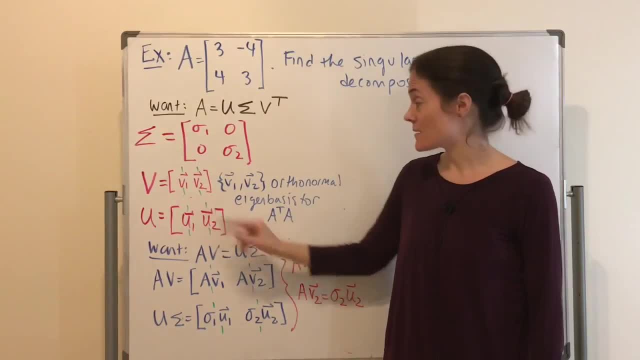 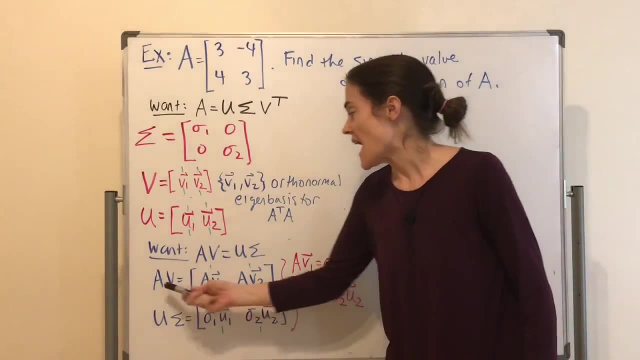 And then, well, I know what V looks like. It has these two columns, and I know what U looks like. It's going to have some U1, U2, and then I know what sigma looks like. A V has columns A V1 and A V2, U sigma. 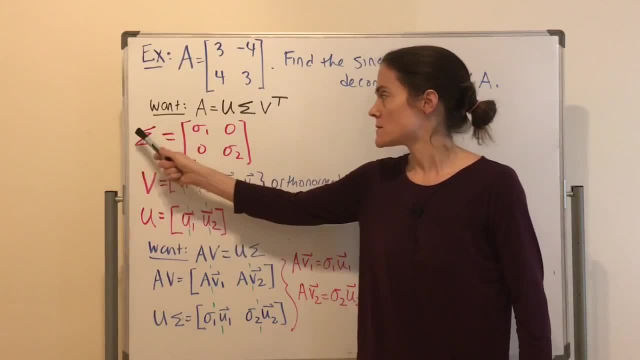 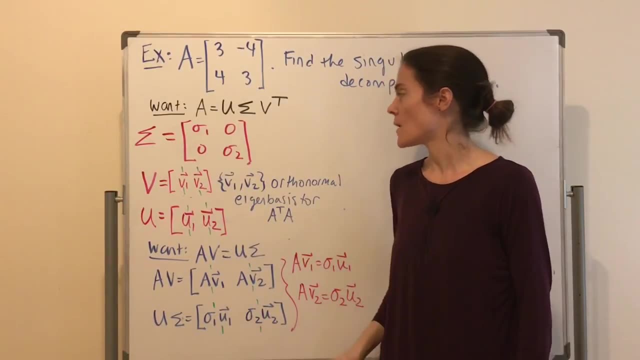 Well, if you multiply U- sigma, the first column would be U times this column, which would be just sigma 1, U1.. And the second column would be U times this column, which would be U sigma and U1. 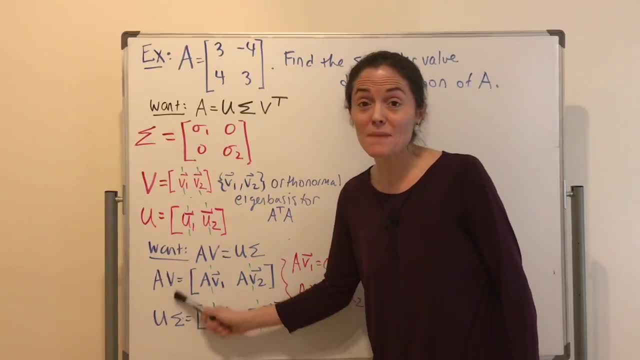 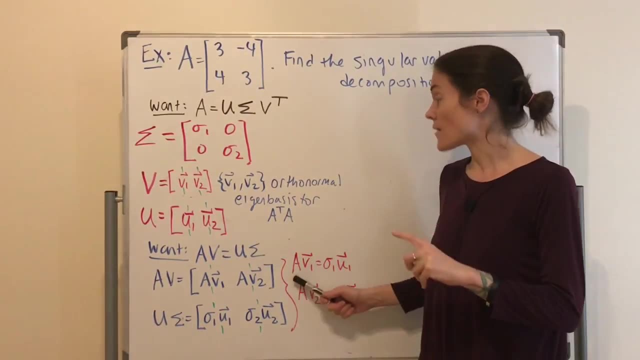 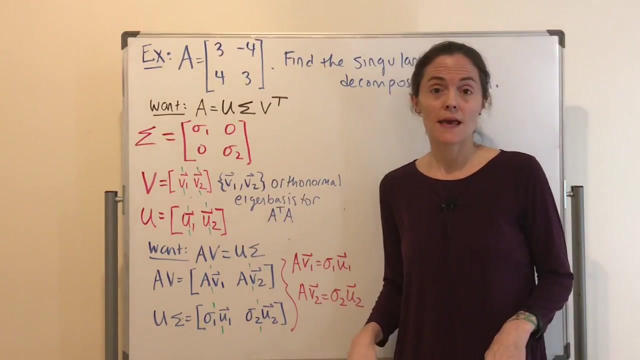 Okay, Now these two matrices are equal. Then we get these two equations. So look, once we have, We already have A given in the problem. Once we have, Then we calculate sigma and V. okay, Just by finding the eigenvalues and associated eigenvectors. 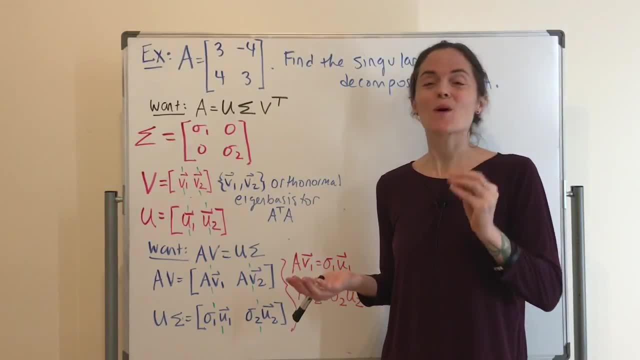 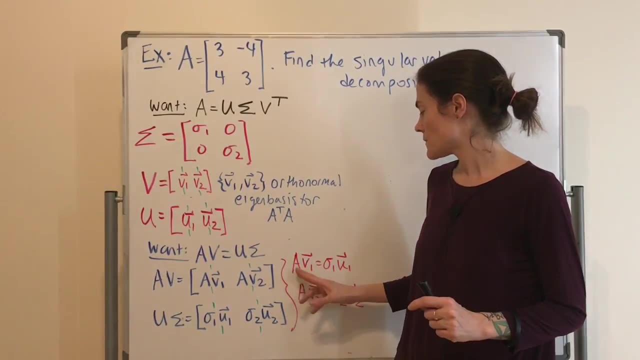 We might have to divide by the lengths to get orthonormal eigenvectors, But we have A sigma U2.. Okay, a v, and then we use this. We have sigma one. We have everything here except this vector. 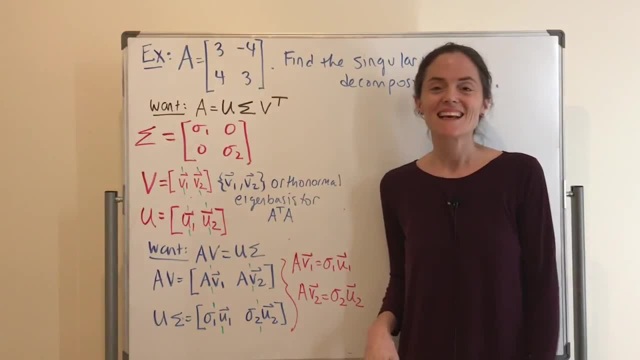 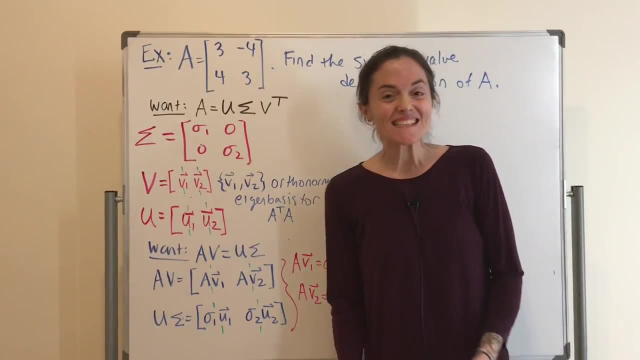 and we can get it from this equation and similarly from this equation. So this is how we will find u1, u2, which are our columns. Okay, well, let's do this now. Maybe I will just try and draw a line. 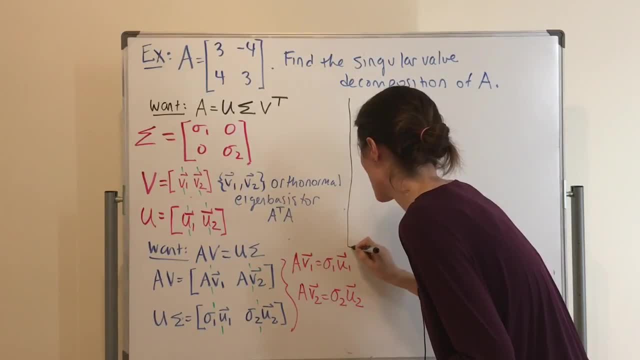 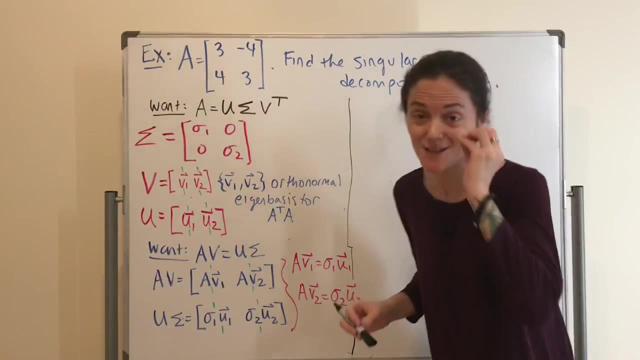 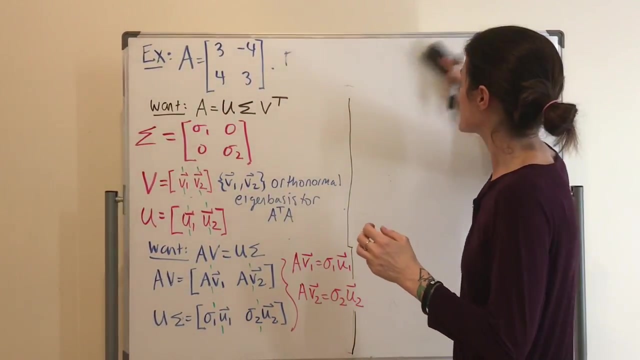 Leave this up if I can, although maybe I will erase if needed. Okay, so the first thing: to compute a, transpose a. In fact, maybe I'll erase this. We know what we're computing: singular value decomposition. I'm gonna erase the instructions because we know it. 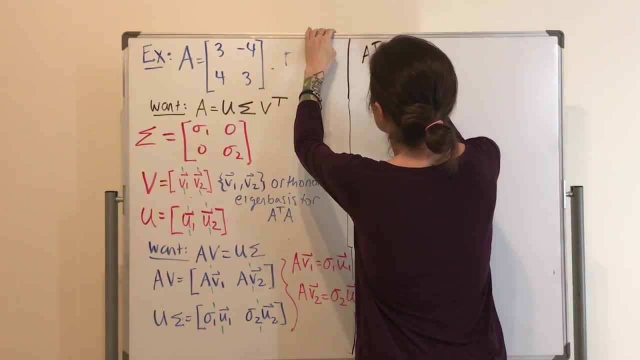 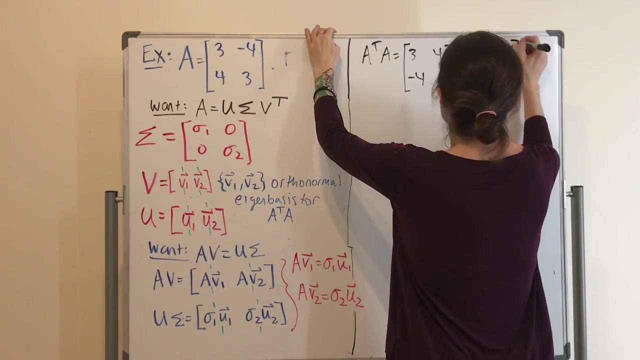 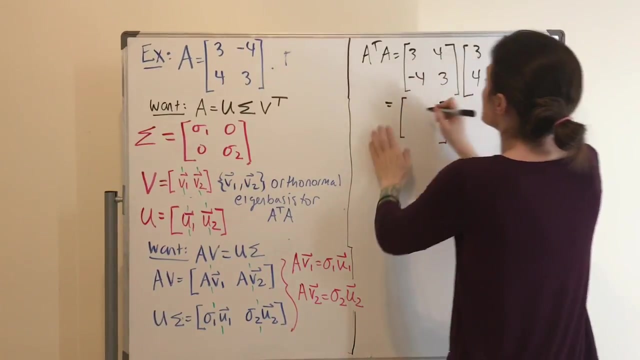 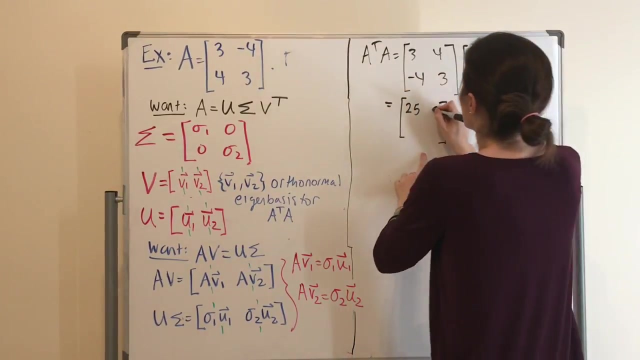 Okay, so a transpose: a Three minus four, Four, three times We have three minus four, Four three. This equals We get nine and 16.. We get minus 12 and 12.. Minus 12 and 12.. 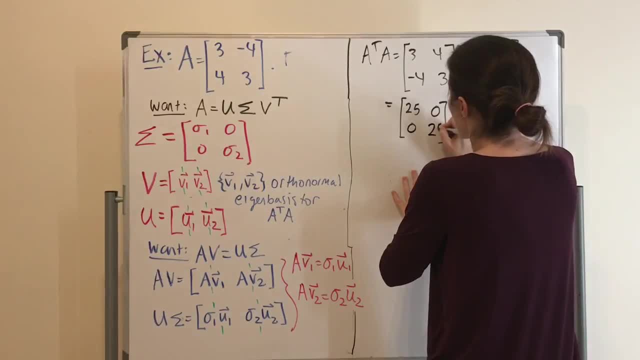 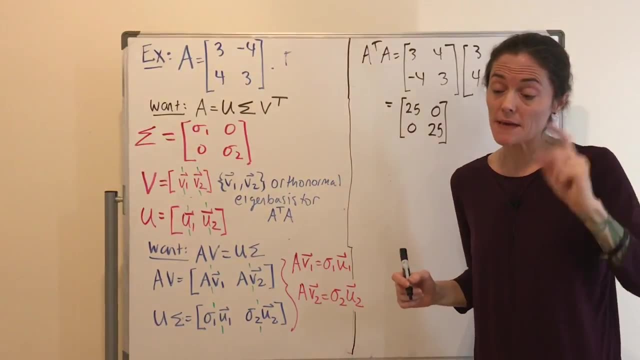 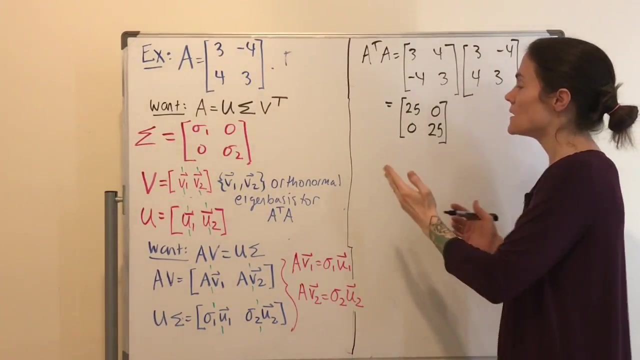 And 16 and nine. Okay, well, this you see immediately. this is a diagonal matrix. I immediately know the eigenvalues 25 and 25, and I know an orthonormal eigenbasis. I can just take one zero and zero one. 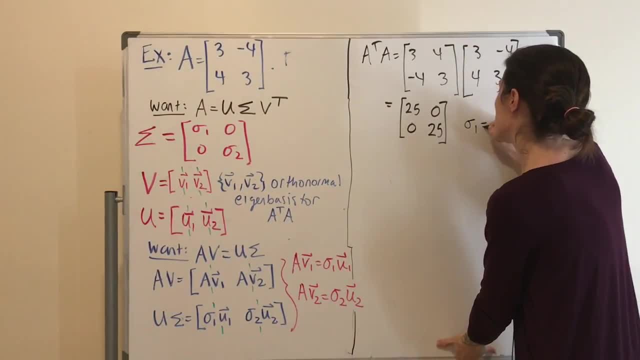 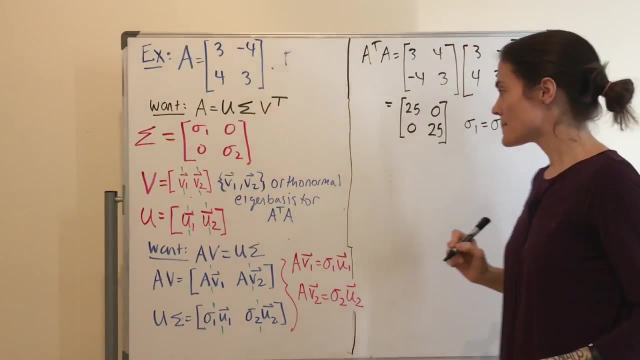 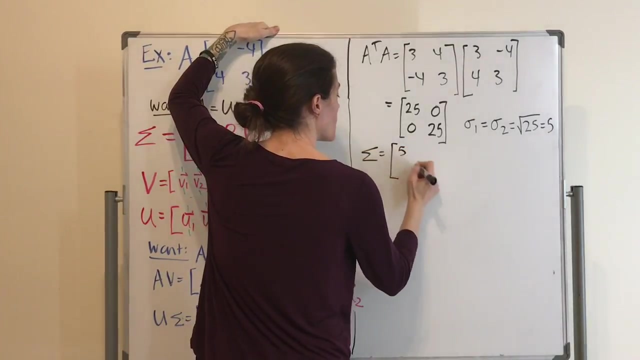 but let's write this down So I can have sigma one and sigma two. They're both the square root of 25, which is five. okay, So I know my matrix Sigma, Sigma is going to be this, Okay, and then this v, as I mentioned. 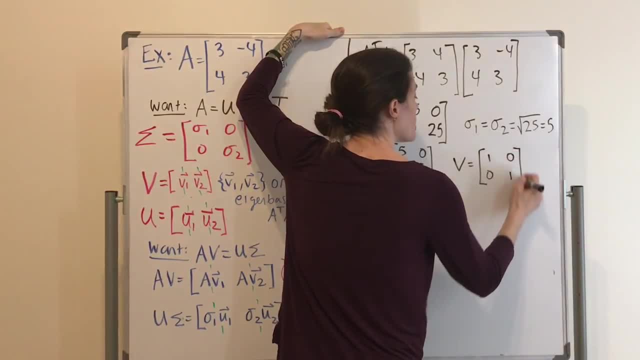 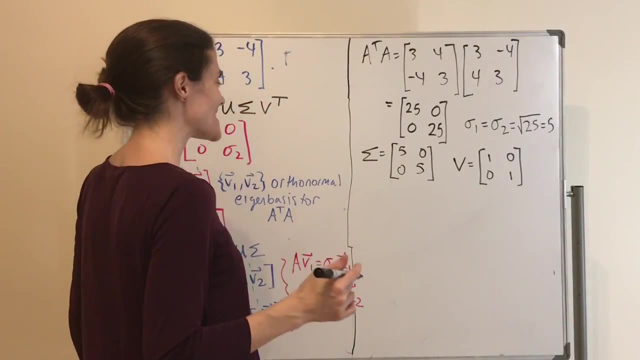 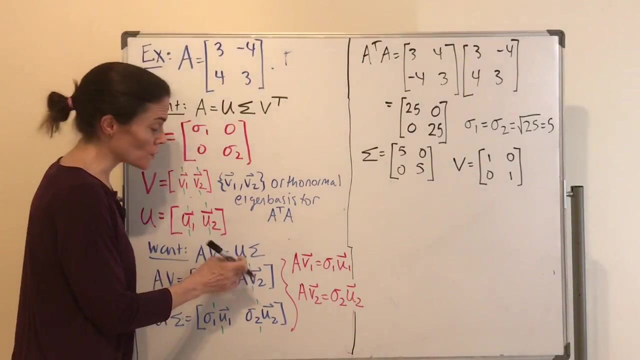 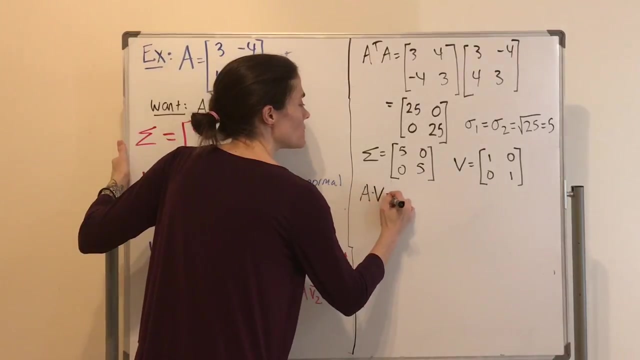 we can take these standard vectors as my orthonormal eigenbasis. Okay, this looks wonderful so far. Now, you see, the thing I left to compute is the u, And to do this I need A, a times V. well, a times V V is the identity. this is just a, which is I'll. 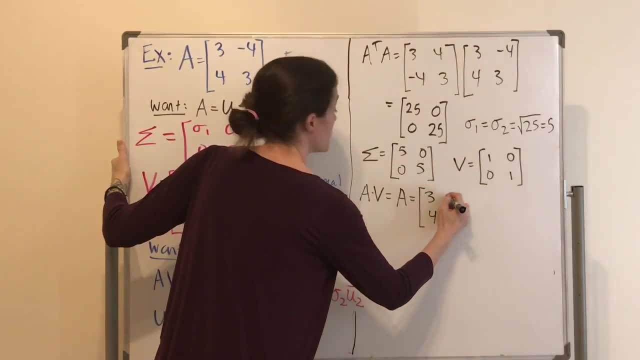 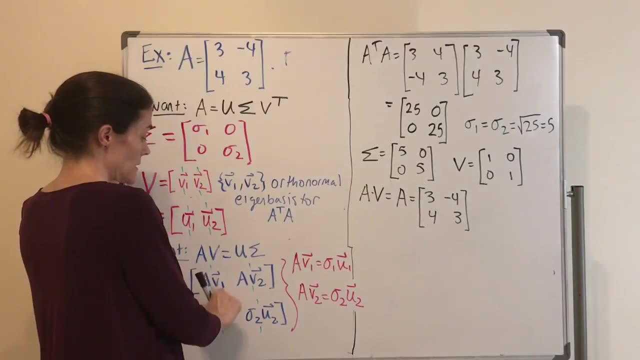 recopy 3, 4 minus, like this, and so we get right: this is a V and it's going to be equal to Sigma 1 u 1 plus, or Sigma 1 u 1, Sigma 2 u 2. so what do I get from this? 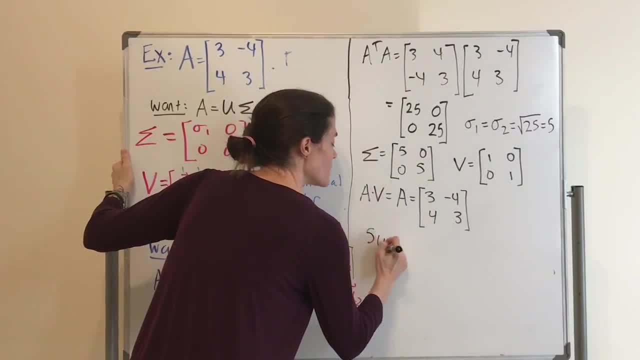 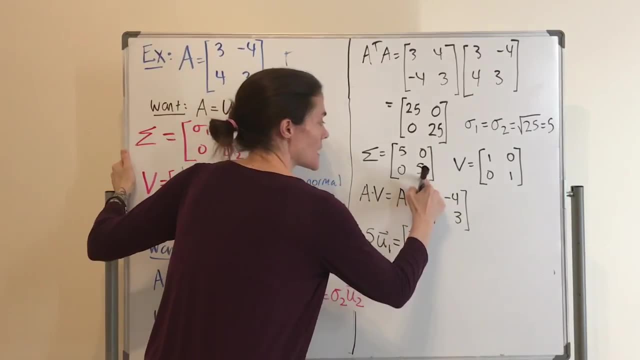 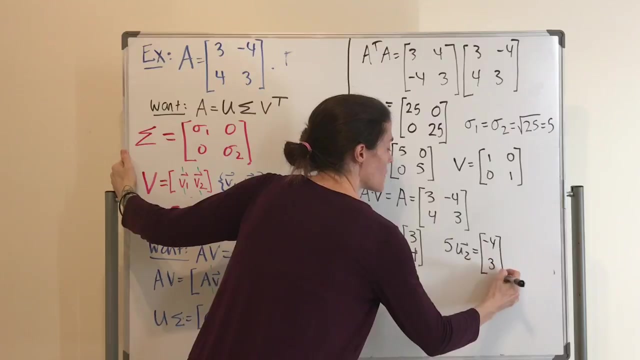 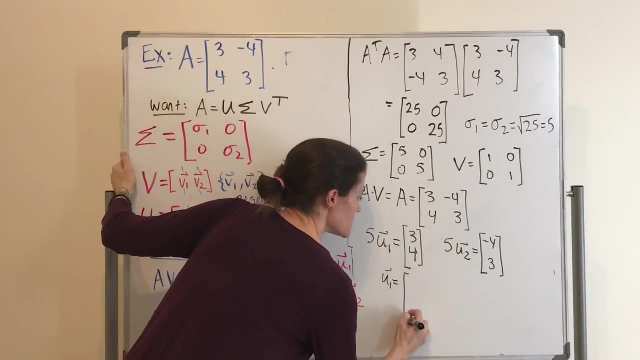 well, here is Sigma 1, Sigma 2. I get 5 u 1 equals the first column. and then I get 5 u 2 equals the second column. okay, and now I just divide. I get: u 1 is 3 over 5, 4 over 5 u 2. 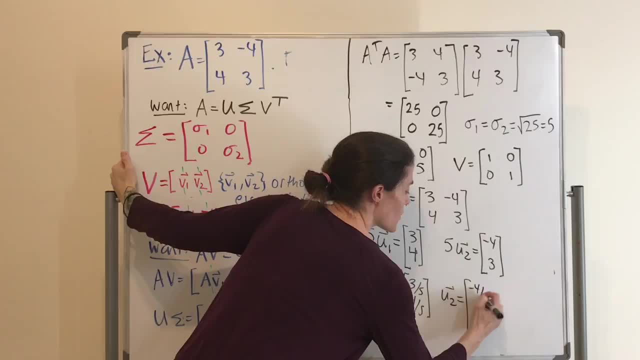 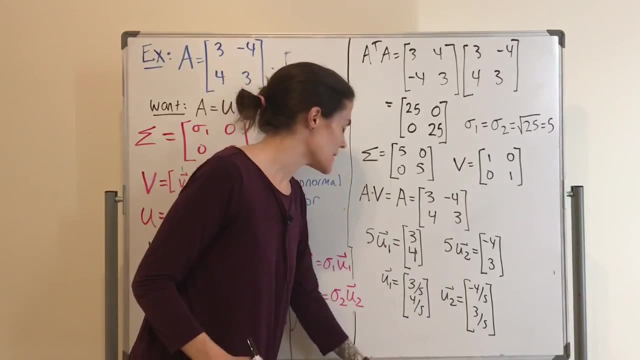 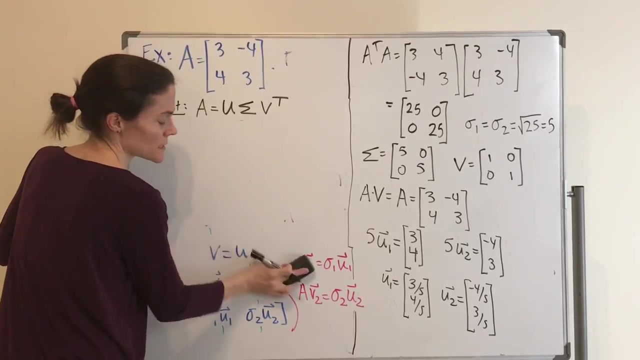 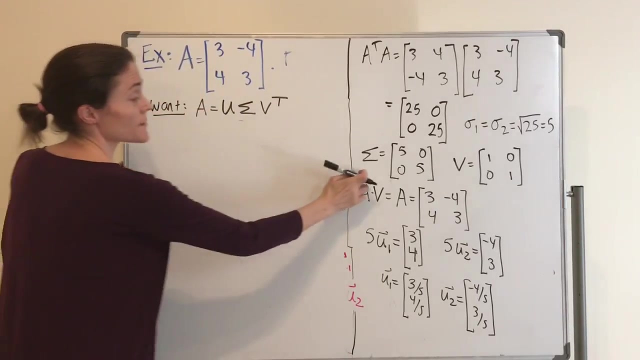 is minus 4 over 5, 3 over 5. these are the columns of my matrix view, and while we have everything here, maybe now let me just erase this- how to find- and I will write everything for this specific problem, because we have everything on the board- okay, so Sigma V, and then we have our u. 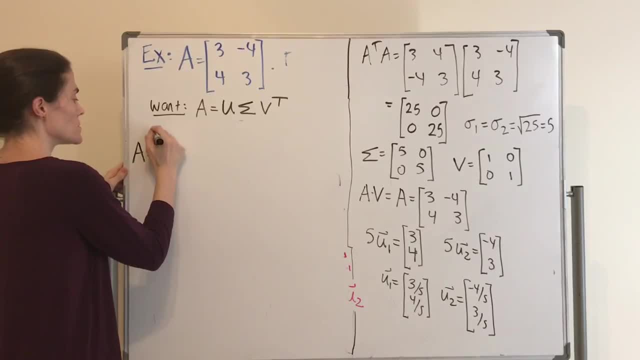 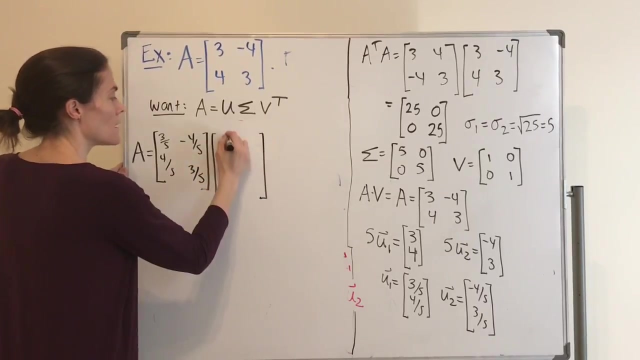 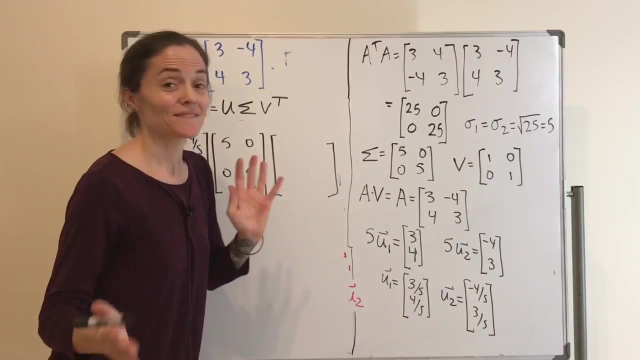 the decomposition would be a equals u, which is three-fifths, four-fifths minus four-fifths, three-fifths, and then sigma five, zero, zero, five, and then v transpose. Well, v is the identity, Transpose it's still. 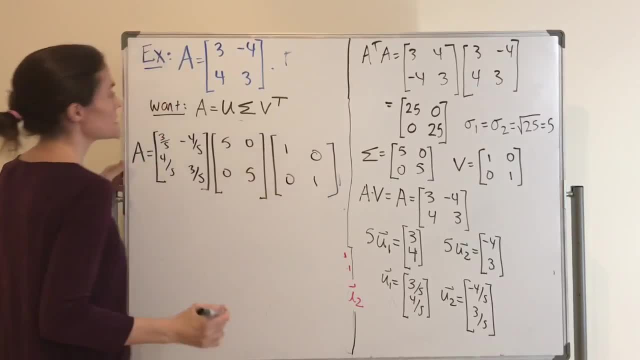 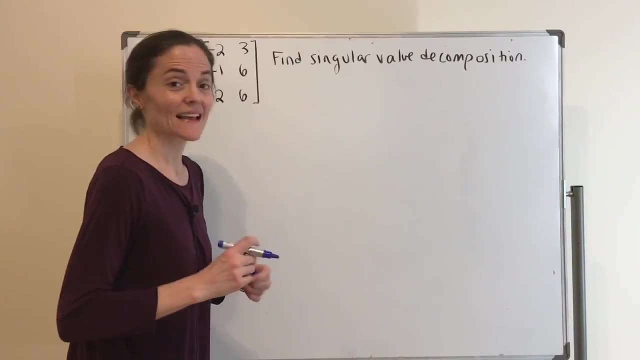 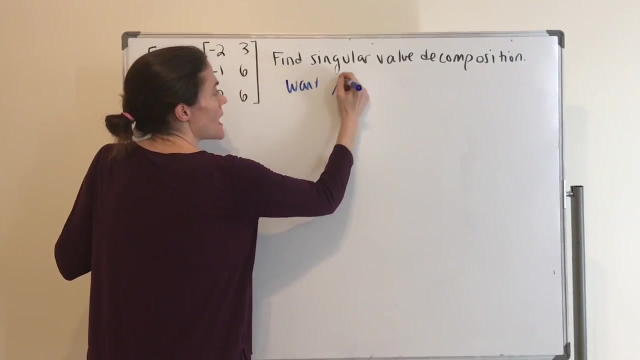 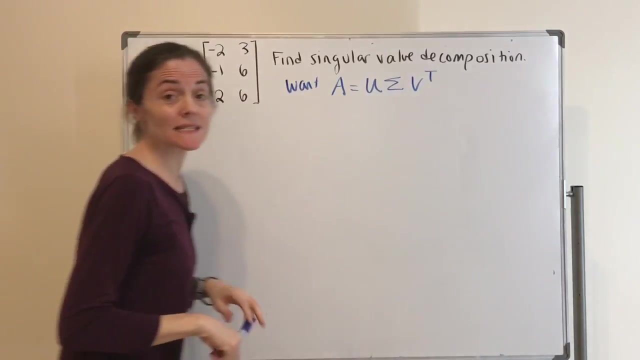 the identity. so we get this. So this is this decomposition here, our first example. Now let's do another one. Here's another example. This one is not a square, so let's write what we want here. We want a. is u sigma v, transpose, and let's write the sizes, because if you are not working with a, 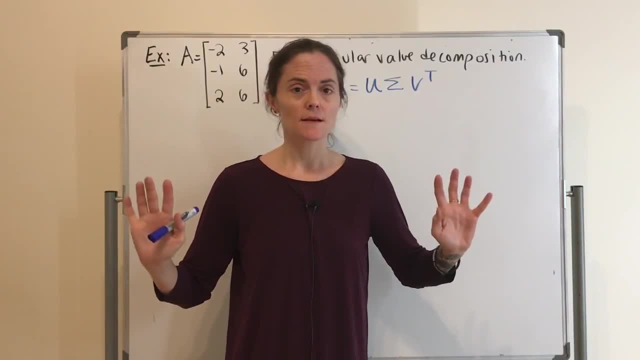 square. this is not a square. So let's write the sizes, because if you are not working with a square, this is not a square. So let's write the sizes, because if you are not working with a, you can make mistakes just by not writing down the sizes of the matrices you are looking for. 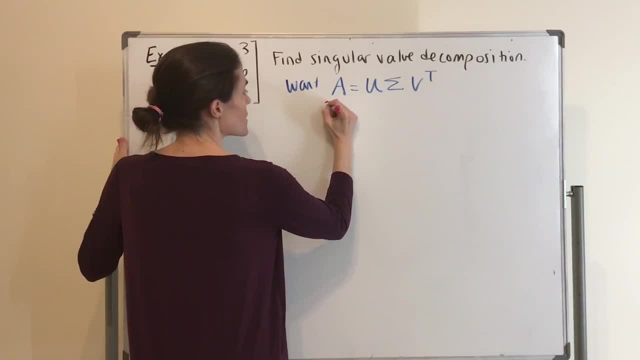 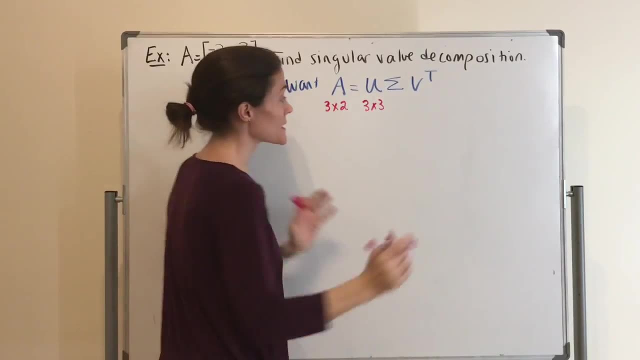 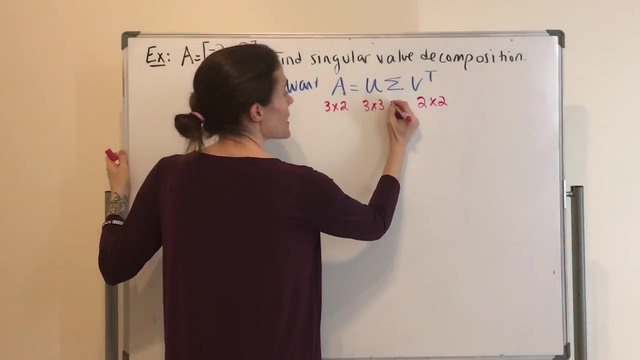 So I'm going to begin this way. This is three rows, two columns. U will be three by three. orthogonal matrix- This has to be two by two. orthogonal matrix- That means sigma, just to make this product defined will be three by two. 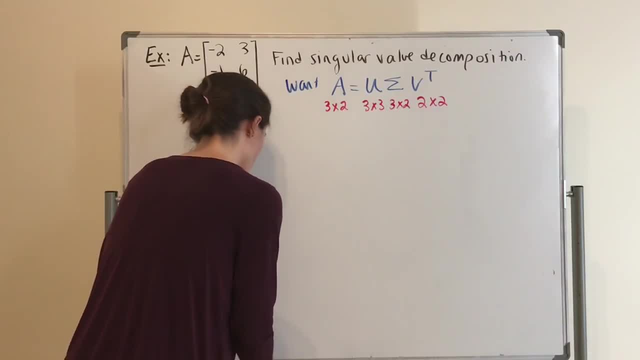 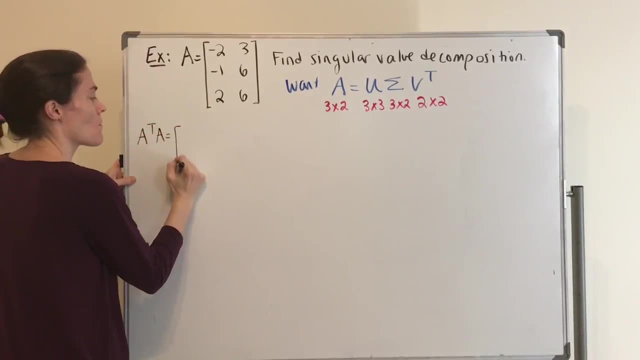 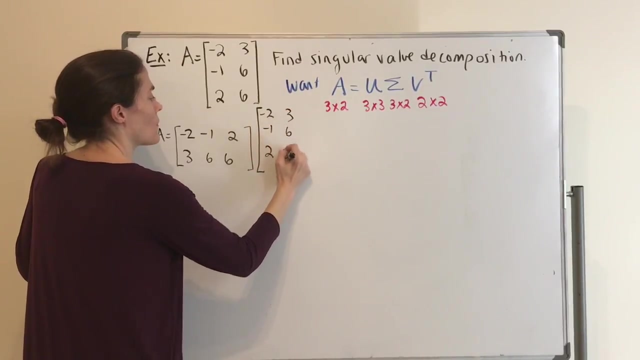 Three rows, two columns, Okay, wonderful. Now let's get started. Step number one: we must compute a, transpose, a. Okay, this is minus two, minus one, two, three, six, six. Well, let's think about the size. Two by three, three by two, this will be. 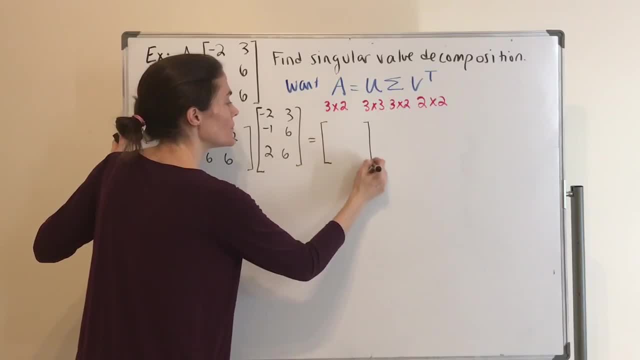 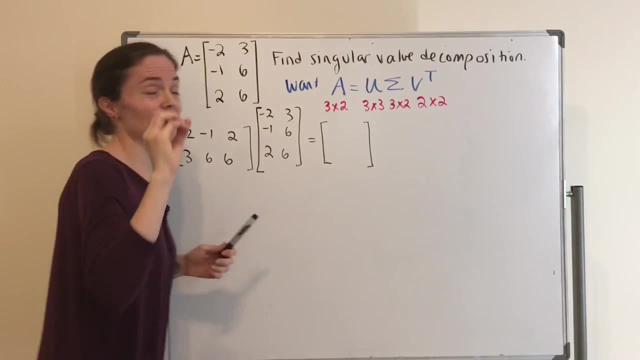 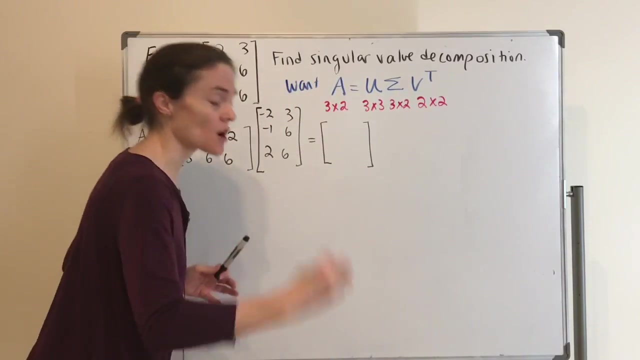 two by two, In fact, we will have two singular values for a And well, this will always be the case. Remember I mentioned, if you're in by m, that's the number of columns. we will have m singular values And the first r, which is the rank, will be non-zero, like this, Okay. 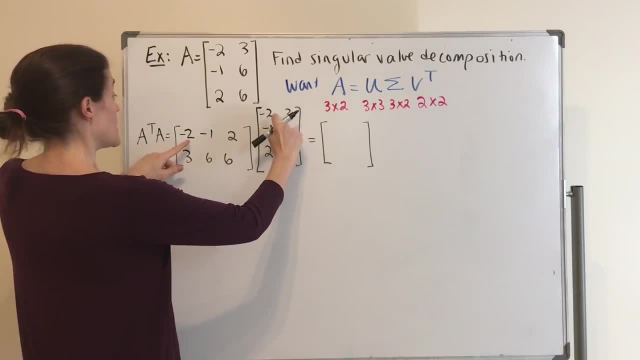 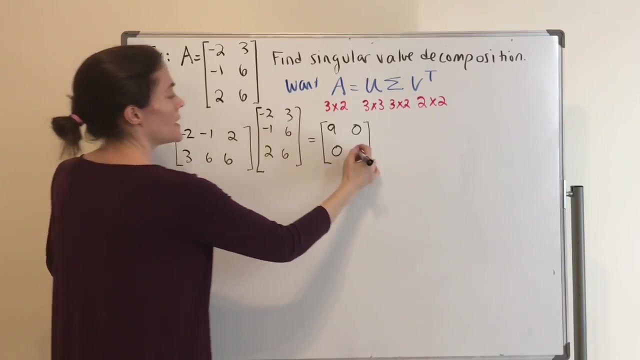 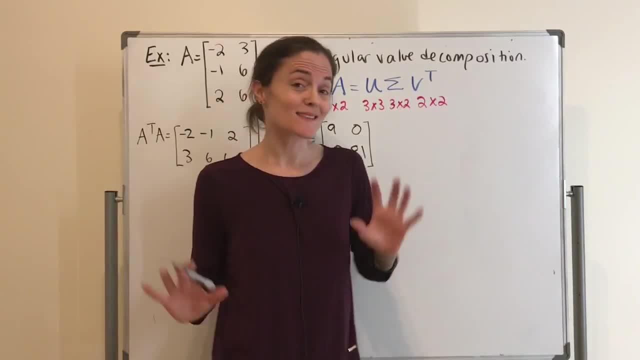 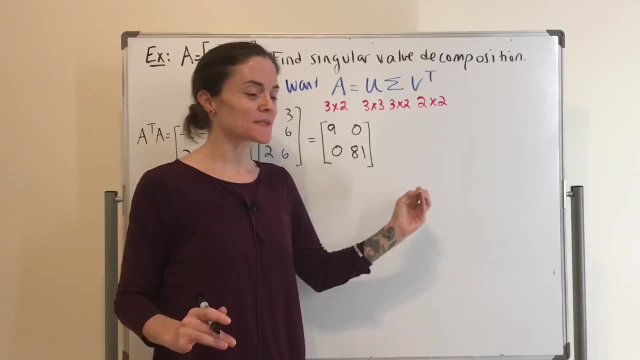 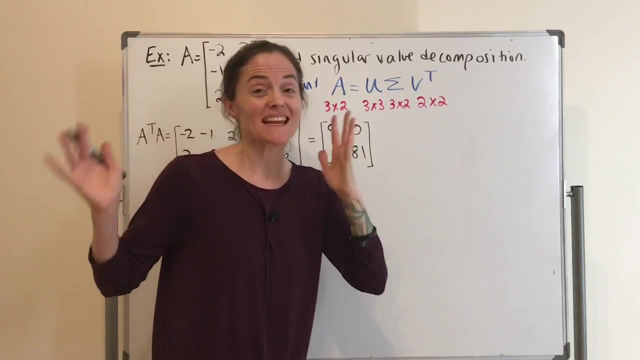 diagonal. It's definitely not the case that a transpose a is always diagonal, but I'm trying to illustrate calculating u, Sigma and v transpose And so making examples where, for instance, finding the eigenvalues and even associated eigenvectors is well straightforward for a diagonal matrix. 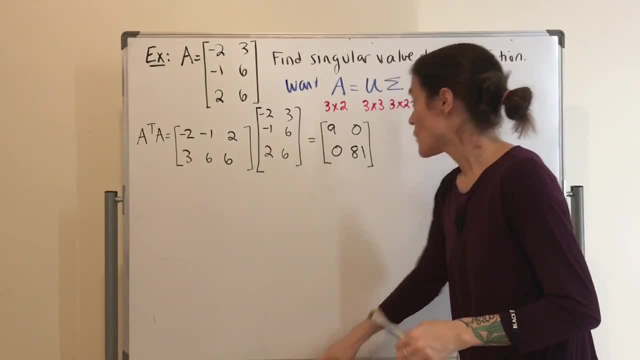 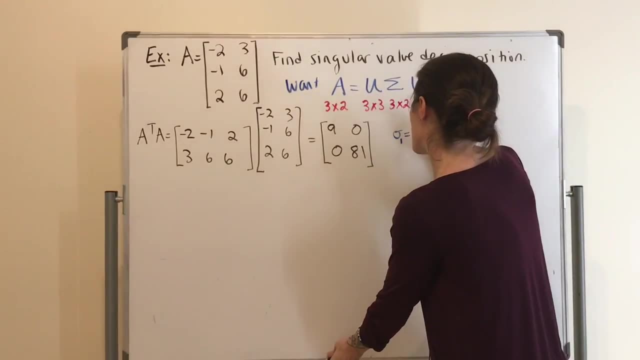 Okay, What do we see here? Sigma one is the square root of 81,, which is nine. You always take the biggest one as sigma one, And then sigma 2 is computing the square root of 9,, which is three. 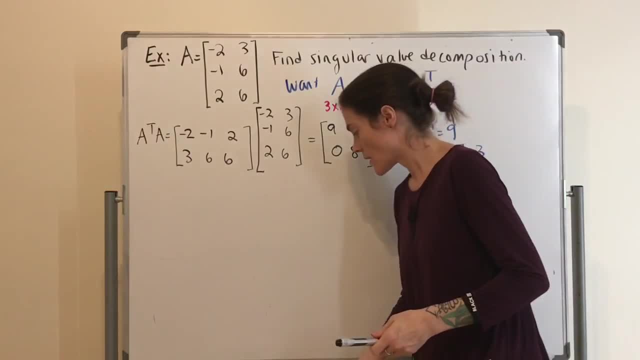 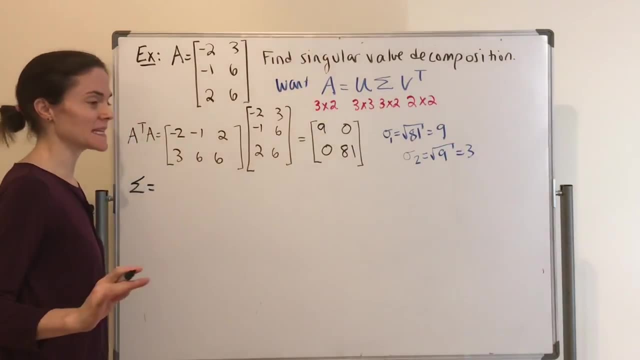 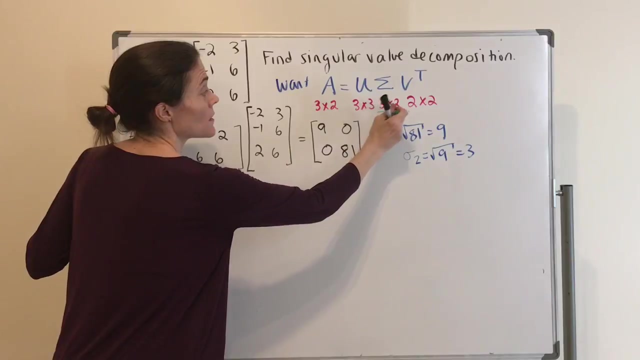 So my matrix, sigma, I know it already- Sigma we will put here. Here's the first time. we have to be careful And we didn't see this in the last example, and that's here. Look, Sigma is three rows. 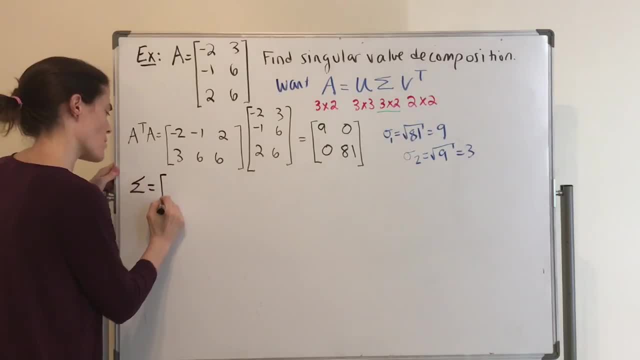 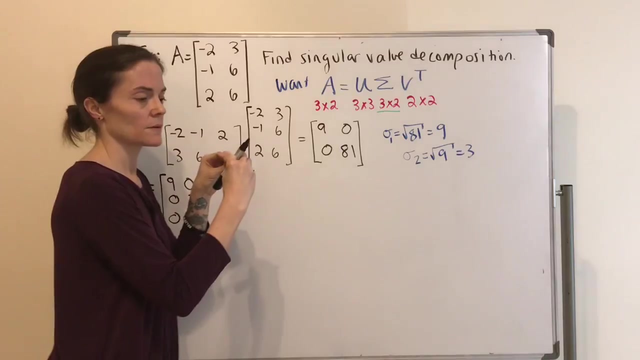 two columns, zeros, two columns, and it will have the biggest singular value here and the next biggest here, and these are the only singular values. then, if you remember, this must be okay. zeros, because the only non-zero entries in sigma are the, the first r singular values, where r is the rank of a like. 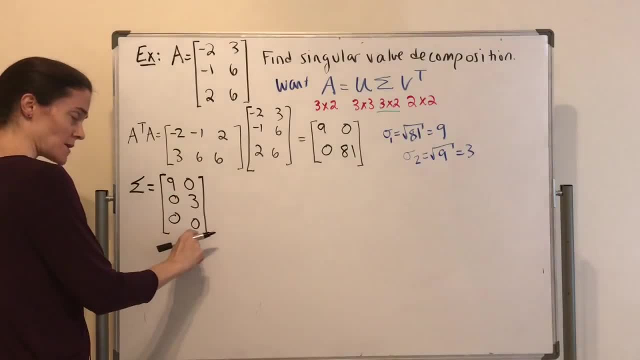 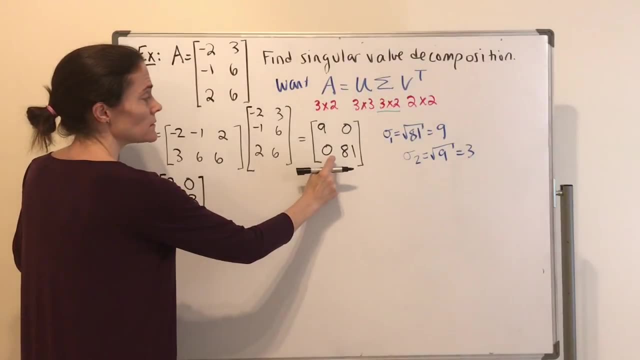 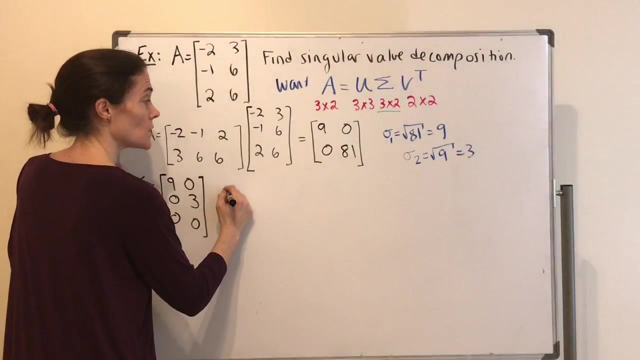 this. we have them here. everything else must be zero. so i know this last row is zeros. okay, then, if i want to get eigenvectors corresponding to each of these, i can easily just take um, v1 to be um, that would correspond to this and v2. 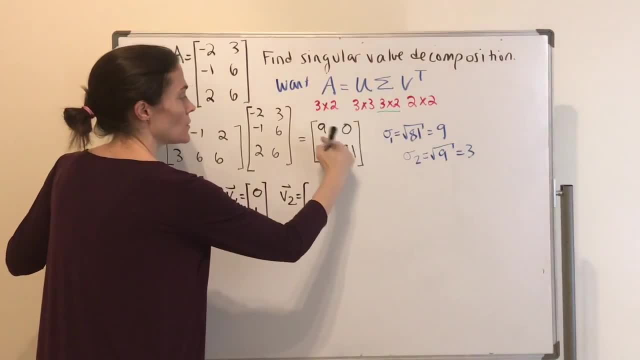 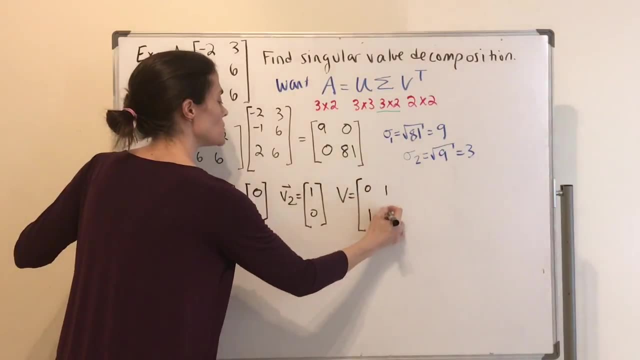 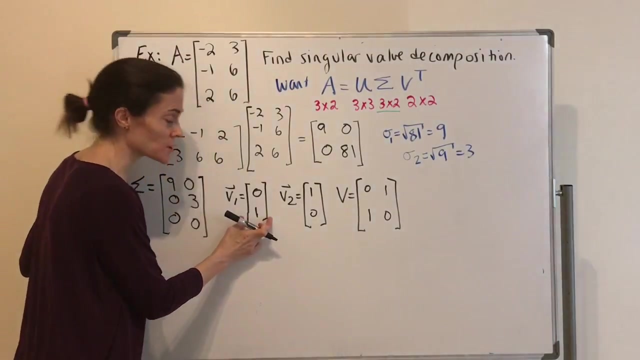 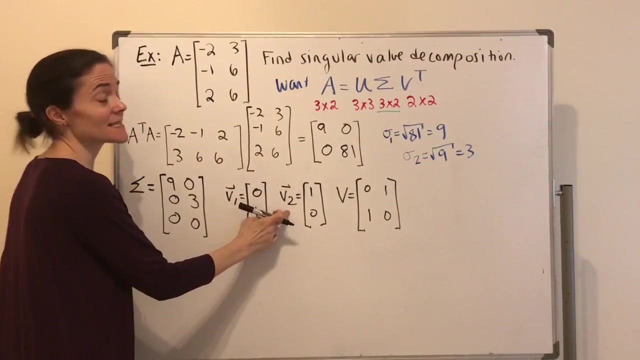 um and v2 and v2. this would correspond to to this one like this. so my matrix v is v1, v2. okay, and the order matters. okay. this eigenvector is a unit eigenvector corresponding to lambda equals 81 or corresponding to this singular value, and this is an eigenvector corresponding. 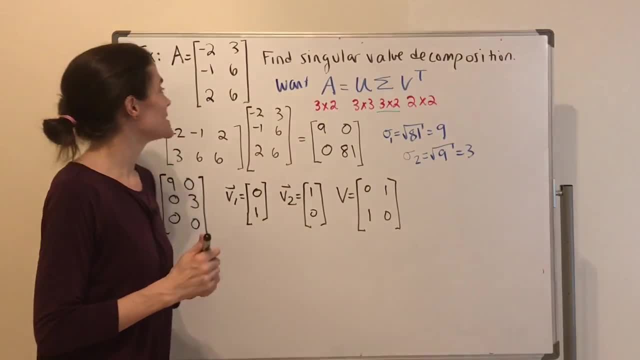 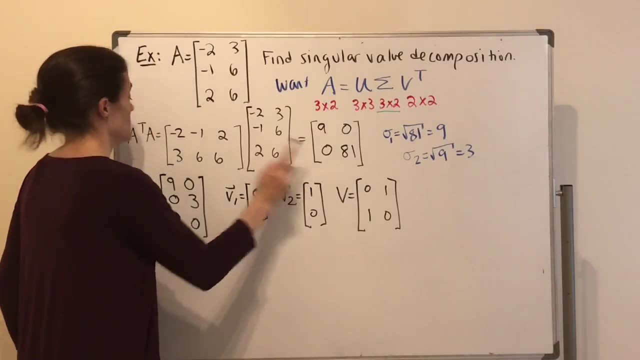 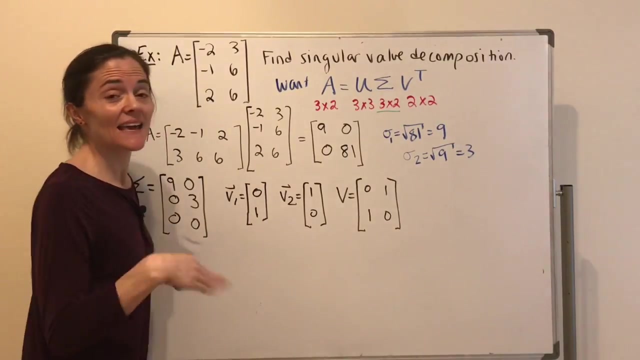 to lambda equals nine. and another comment that i'll make, which is important, and notice: v1, v2, eigenvectors for a transpose a here. okay, i made my board shake, i got a little excited there. they are not eigenvectors for a because, well, even though a v1 is, without a doubt, 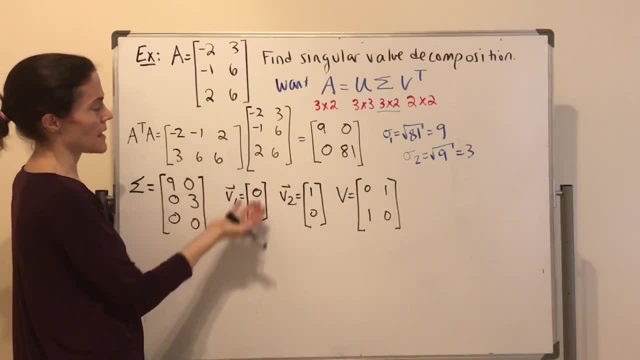 defined here. right, you can multiply a times v1. the problem is it's a vector in r3, so this is not an i v1, so this is not an i v2. so this is not a vector in r3, so this is not an i v1. so this is not an i v1. 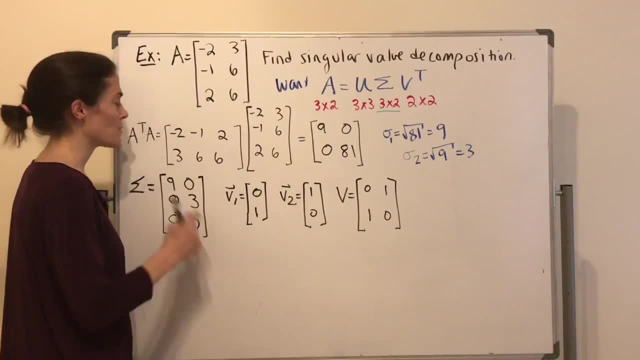 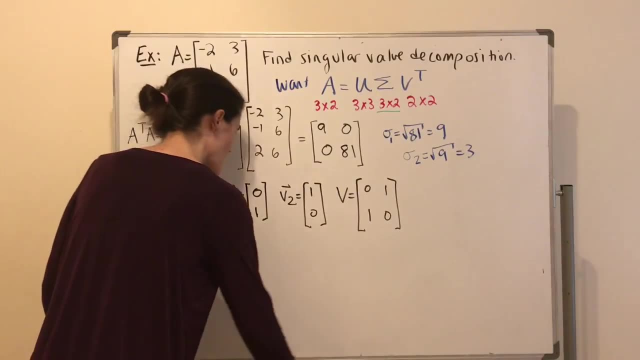 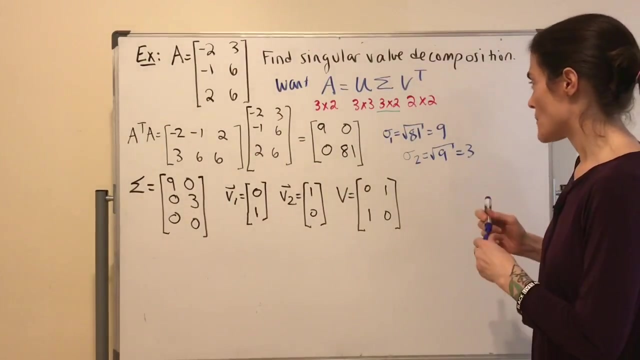 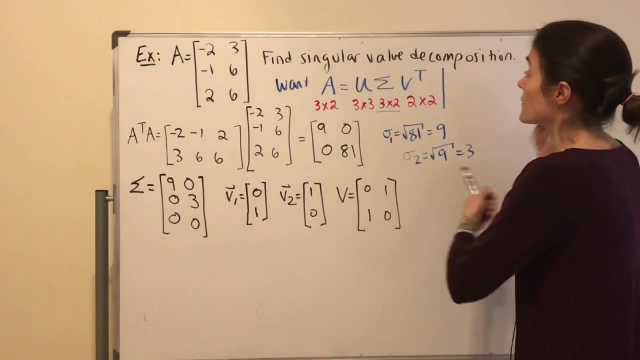 vector for a. neither one of them is okay. just remember that they're eigenvectors for a. transpose a. okay, we have sigma. we have v. very nice, i need over here to compute a v and then i can find my matrix u. so maybe i will even rewrite this here. i will do it in brown. it was a v equals u sigma. 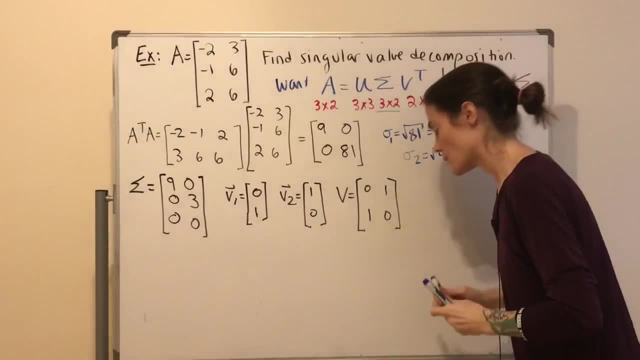 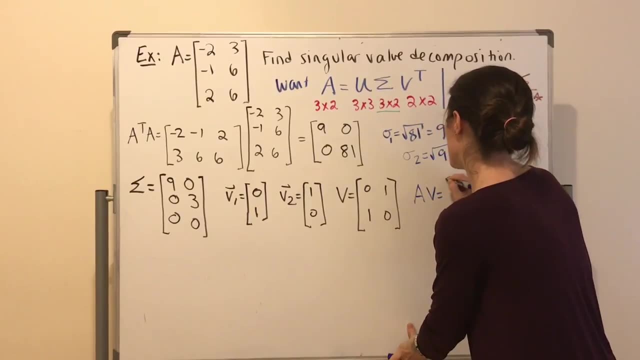 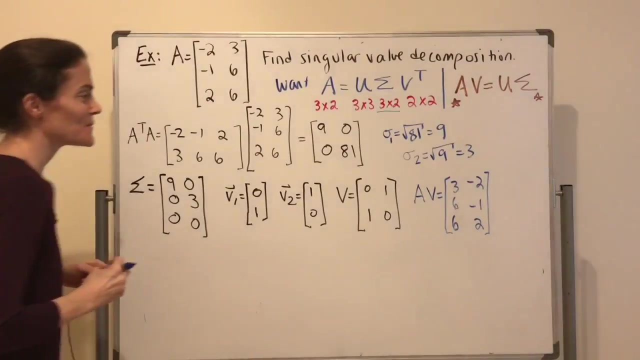 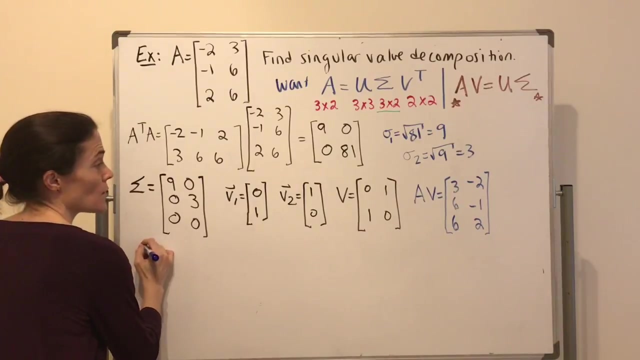 this is what i use to find u right. so if i multiply- and this is not very hard- with this a and this v, you'll notice this just interchanges the columns. okay, so now i can find u1 and u2. okay, so i will. i know that sigma one, nine, u1, will equal. 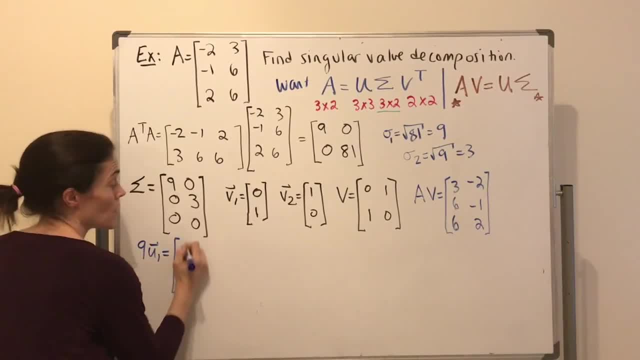 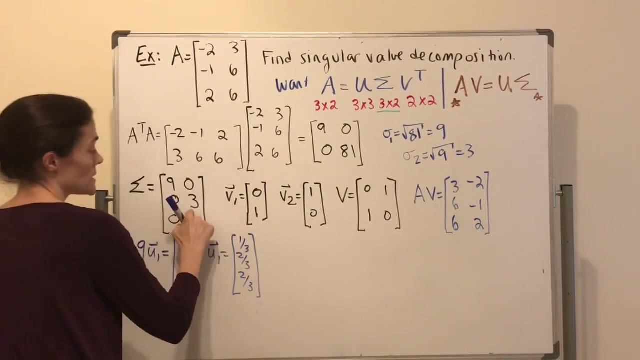 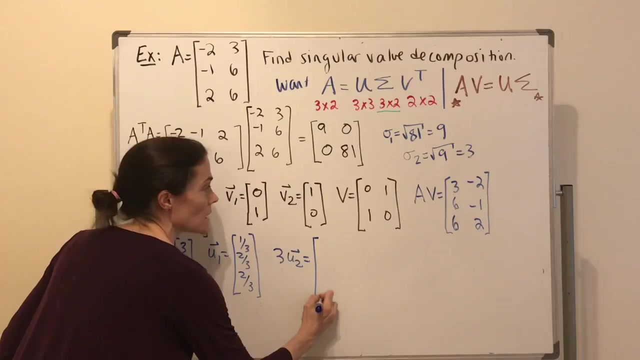 three, six, six. this is that sigma one. u1 is equal to three six six a b one, and so u1 equals um one third, two thirds, two thirds. and then i can use this: three u2 equals the second column of a times v minus two. minus one, two. 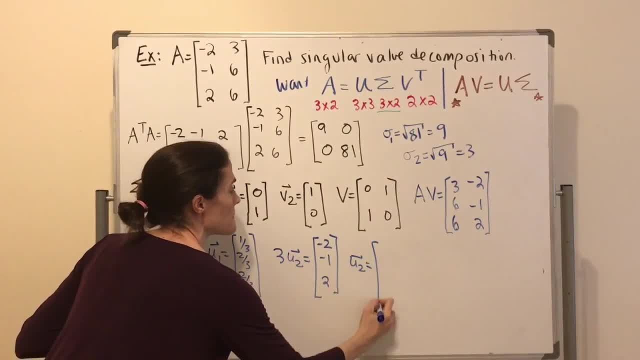 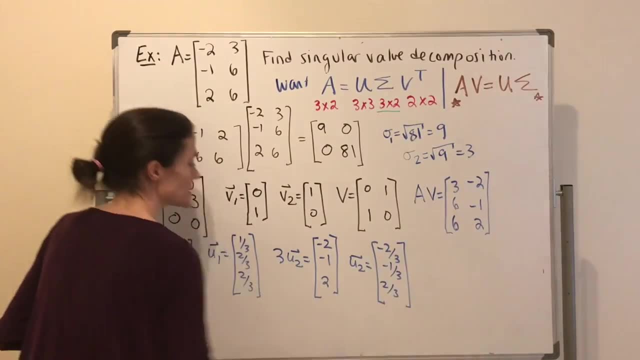 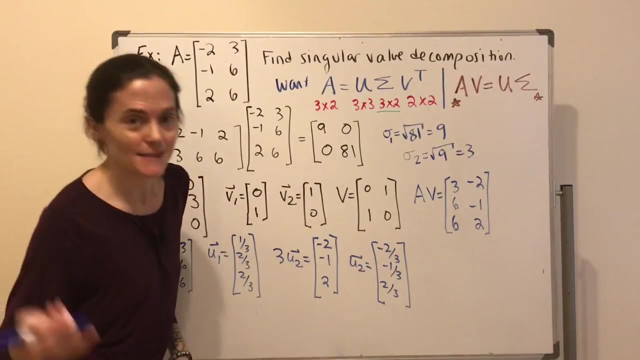 and i get that u2 is minus two over three, minus one over three and two over three. in fact, take their first of all. u1 and u2 are unit. second of all, take their dot product zero. so these two, u1- u2, are orthonormal vectors. now you might be thinking: 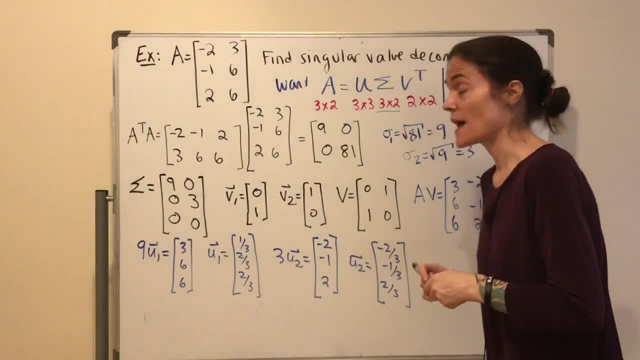 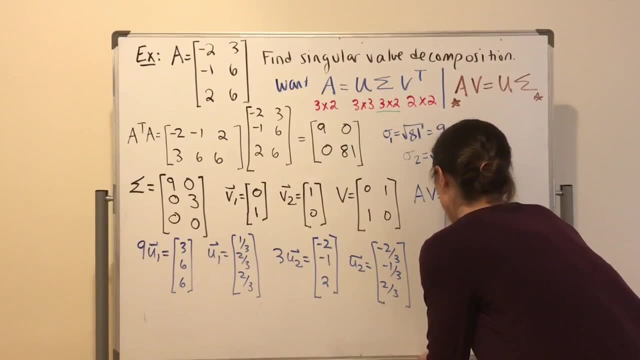 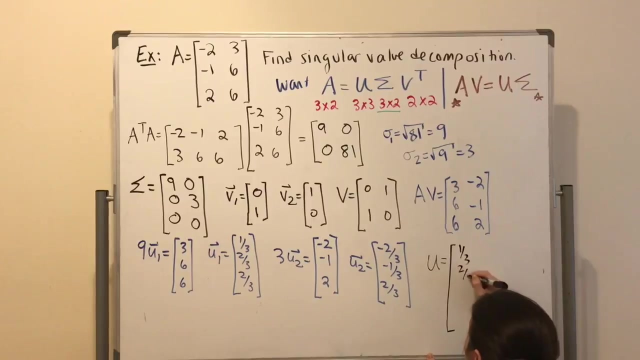 uh, oh, because we don't have any more singular values to work with. okay, so so far, what do we have here? we know, We know U is. Let's write what we have. It's going to be 1- 3rd, 2 3rds and 2- 3rds, And 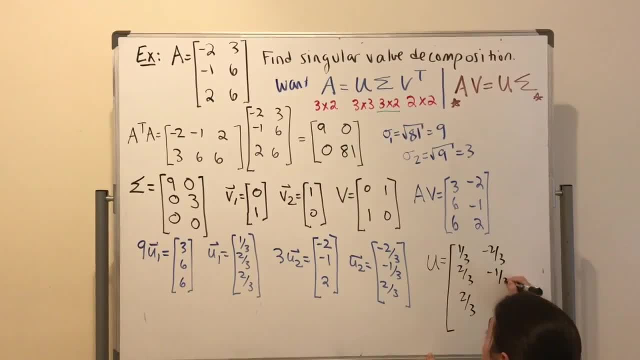 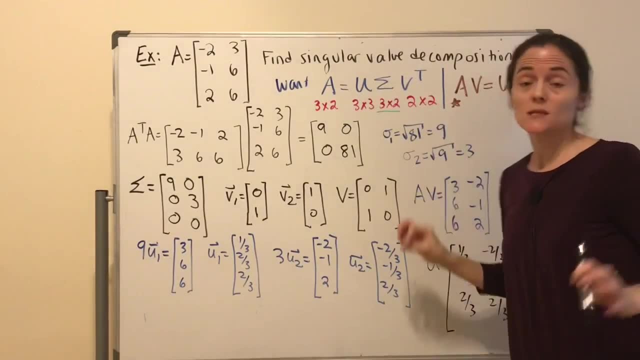 minus 2 3rds, minus 1 3rd and 2 3rds. But the problem is- and this is where I said we really want to write the sizes when we start so that we don't make a mistake. Problem is, this is not U. 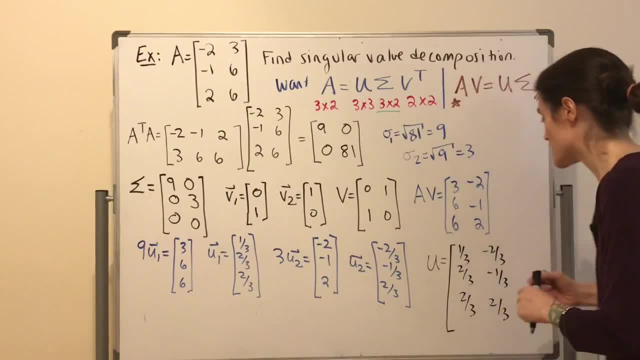 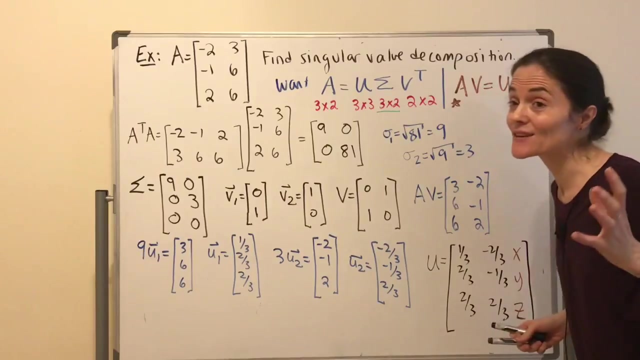 because U is 3 by 3. And so it's going to be something. It's going to be some x, y and z, But uh-oh, the cap came off. Let me close this matrix. Well, there's no singular value of a. that's going to help me find x, y, z. okay, If you might think. 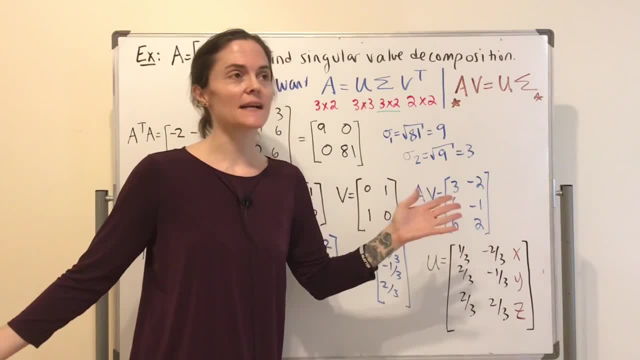 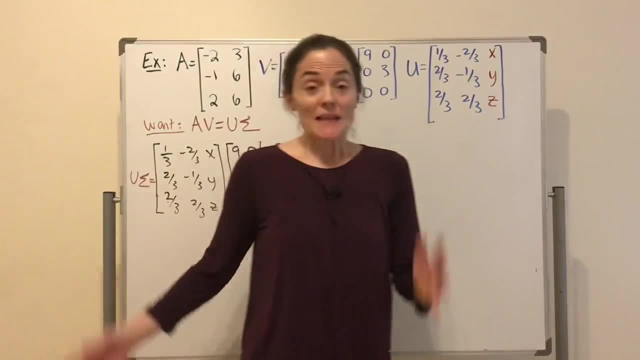 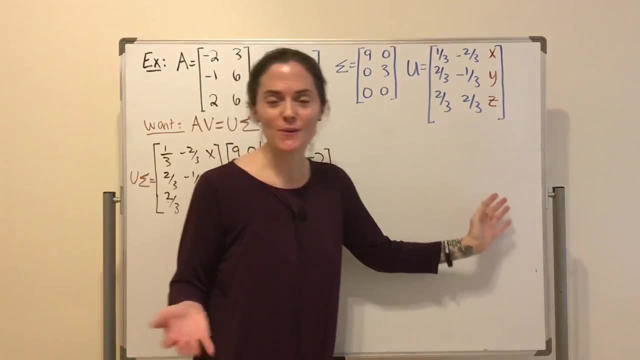 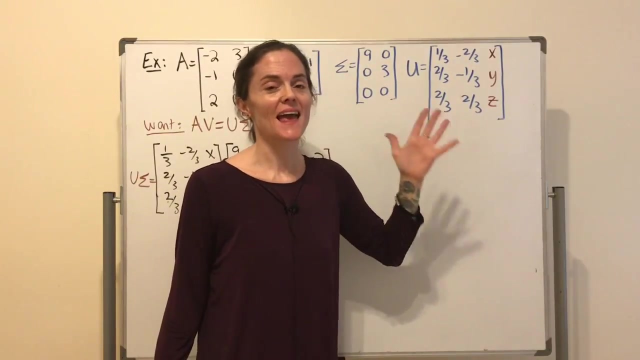 that we need to talk about. Well, I have erased and I kept v, which I need, sigma, which I need, and U, which I don't quite have yet. right, Because we want U to have numbers, And right now. 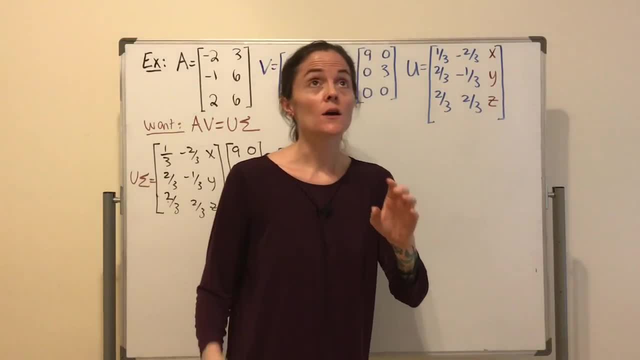 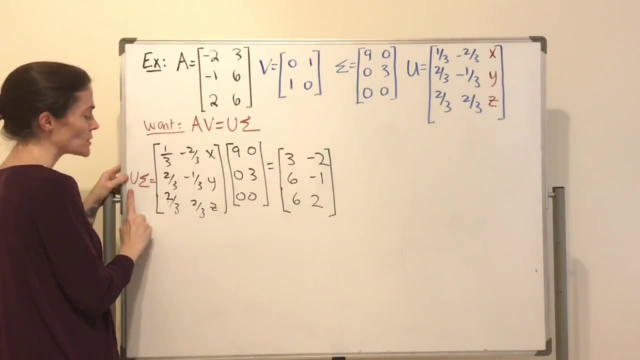 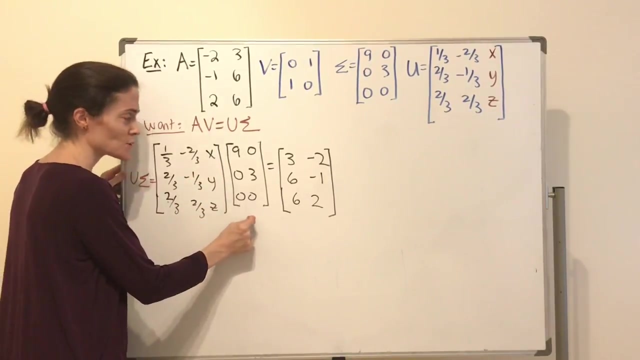 it has x, y and z. But how we're finding U is A, v is U sigma. And you notice, if I multiply U times sigma with any numbers, x, y, z. well, this matrix times this matrix, it's not that hard to multiply. We only have two. 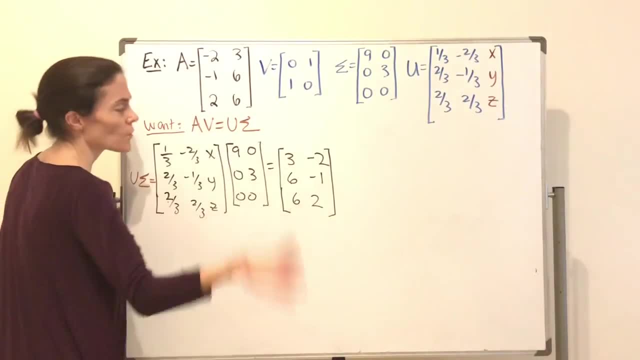 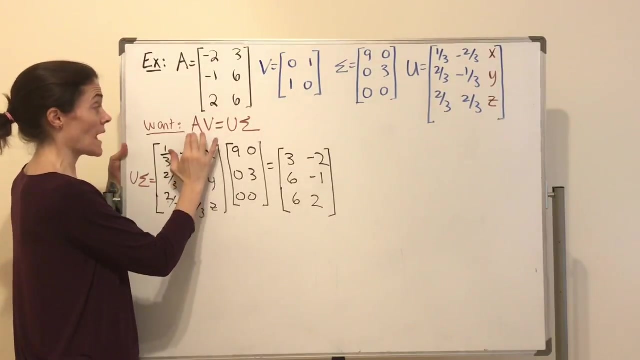 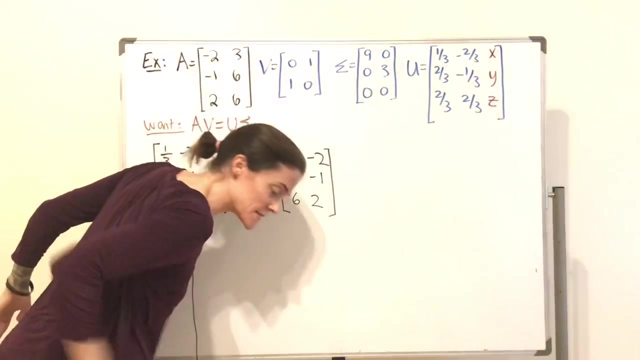 non-zero entries. We get this, Of course we should know. we get this just by multiplying A times v. But my point here is: no matter what x, y, z is, we get that A v will be U sigma, just because sigma has this row of zeros at the bottom. 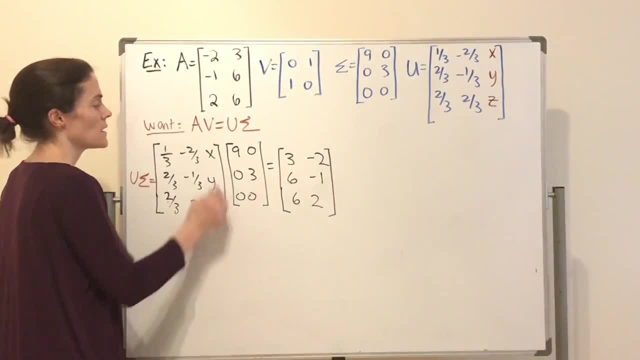 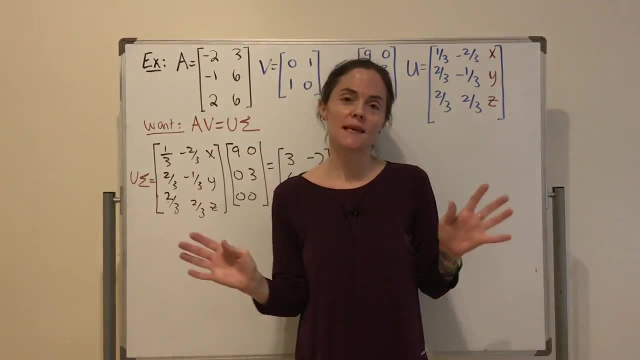 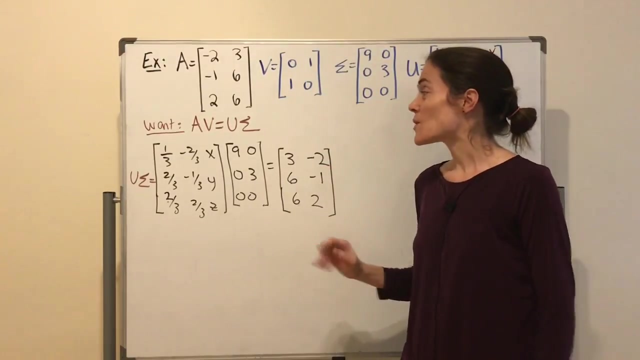 So this product will be equal to this, no matter what x, y and z are. Okay. so x, y, z, this vector does not come from the singular values. But what does it come from? Well, what do we know? 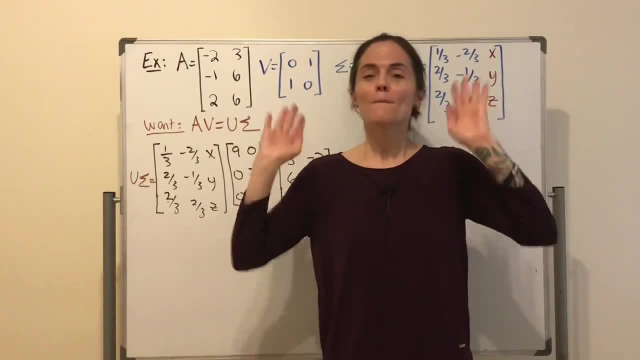 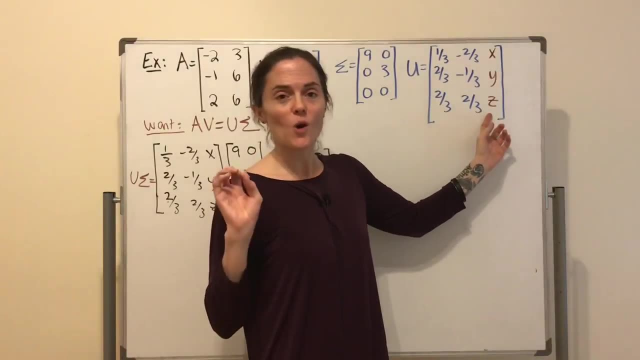 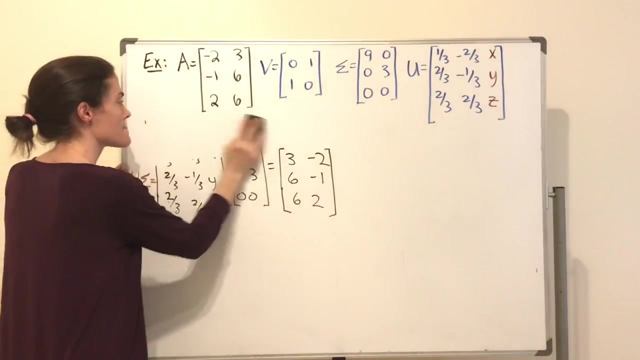 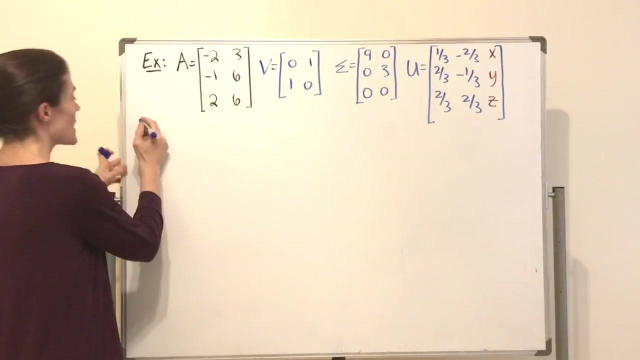 about U. What must be true about U? Orthogonal matrix, which means the column. So this column, this column and this column are orthonormal vectors. Okay, now let me erase this here. So how are we going to find x, y, z? So we can find U three times sigma, which means: 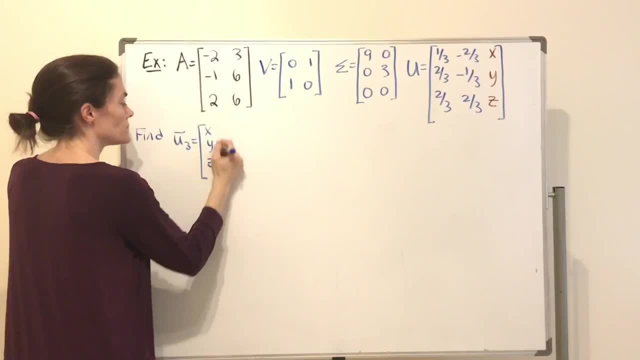 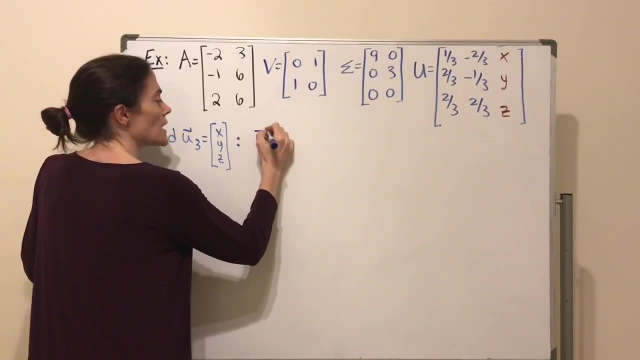 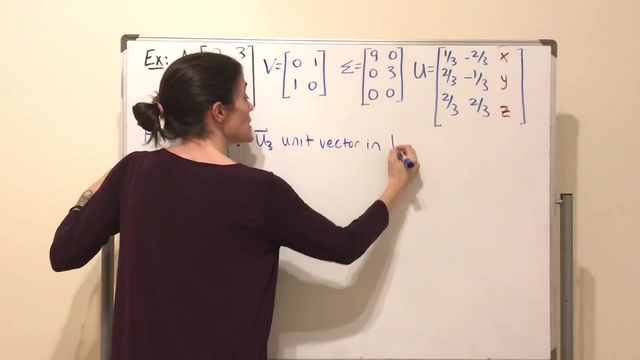 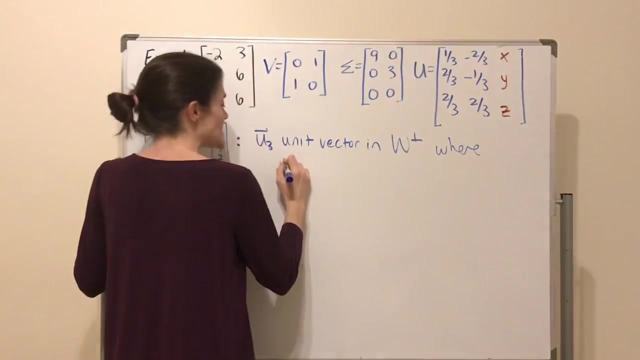 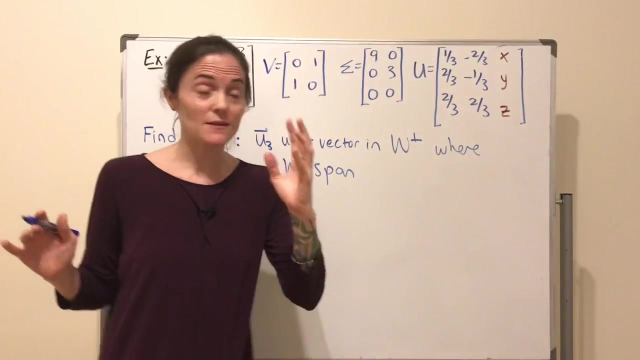 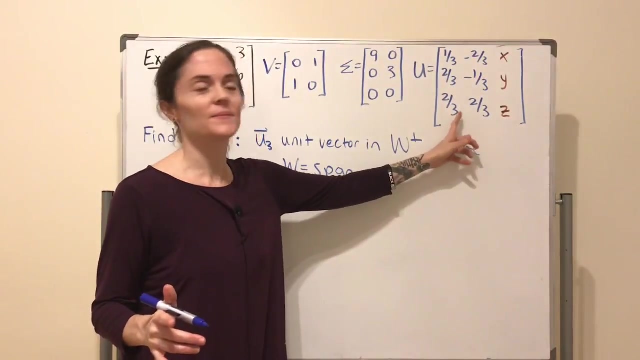 x, y, z as I have called it in this matrix. We want u3 to be unit vector in the orthogonal complement of w, where w is the span of the first two columns. This will make u3 unit okay And it's going to make it perpendicular to this column and this column. 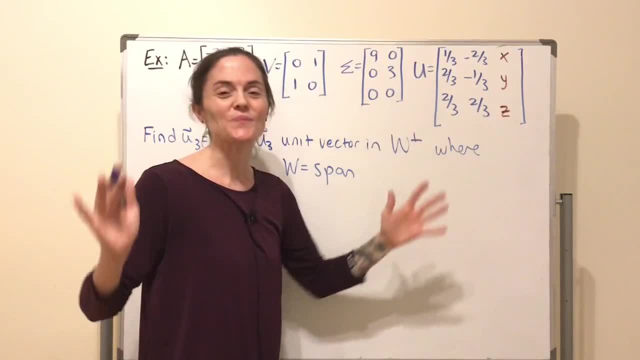 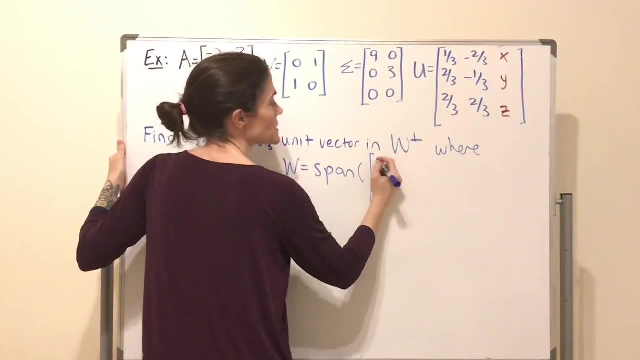 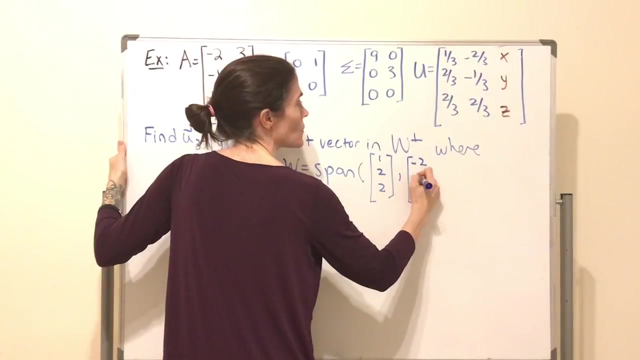 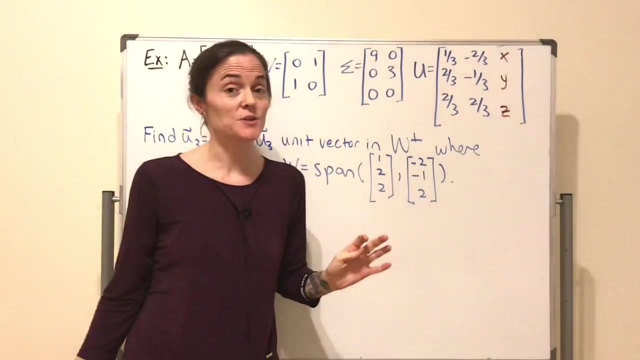 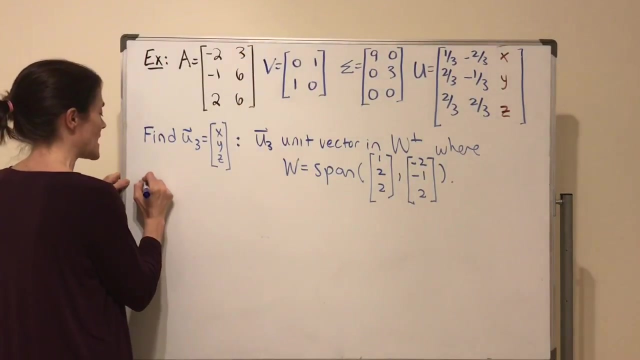 so that the matrix u is an orthogonal matrix. So where w is the span? maybe I will just list them without dividing by by 3.. And how do I find a unit vector in an orthogonal complement? Okay, well, we can. let's restate. 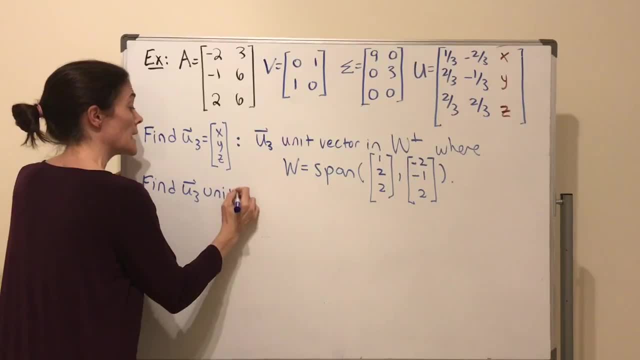 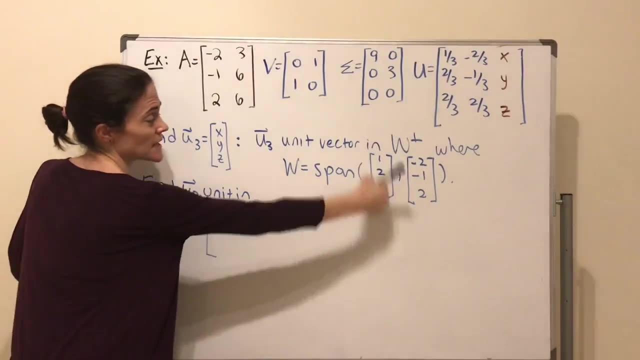 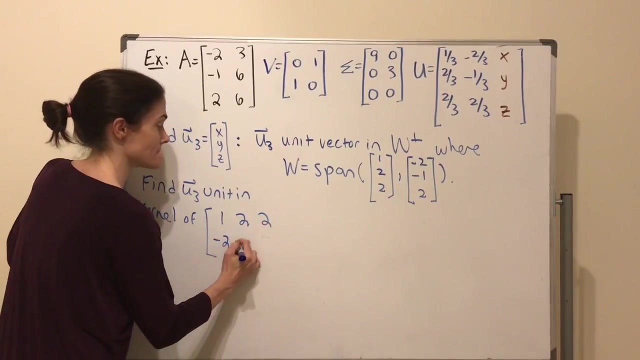 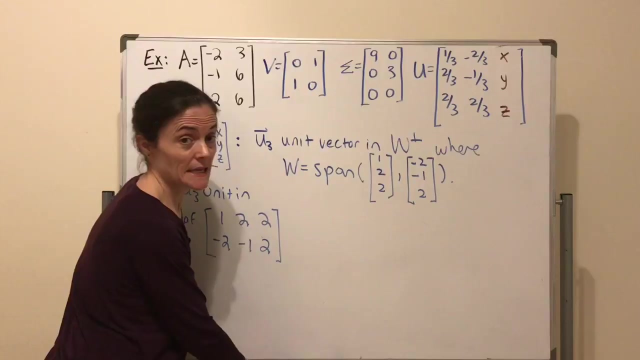 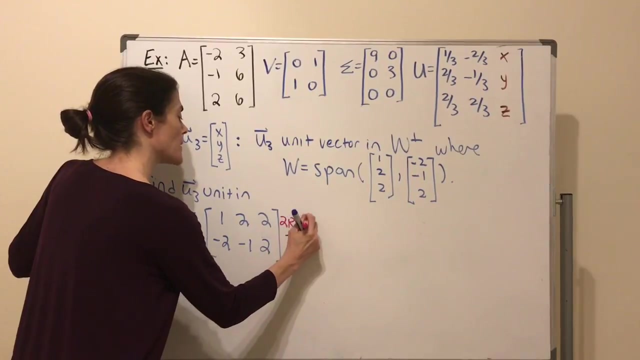 find u3 unit in the kernel of this matrix where we put these vectors as the rows. This is something we have practiced, Okay. so now let's perform some row operations to get this in reduced row echelon form. The first thing I will do is I will take 2 row 1, add it to row 2.. 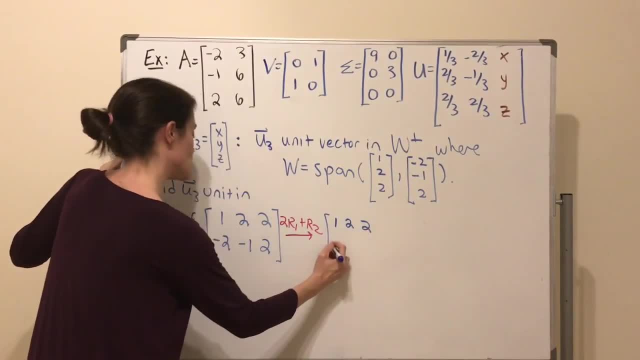 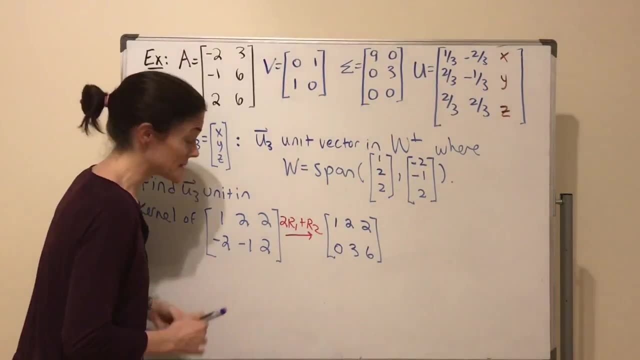 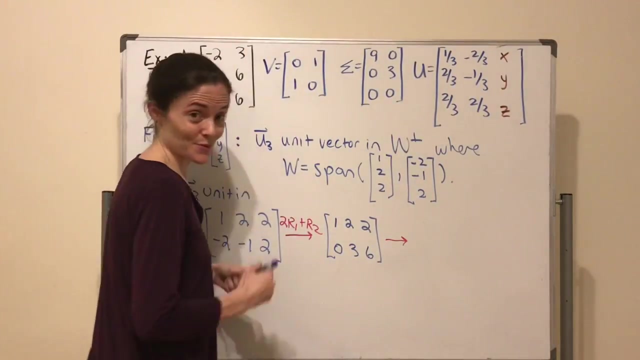 Row 1 stays the same, row 2 is now 0,, 3, and 6.. And maybe I will do 2 steps at once here. The first thing I will do is divide row 2 by 3,, 0,, 1,, 2.. 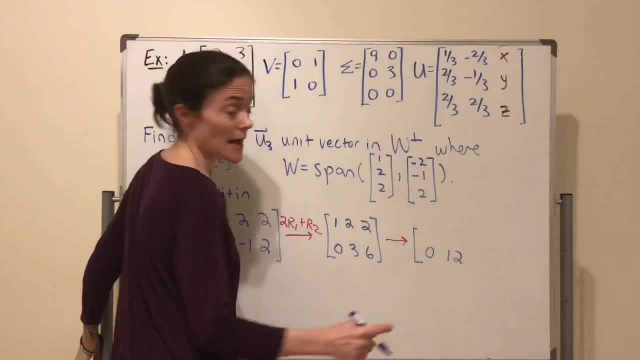 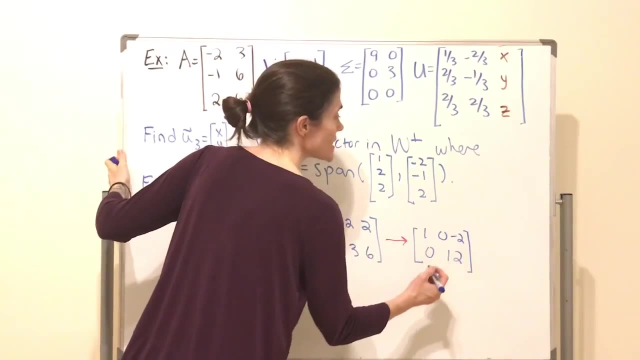 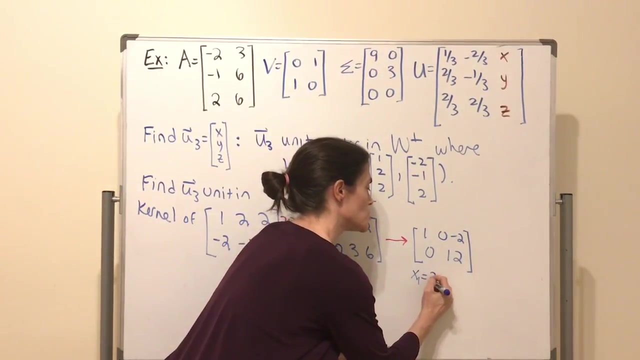 And then I will take minus 2 times this, add it to the first row. What do we see from here? We see x3 is free. We see x1 is 2x3.. We see x2 is negative 2x3.. 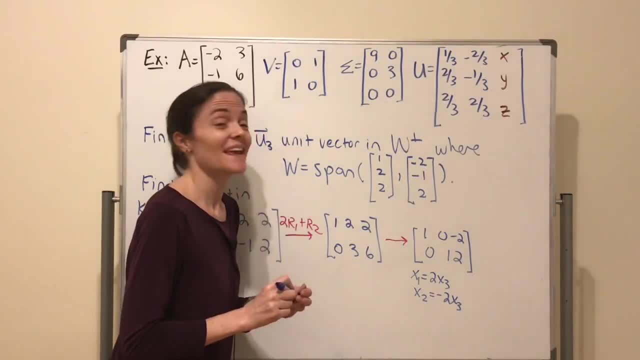 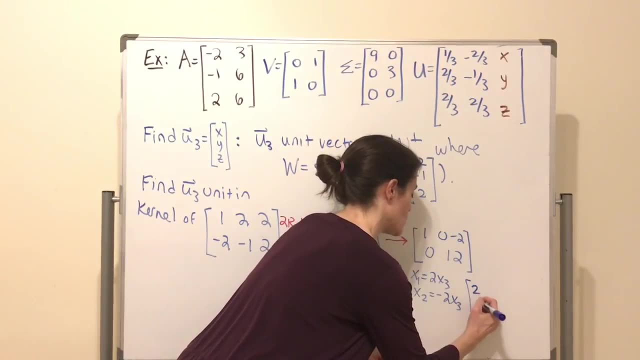 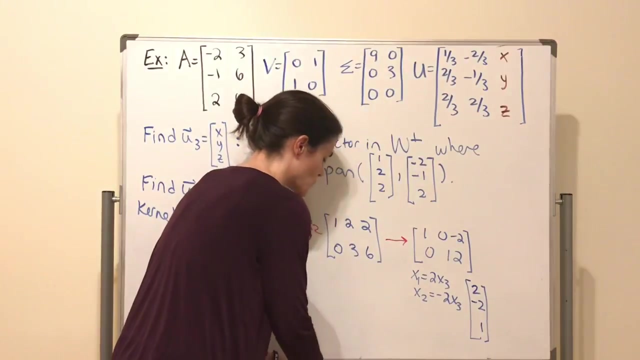 So one non-zero vector in the kernel would be. well, I could put a 1 here, a 2, a minus 2.. It's not units. So to get a unit vector in the kernel, which is what I really need to fill out my matrix. 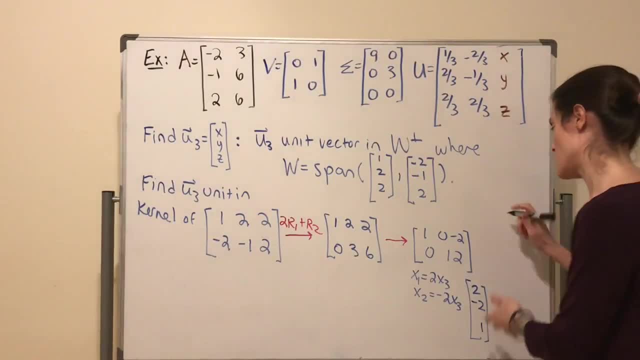 u and make it an orthogonal matrix. maybe I will write that here. I just divide by the length. The length here. well, we have 4,, 4, 1, square root of 9, 3 is the length of this vector. 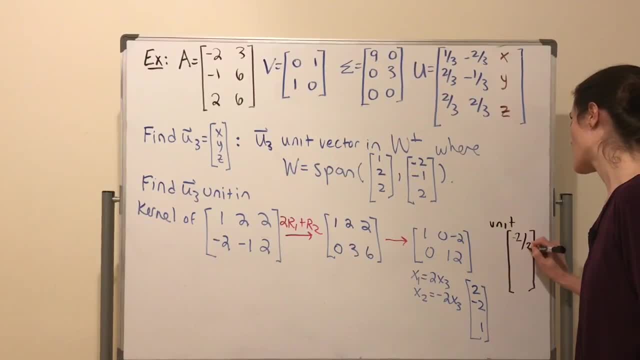 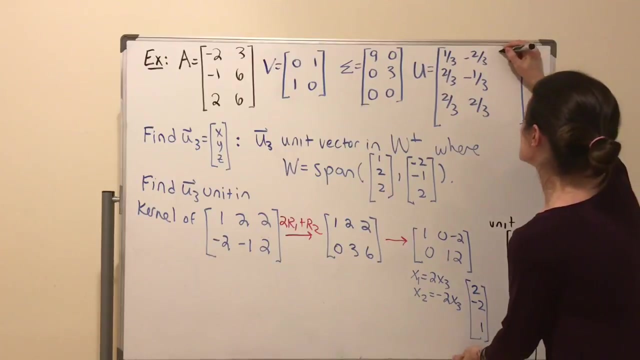 So we have uh-oh, 2 over 3, negative, 2 over 3.. Okay, Let's put it here: 2 over 3, negative, 2 over 3,, 1 over 3.. Let's put it here: 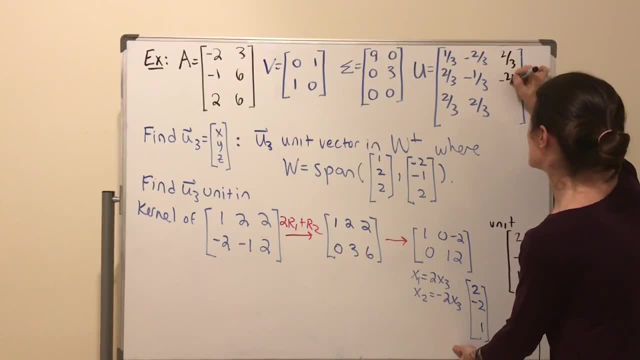 2 over 3, negative 2 over 3, 1 over 3.. Okay, So my matrix u is orthogonal, And well, we would have u. sigma is a v. But now let's do something. Let's see, I'll erase this and we will write out the singular value: decomposition. 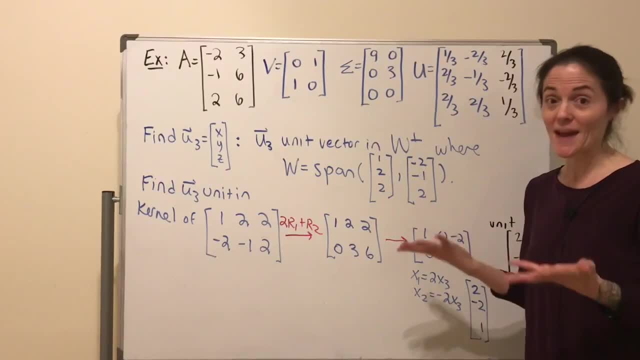 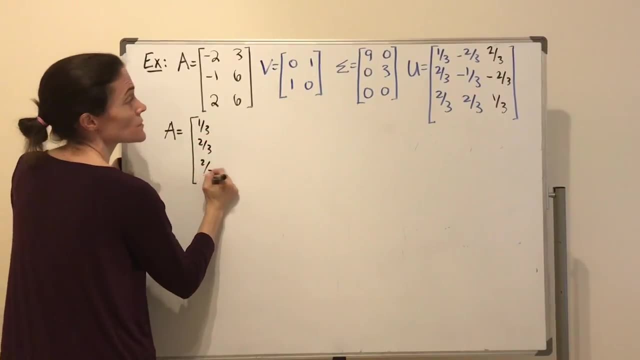 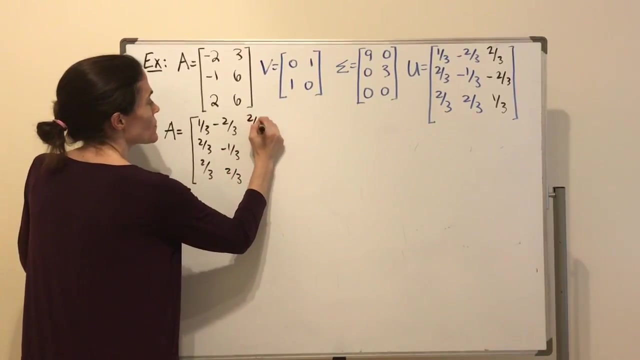 even though we have all the matrices on the board, We'll write it out now: 1 3rd, 2 3rds, 2 3rds minus 2 3rds minus 1 3rd, 2 3rds, 2 3rds minus 2 3rds and 1: 3rd. 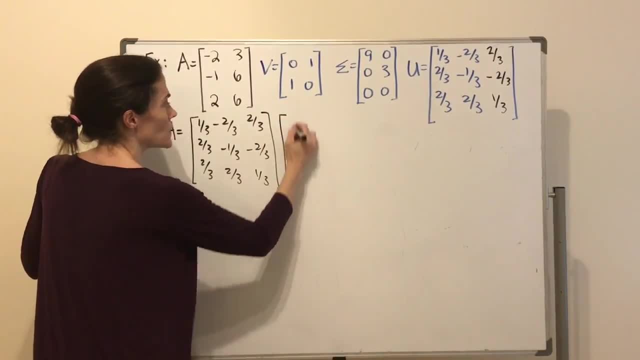 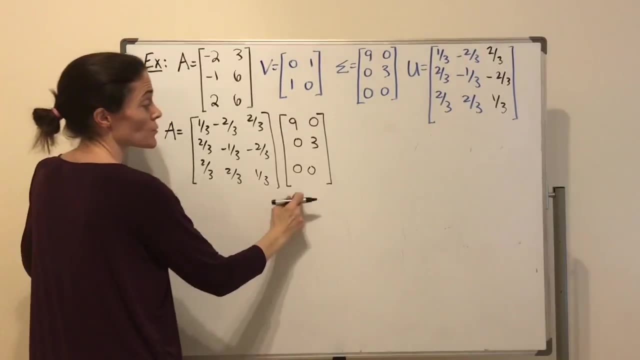 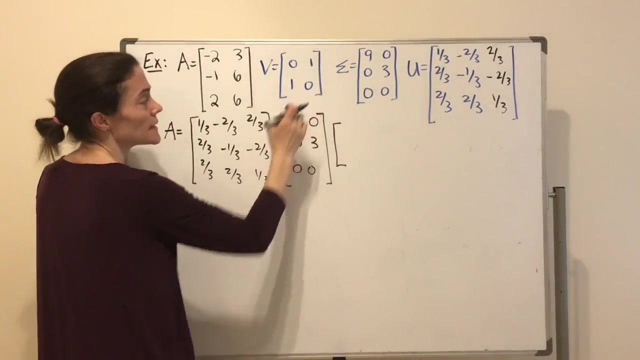 And then sigma 9 0 0, 3 0, 0,, 3 by 3,, 3 by 2, the product makes sense. And then, while we take V transpose, but again, V transpose is V, so we get this. 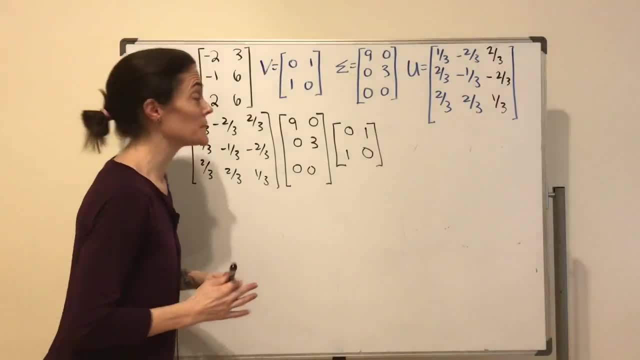 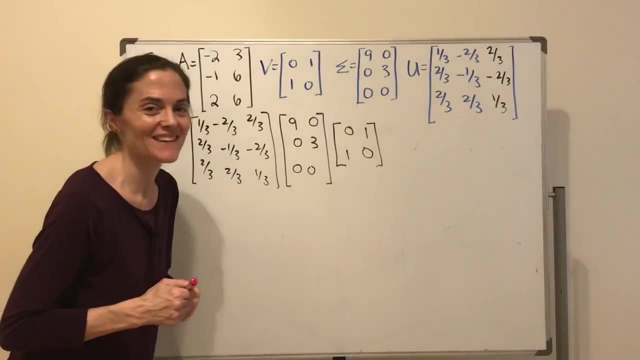 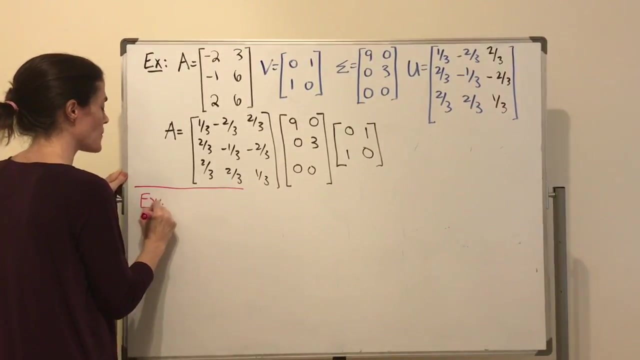 Okay, this is the singular value decomposition And you can check if you want to multiply. you will get back A. Now, immediately before I pause, before I erase anything, let's do another example And, believe me, I can fit it on the board. 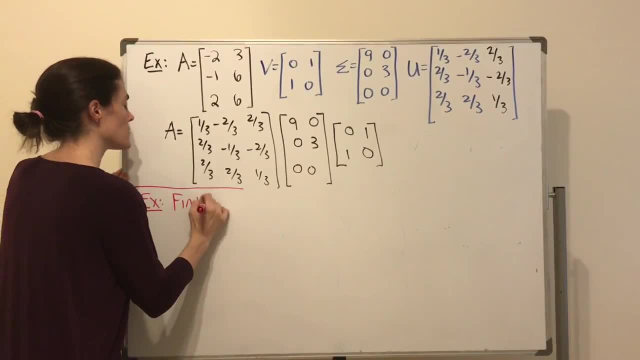 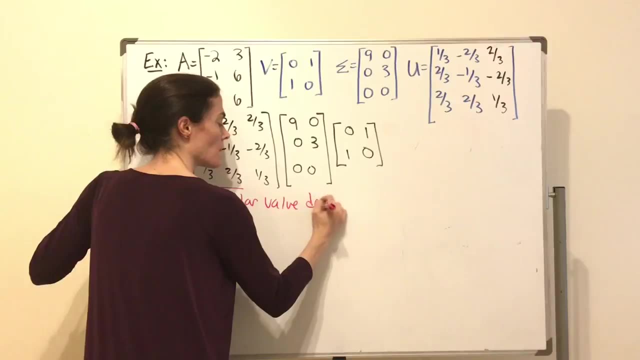 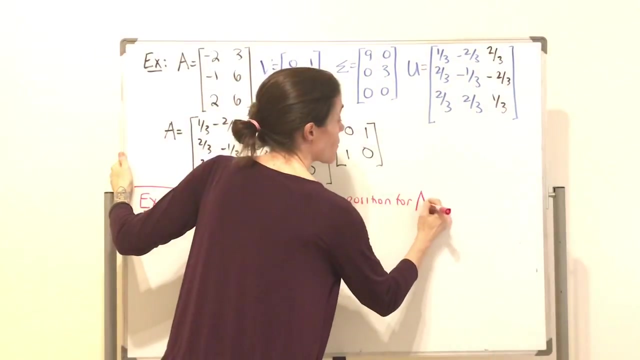 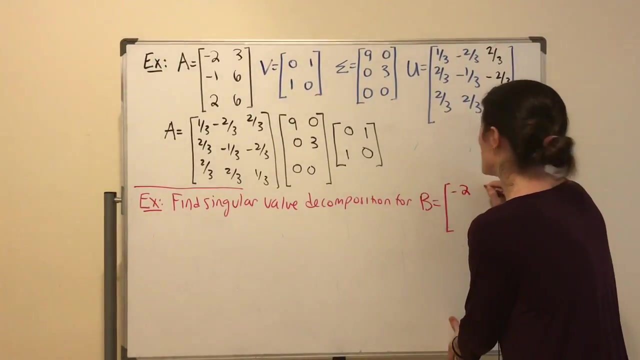 What if we want to find the singular value decomposition for the following matrix: Oh, I won't call it A, I'll call it B. Okay here, minus 2, 1, minus 1, 2, 3, 6, 6.. 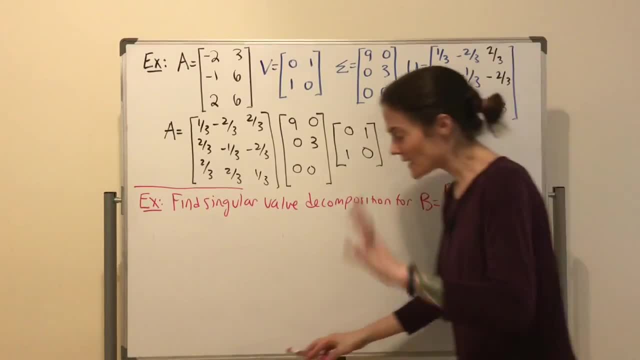 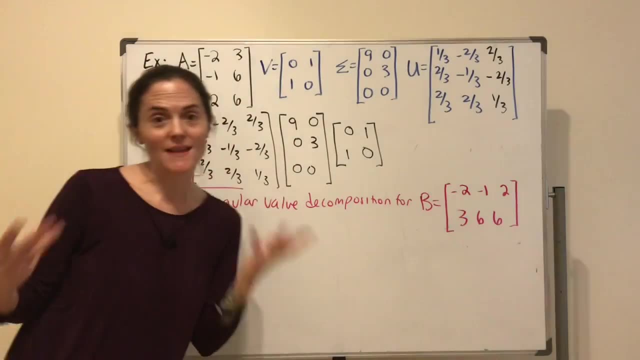 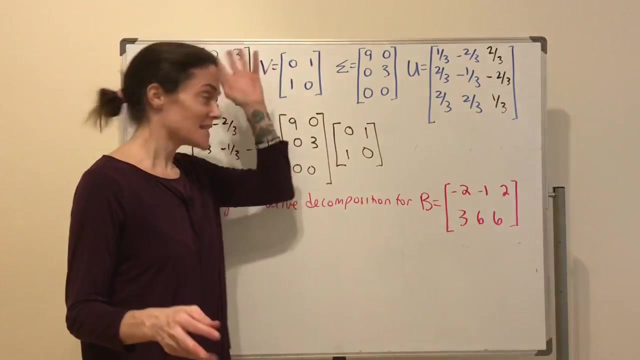 What am I going to do? Well, if I hadn't done what's above, I would start. I would take B transpose B. This would be 3 by 3. And then I would have sigma. I would have some work, because B transpose B will not be the identity, as we have seen. 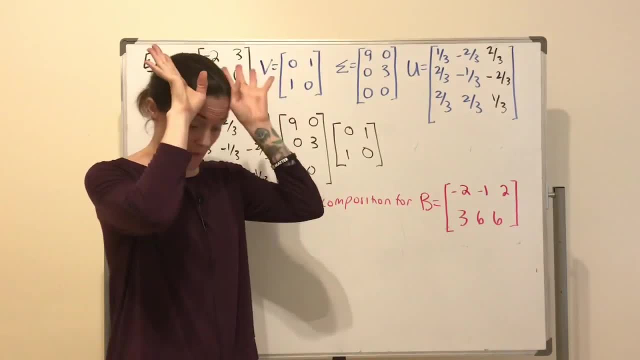 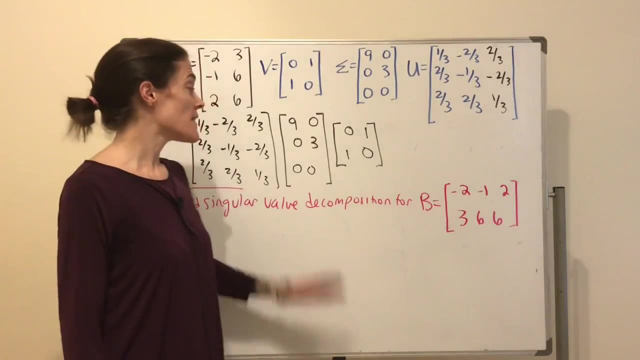 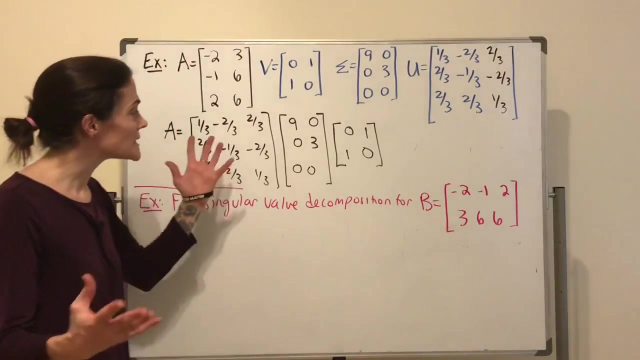 in these shorter examples I should say: find eigenvalues, find eigenvectors for B, transpose B And then the process that we have just discussed. there is no way, if I did it like that I would fit it here, unless unless I wrote really small. 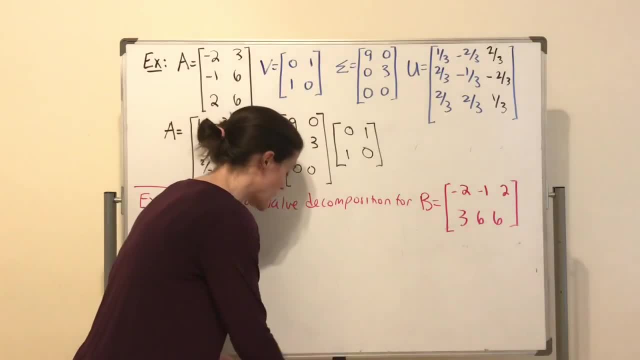 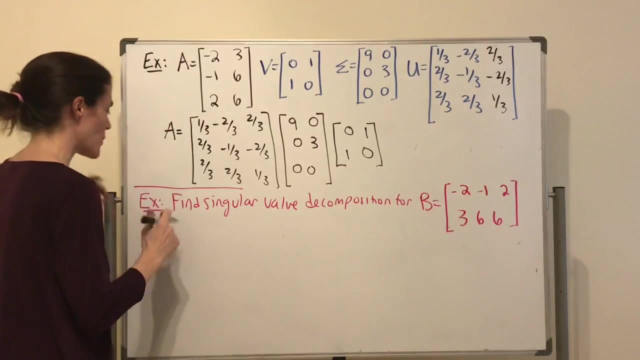 But look, B is A transpose. Okay, For this A. that's why I didn't want to call it A on this example. B is A transpose. So because I already have this singular value, decomposition, this is orthogonal, Orthogonal. 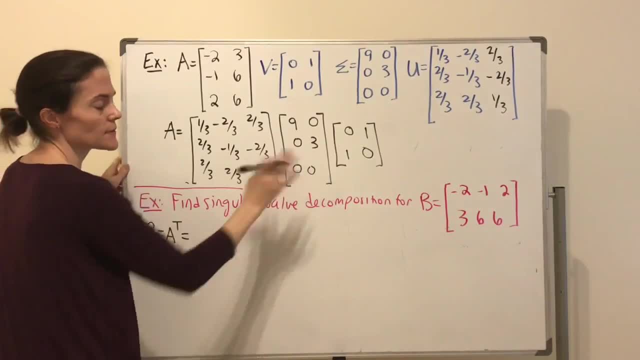 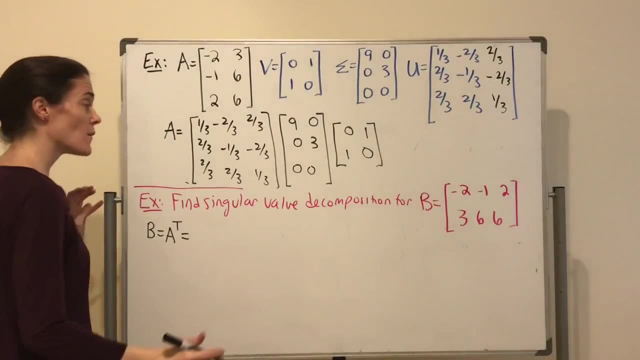 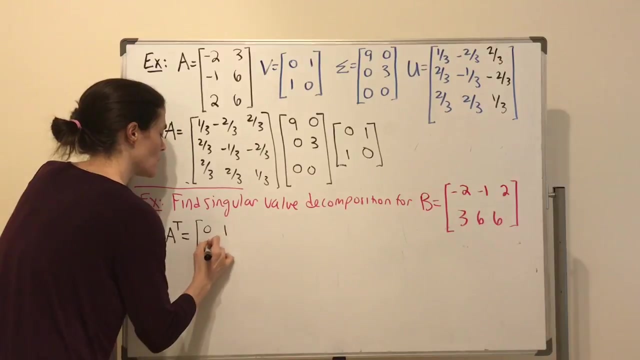 Okay, And this is this, this sigma matrix, If I take phew transpose. well, we know what goes in the other order, So this would, So I have this transpose. Uh, oh, I didn't write it right. 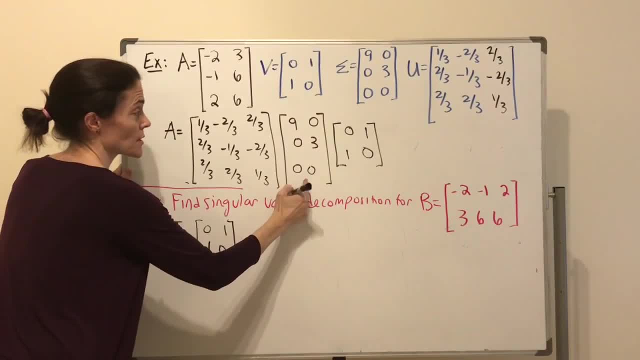 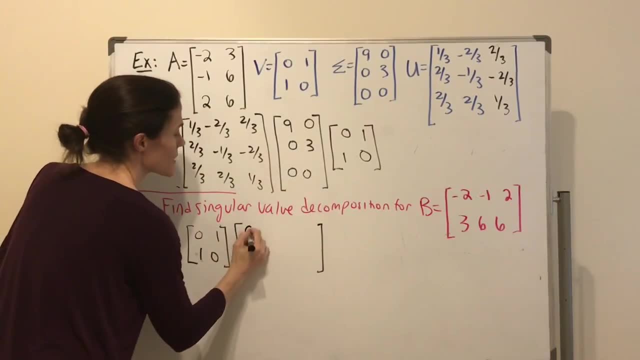 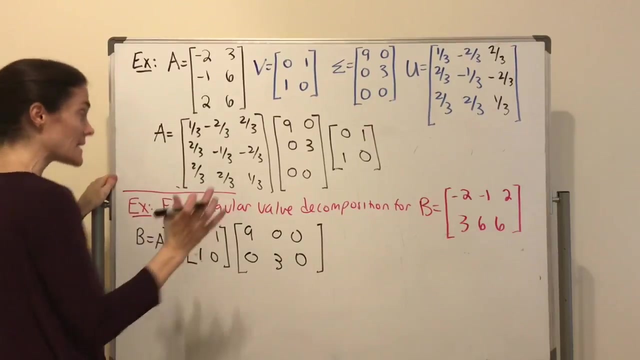 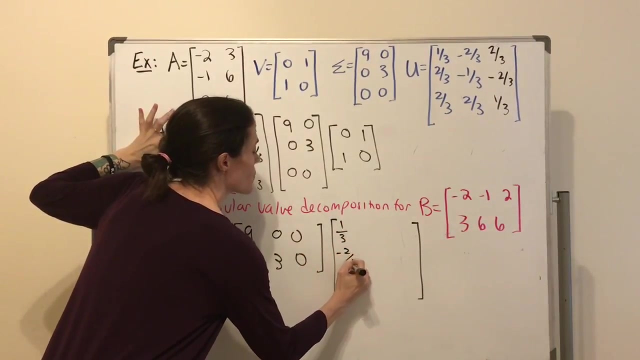 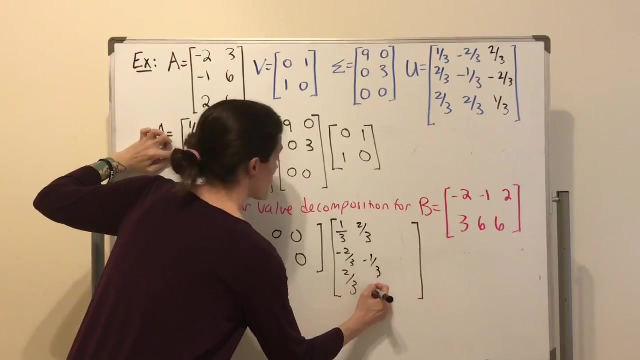 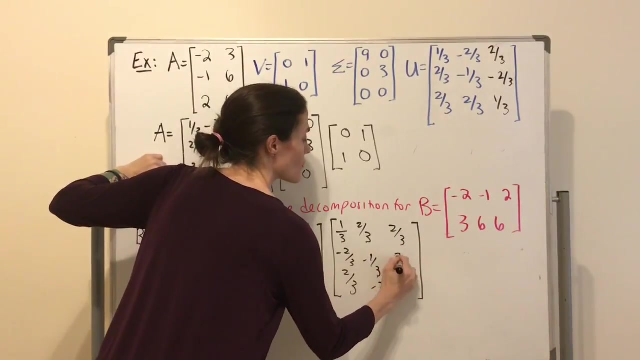 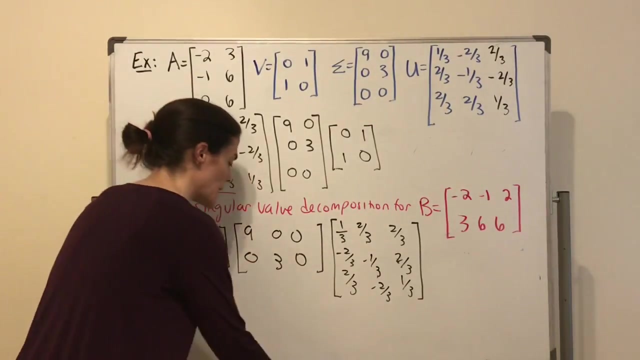 Then I take this transpose: Let's see: the first column becomes the first row, Second column becomes the second row, And then I take this transpose: Okay, well, first row, second row, third row, and this will be the singular value decomposition for B. this is its own well. 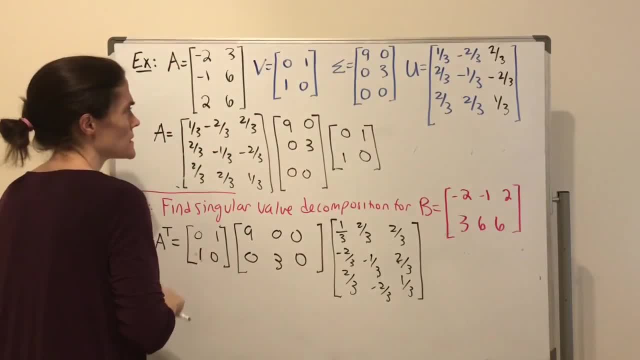 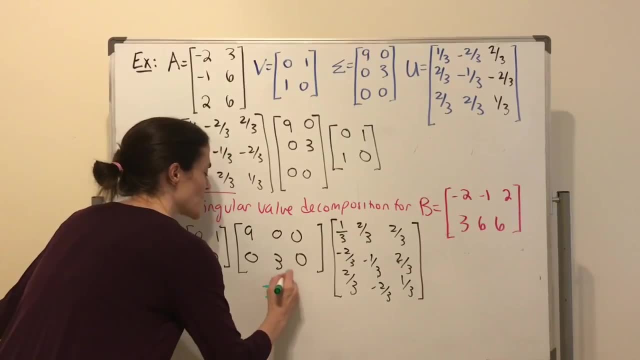 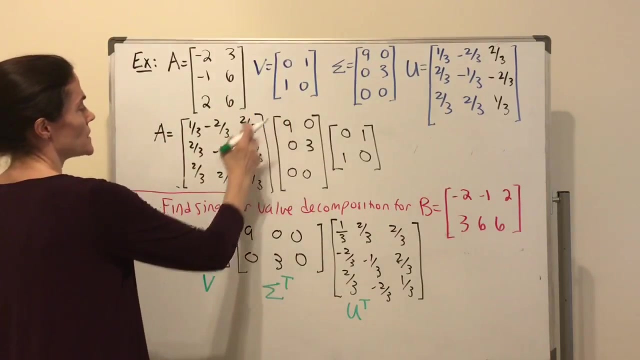 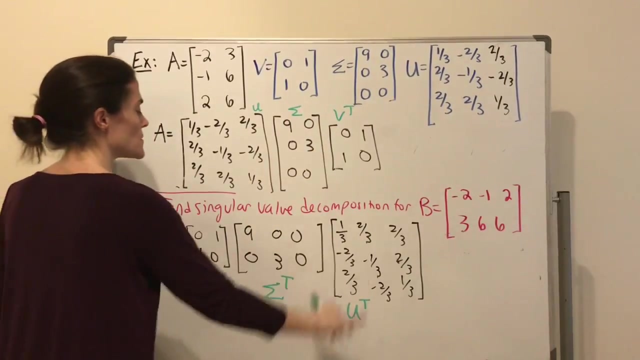 it's not the same. maybe I'll even write it like this: this is, this is V and this is Sigma transpose, and this would be U transpose like this: where, where this was U, Sigma, B transpose, like that. I just took the transpose of each one and you can also check. for example, this is 2 by 2, 2. 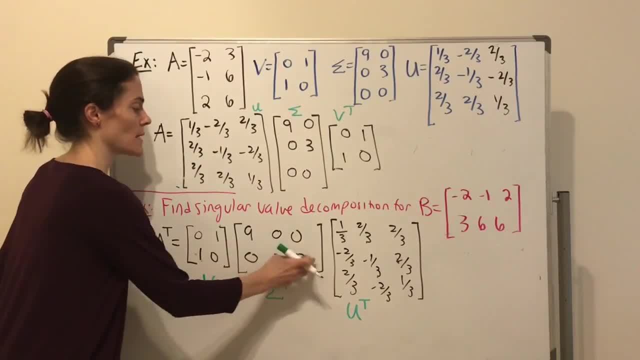 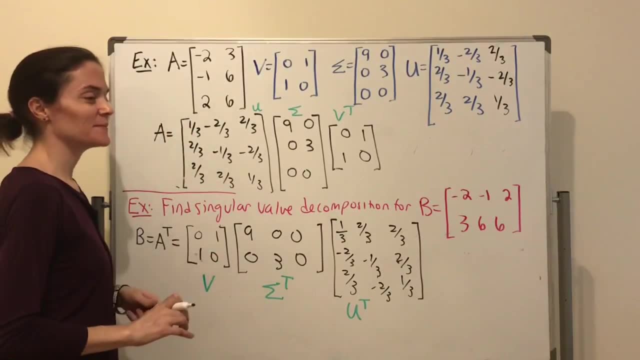 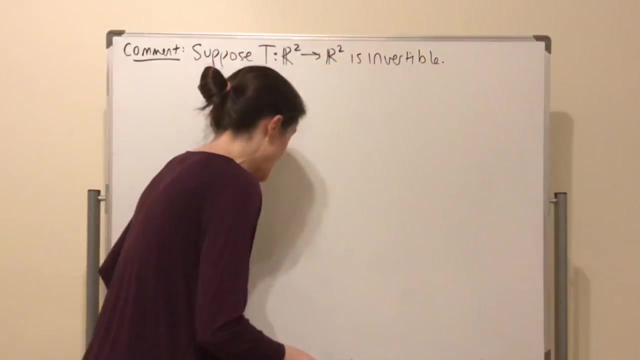 by 3 product makes sense. this is 2 by 3. 3 by 3 product makes sense and if you multiply all three you get a 2 by 3, which we have here. I want to make a comment about sort of geometrically thinking. let's suppose we have T from R. 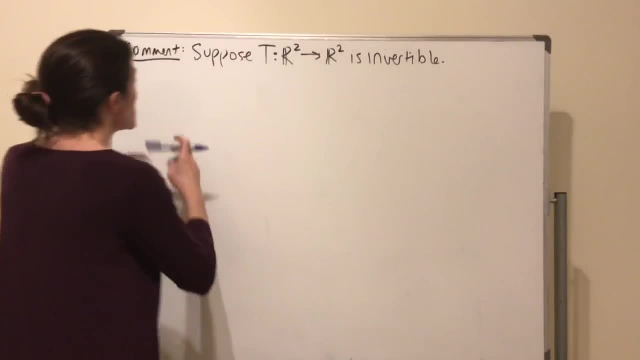 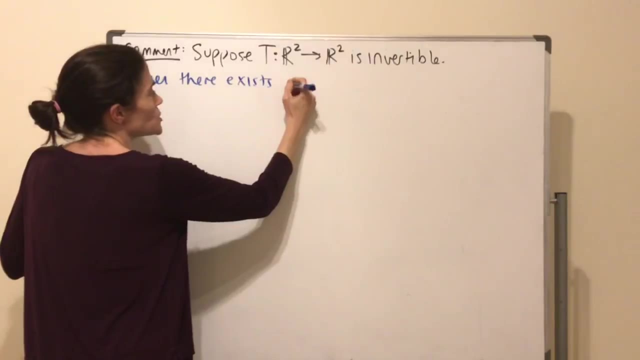 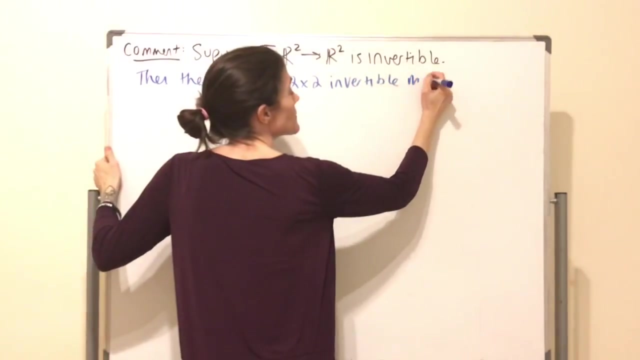 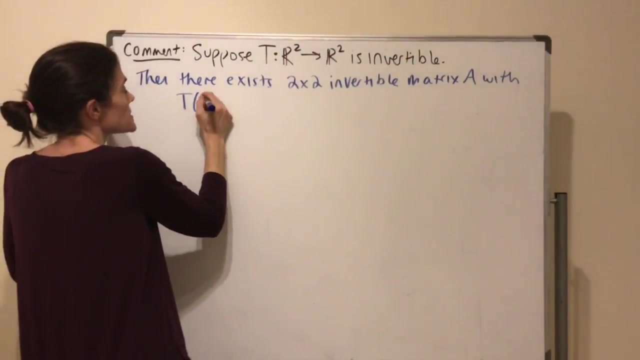 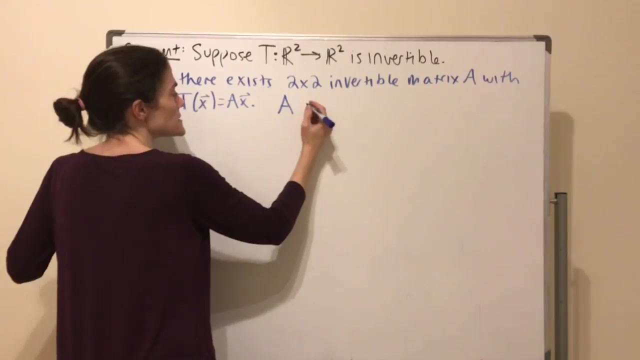 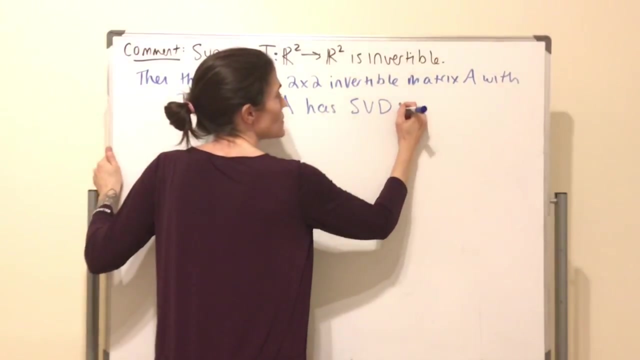 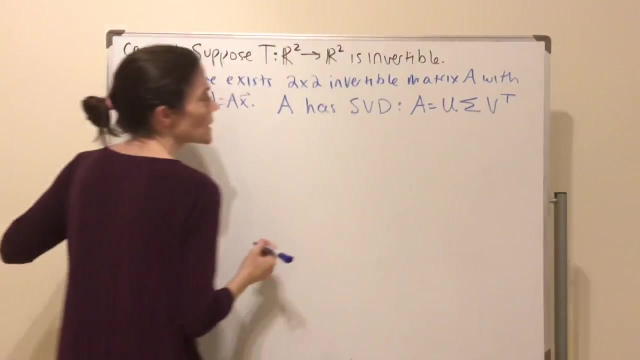 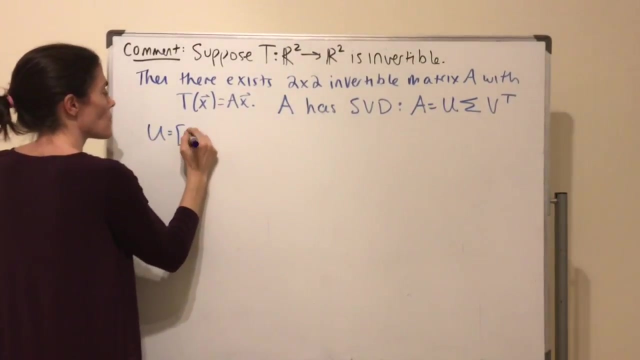 to R 2 and it's invertible. well then, there exists 2 by 2 invertible matrix. a with T of X is a times X. okay, now a has singular value. decomposition. that looks like: a is u, Sigma, V, transpose and um. let's write some things. the rank of a is 2, which means an. 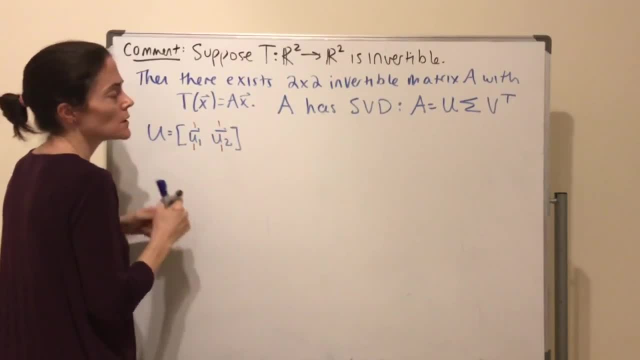 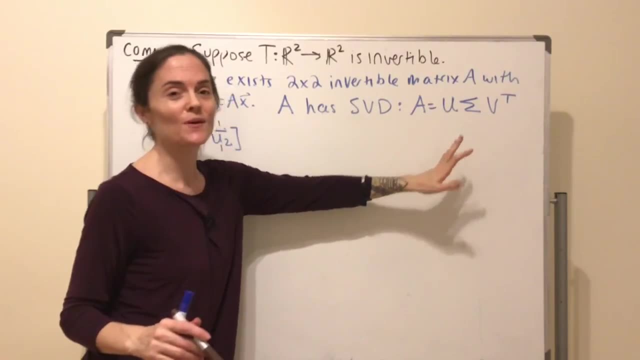 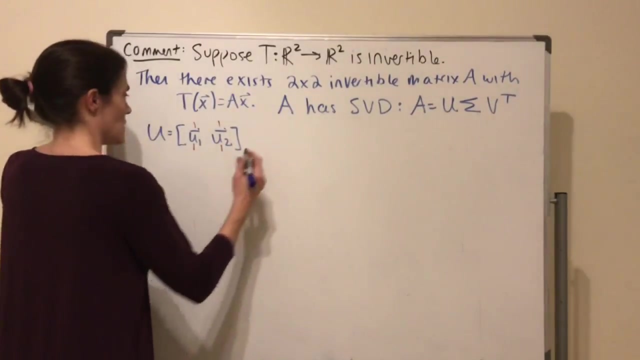 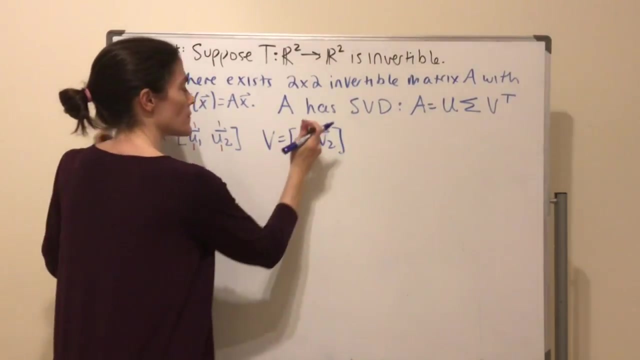 you will have two non-zero things in sigma. Well, it's only two by two, So sigma is going to be invertible. Sigma one, sigma two: the two singular values of A are both non-zero, And I'll write that. 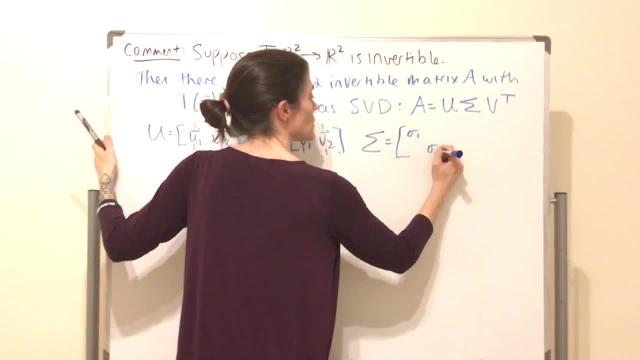 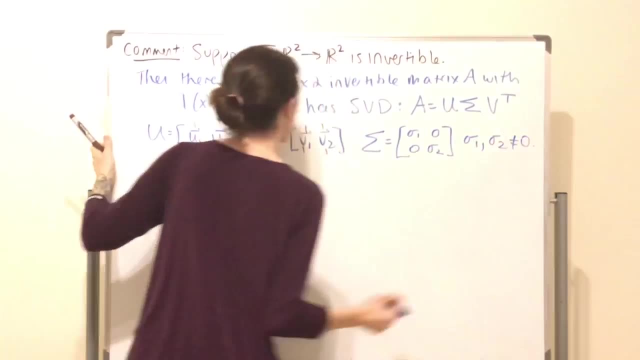 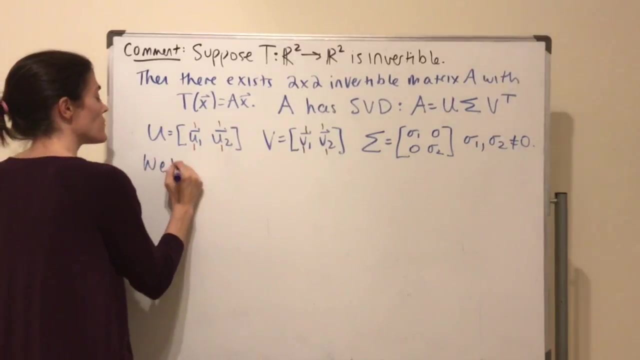 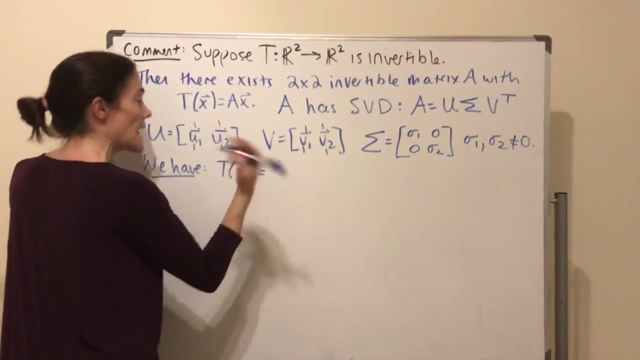 So where sigma one, sigma two, not equal to zero. Okay, Well, remember this: A V is U sigma. So we have here this T of V one is A, V, one which is sigma one, V one, U one. excuse me, 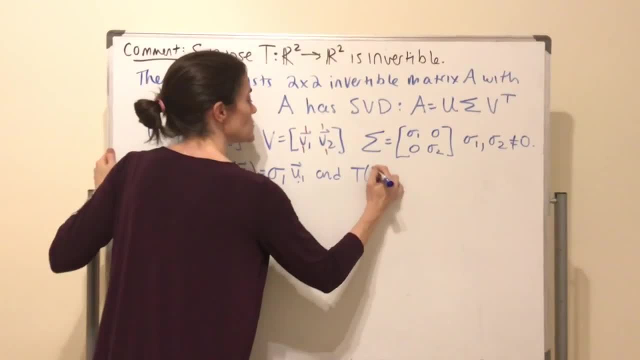 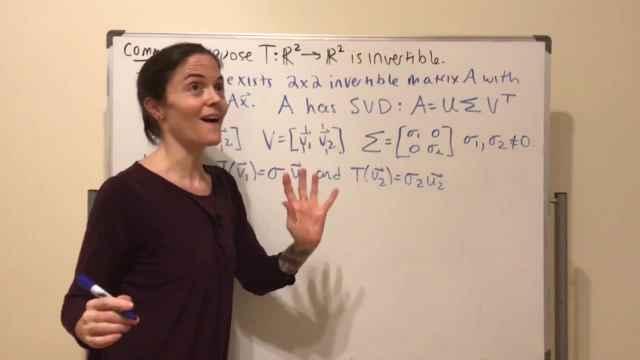 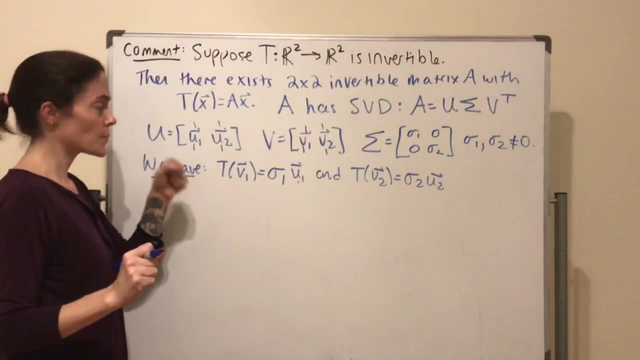 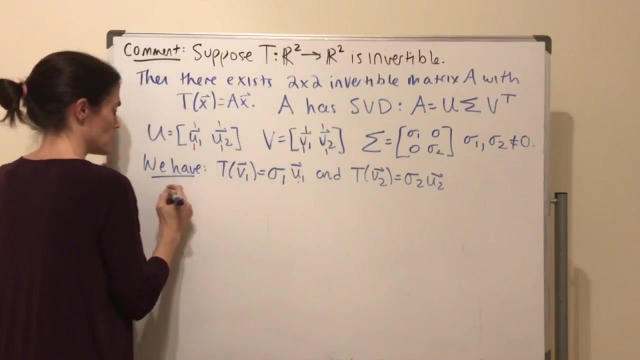 And T of V two is sigma two, U two, where U one and U two are perpendicular. So what we see here is that T of these two vectors are perpendicular, but they're no longer unit here. This has length. I'll say this. 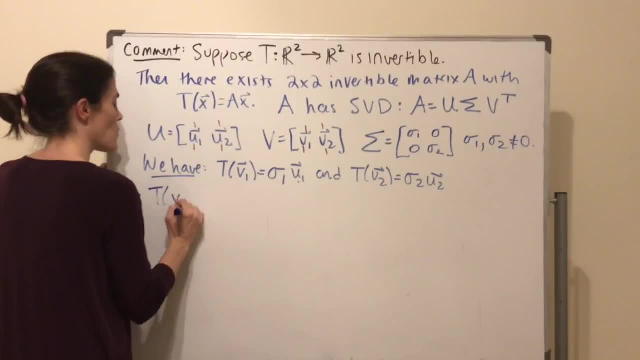 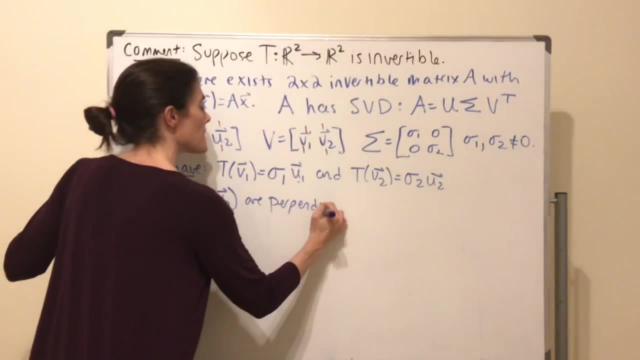 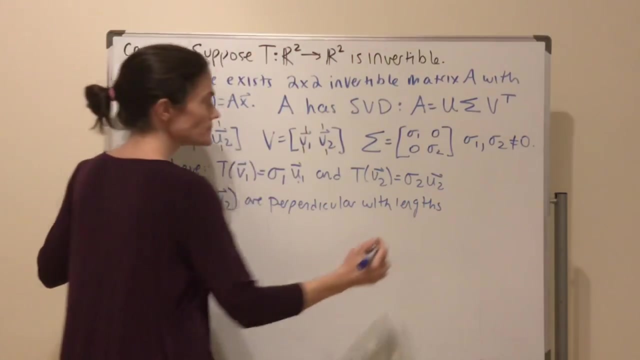 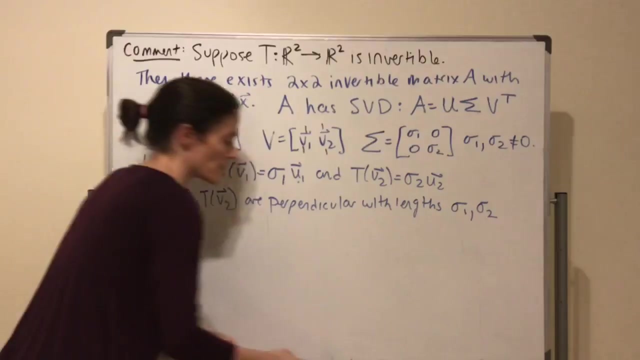 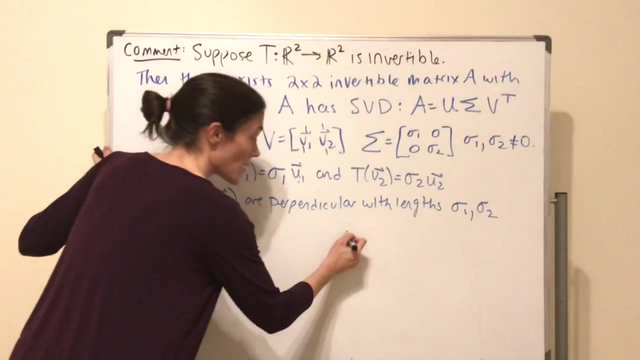 So T of V one, T of V two are perpendicular with length in sigma two. Now, what's happening geometrically? This is the cool thing that I will just mention. Okay, So here we are R two, And here we are R two. 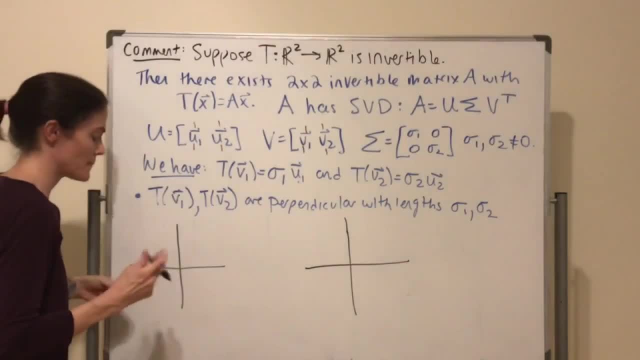 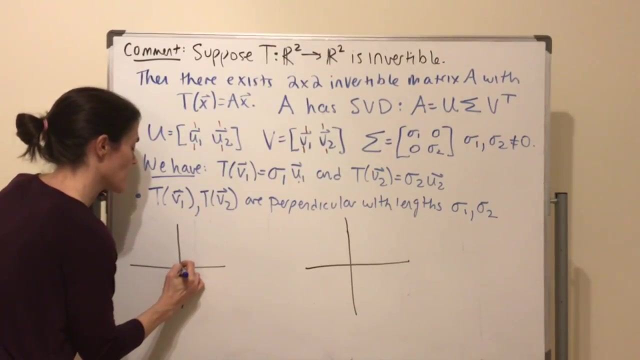 This is when I'm gonna attempt to draw. Well, I'm thinking about this as the domain Over here is the co-domain, So I have some- okay, not necessarily the standard- vectors. I have some vector here and some vector here. 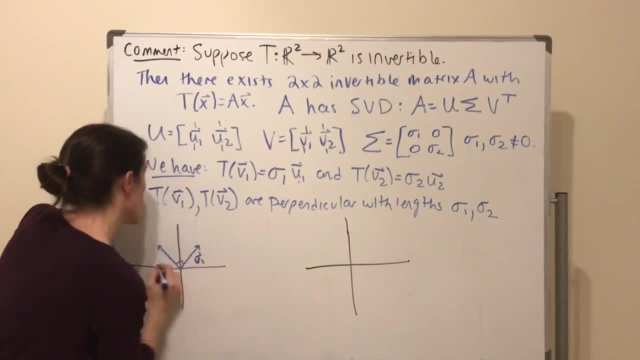 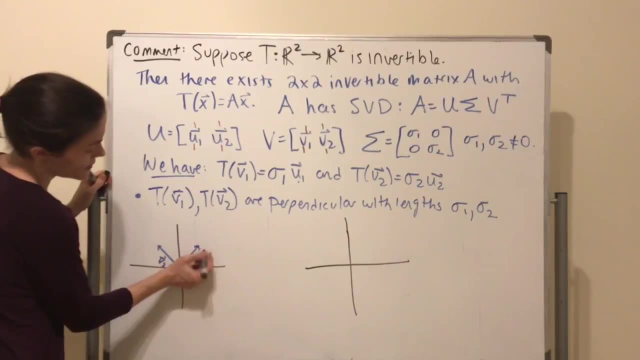 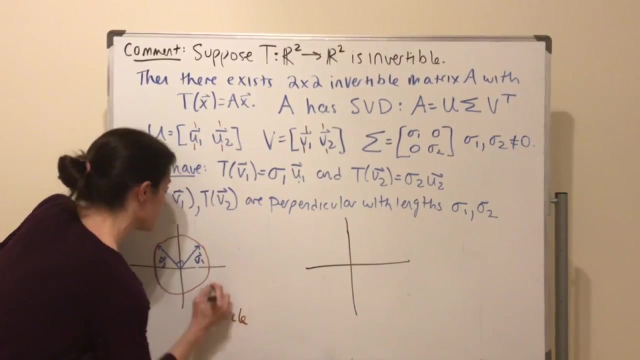 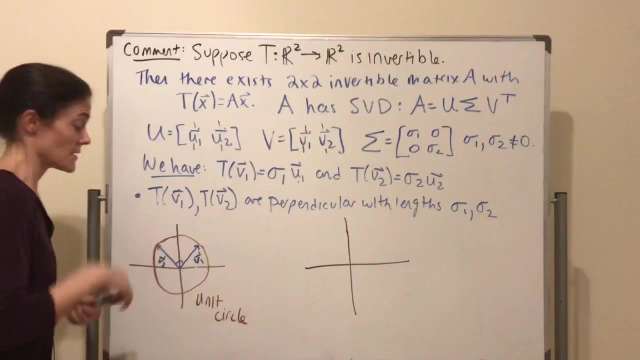 Perpendicular. this would be my supposed V one and V two. These are unit vectors And if I sort of look at what goes around here, this is the unit circle. Okay, It's everything that is distance one from the origin. Now the question is, or the comment is, what happens under the map? 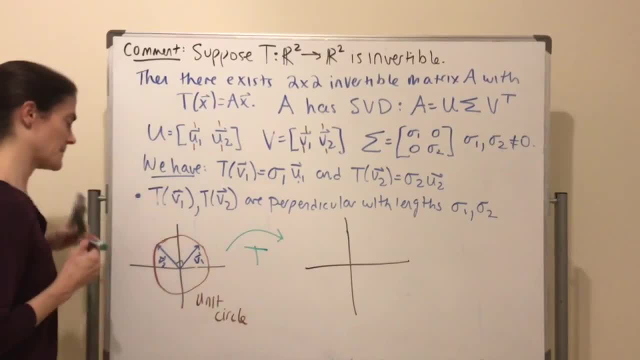 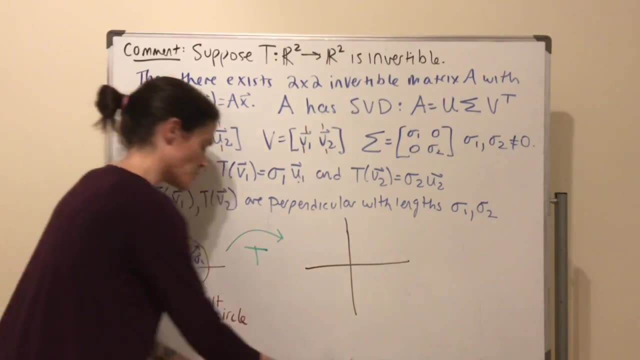 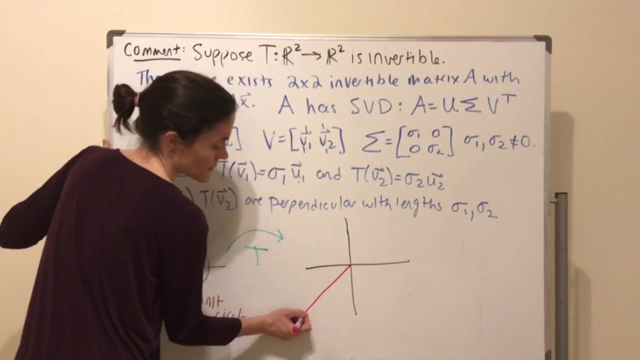 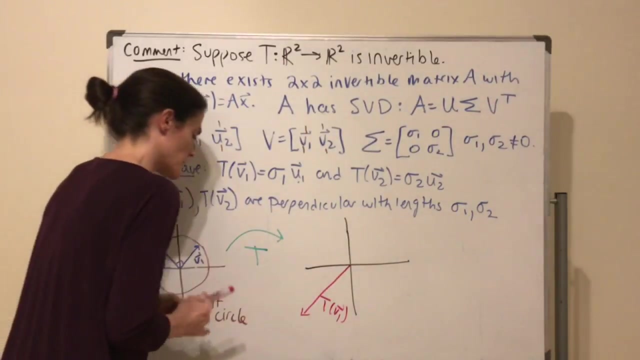 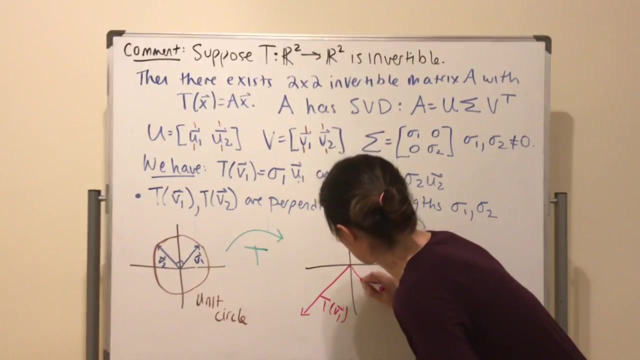 T. Well, these two vectors map to two vectors that are perpendicular, but they're not unit. Okay, So maybe T of V one maps here, And now I need to be perpendicular. Okay, Maybe T of V two Is here. 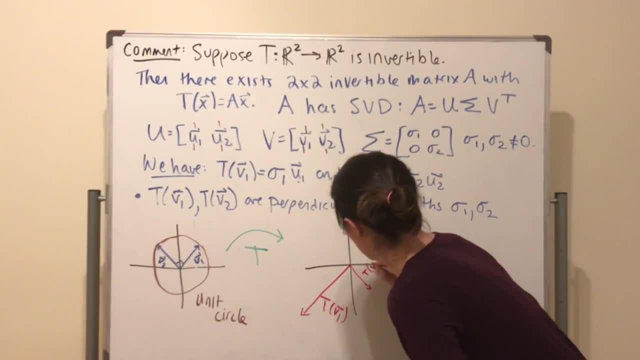 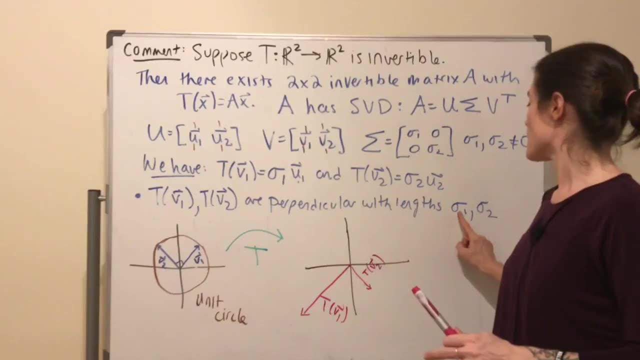 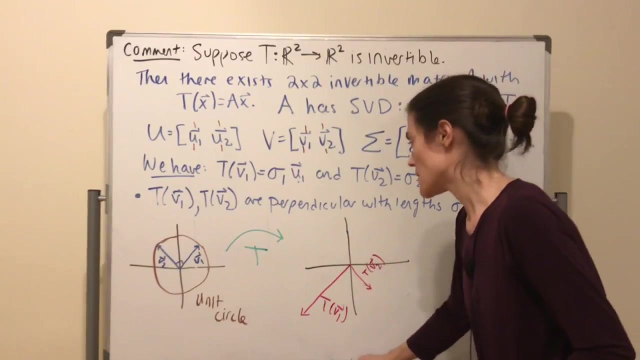 T of V two, And I know T of V one will be at least as long as T of V two, because the way we write them, that Sigma one is bigger than or equal to Sigma two. Okay, Well, what is the image here?